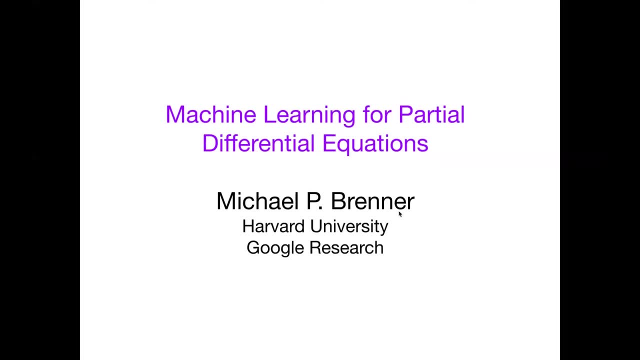 for accepting our invitation and I look forward to your seminar, Michael Brenner. Thank you, Tom, and thank you all for coming and for having me, So I should apologize in advance. I'm really bad at listening to directions and I only just realized in the last 20 minutes that this was a 30-minute talk, followed by 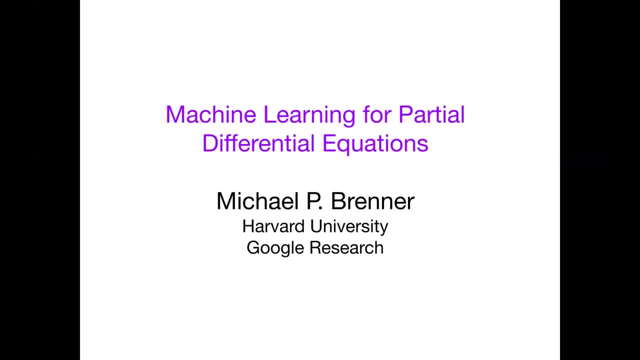 30 minutes of questions, So there are many more slides than this. So what I'm going to do- and I hope this is okay- is I'm going to set up the problem and then skip things, assuming that the problem is set up so that I can get to the next slide. So I'm going 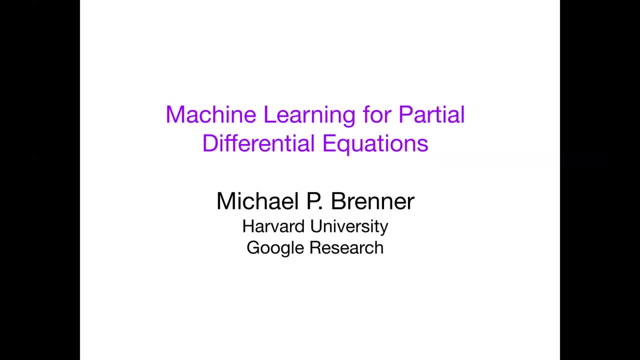 to go back to what I think will be most interesting to this group, which is at the end, and hopefully it won't appear too chaotic And if I don't get through it, I don't get through it. But anyway, I just want to apologize in advance. So the work I'm going to tell you about was 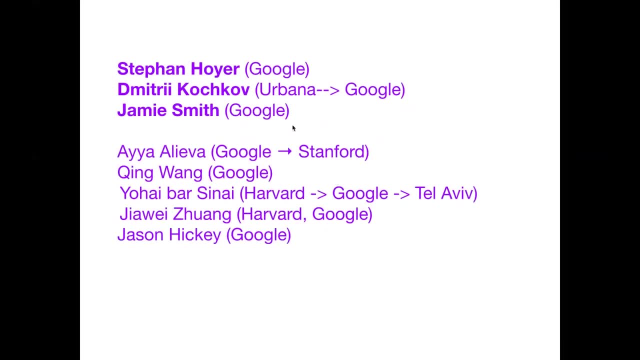 done by the group of people that I want to acknowledge first. So there's a group at Google- Stefan Hoyer, Dmitry Koshkov and Jamie Smith- who worked on the Navier-Stokes machine learning for Navier-Stokes part, which is the second part of the talk which I think is going to 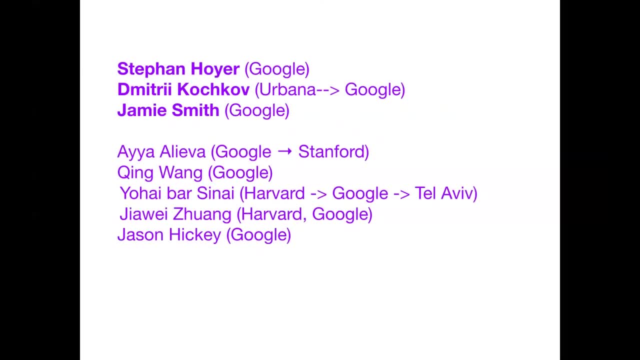 be the second part of the talk, which I think is going to be the second part of the talk The most interesting to this group, along with a larger group of people. So Yochai was a postdoc at Harvard when we started this work with Stefan and Jason, Anyway, so I will. 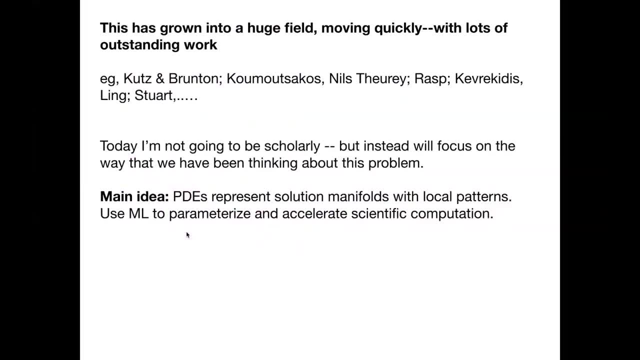 just jump into this And I guess I want to say the subject of machine learning, just as apologies for scholarship. So the subject of machine learning for PDEs is a large field that is rapidly growing and there's tons of outstanding work that's going on And I 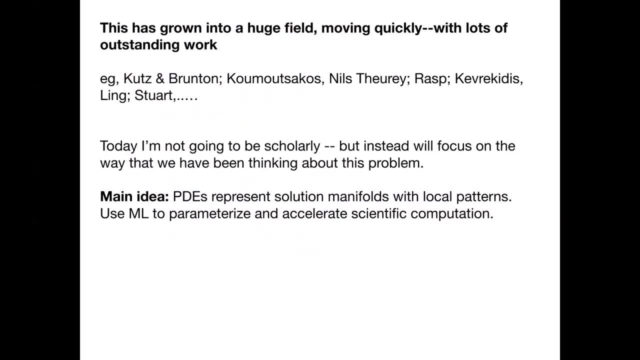 sort of you know. I'm going to start with the first part of the talk, which is the work of the school and the work of the faculty, And I've been working on this for a long time and I kind of like to say that I really like it when people are scholarly in their presentations. 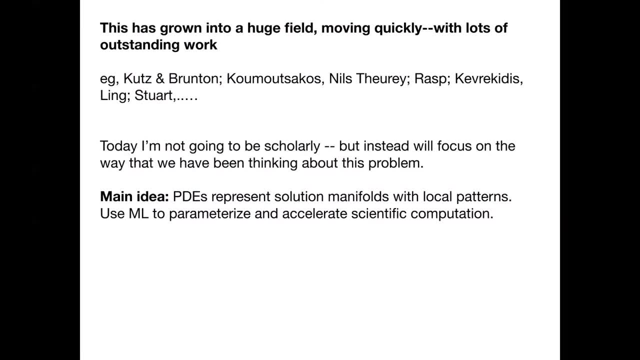 and I'm not going to. I just want to apologize in advance that I'm not going to be scholarly here today. Instead, what I want to just get through is the way that we've been thinking about this problem and what we've been doing with the hope of stimulating conversations. 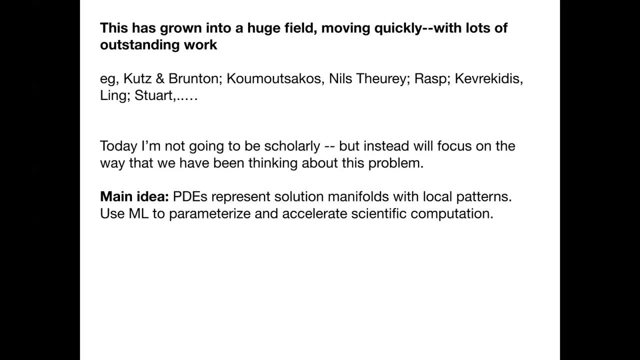 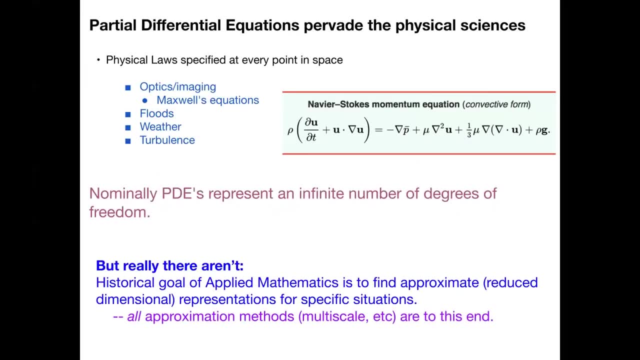 But I just want to make it clear that there's a really big and exciting field out there that I'm just not paying proper homage to. Okay, so this is the part where I go fast. So we tell students that PDEs. when we teach PDEs to students, we tell them that a PDE 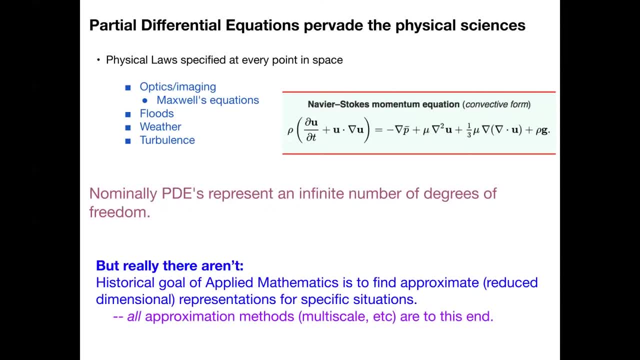 represents an infinite number of degrees of freedom and that, indeed, when we solve them numerically, you know, as in climate and weather, for example, within this context you know there are an infinite number of degrees of freedom, which means that we, we basically resolve them by using large numbers of mesh points to to resolve every possible scale. 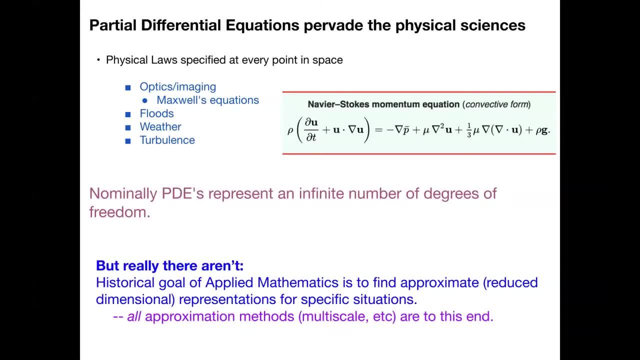 But but we really know that in a particular situation this isn't the case, that the solution manifold has a finite dimension, And in fact I would argue that you know, historically, the goal of applied mathematics as a subject has been precisely to find approximate representations of the solution manifold in specific situations to make them useful for computing. 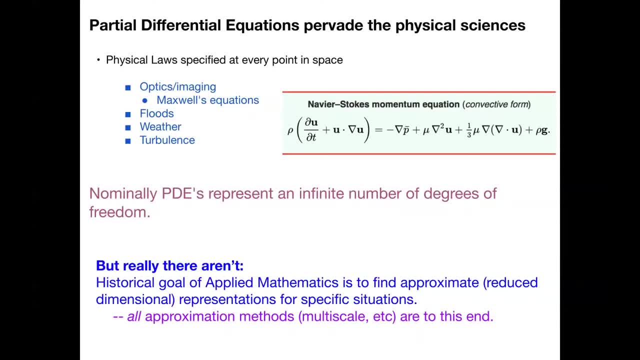 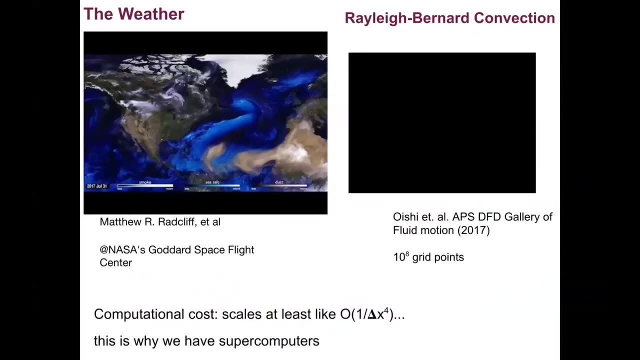 And this is, you know, there's a you know a century of approximation methods, that sort of go after this, But yet when we actually compute things, you know, you know, in the computer We really haven't figured out, and I think that this is a fair comment- you know how to take advantage of this and this you know: movies of the weather, there are movies of things, and that, basically, you know, things are computationally expensive. 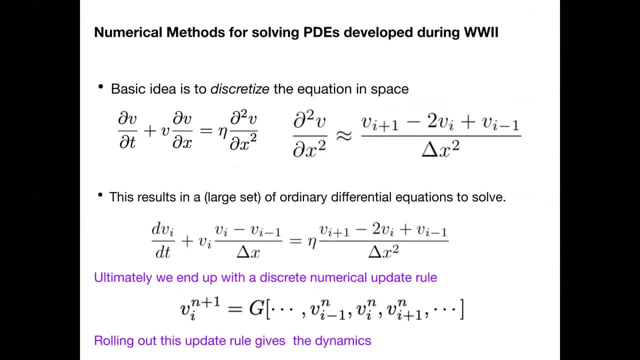 So the way that we develop numerical methods, of course, is by taking an equation- and here's burgers equation, which I will use as a simple example in a little while- and we of course you know 1, you have to break it up into a bunch of discrete, into a bunch of variables that live on a mesh. 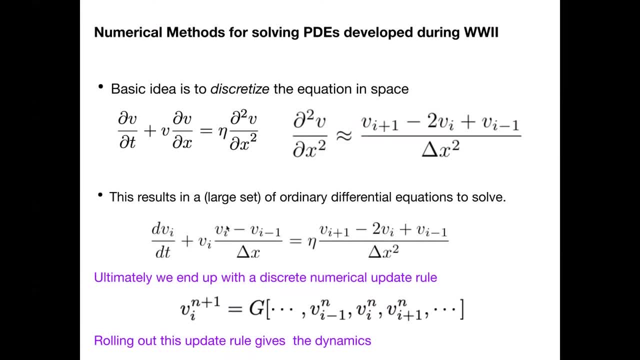 By using discrete, discrete Operators for the finance derivatives, and that reduces the into a set of, and then, ultimately, we end up with this set of discrete numerical update rules that we teach students and that we indeed drive ourselves. How 1 starts with the original equation and through whatever hook or crook numerical method you want, get a numerical update rule to update the solution at every time step, and then we simply just roll this out, and that's, that's the way that numerical methods works. 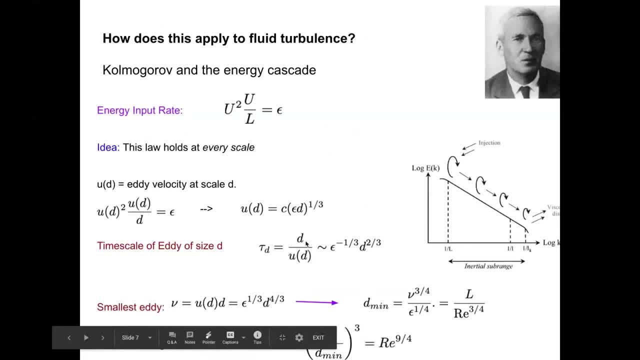 And so this I'm not. I'm going to skip the slide in the interest of maintaining my 30 minute thing, But What I meant to say was that you know, if you think about fluid turbulence, then this presents an impossible conundrum because, of course, the range of scales is very large and you know, taught us what the ratio is of the largest scale to the smallest scale through the scale and freedom. 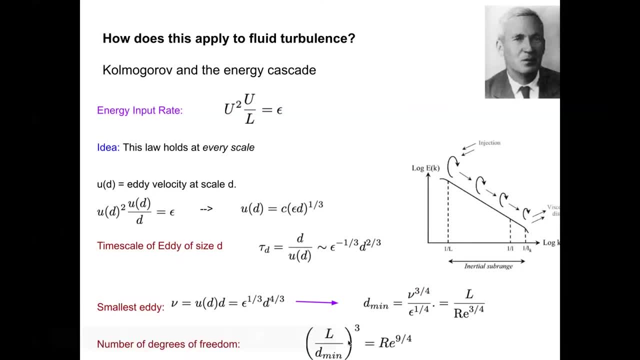 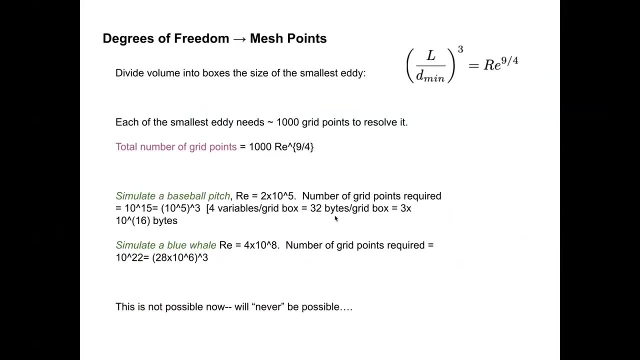 Just the number of eddies that can fit in a box scales like a huge power of Reynolds number, like the Reynolds number to the 9, 4th power, And you know, if you basically choose To use- I don't know- 10 points per or whatever, you end up with a number of grid points that are required to resolve the direct numerical simulation which is. it was impossible 50 years ago, It's impossible today. 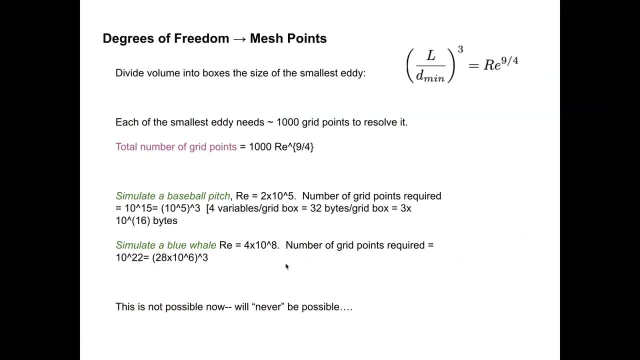 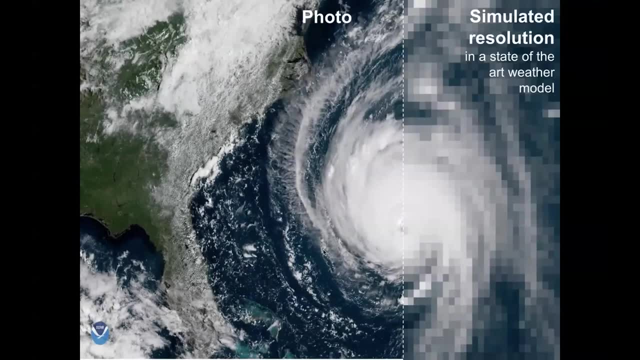 And we'll basically always be impossible. And the question that we really face as a community is: how do we get around that and do more accurate Simulations, you know, for example, of climate and weather, where computational grid boxes tend to be much larger than the degrees of freedom which are certain? 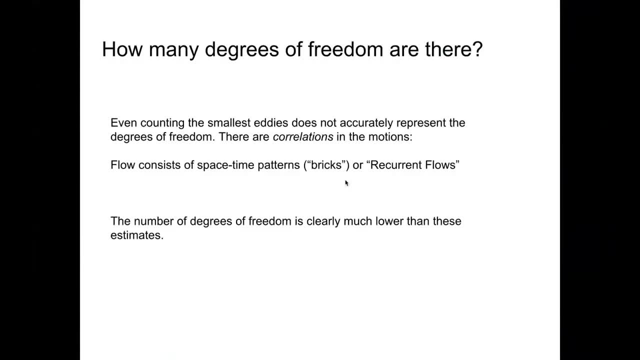 And of course, there's a long intellectual history of this subject. I'm here, I'm going to skip this point At this point. this slide makes the point that you know, even the individual, even this estimate, right. 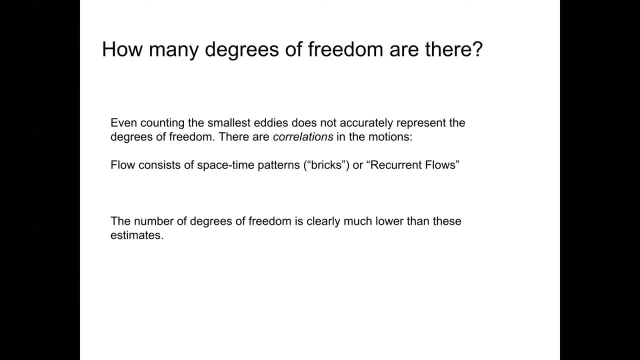 You know, if county is a massive overestimate of the real number of degrees of freedom in the system, because there are correlations between the eddies and you know 1 really needs to take into those, This is sort of a huge problem for our community. It's been a huge problem for our community for a long time. 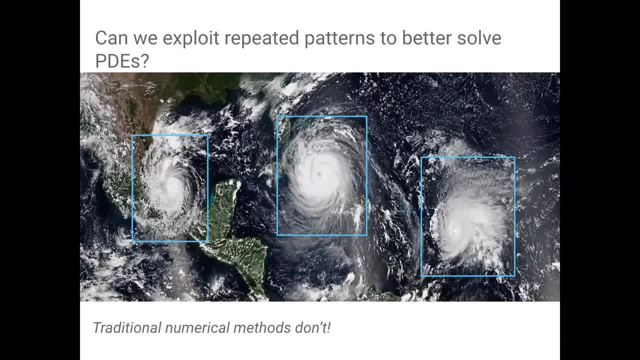 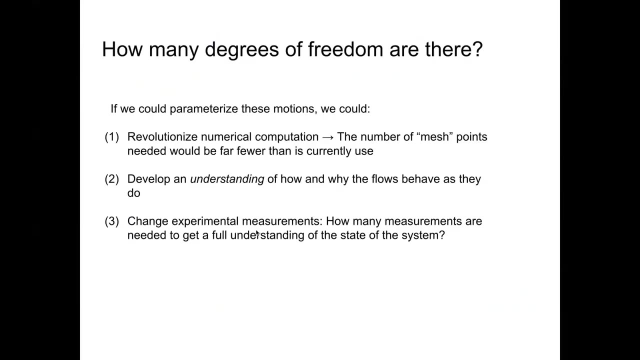 And the question that We've been interested in that I will discuss in this talk, is to what extent can we use machine learning to basically recognize repeated patterns within the solution to better solve, more efficiently solve and to better understand partial differential equations? So- and this is all based on the idea that there is a solution manifold and underlying solution manifold, If 1 could parameterize it, then you know then and compute with it, then there would be a huge cost savings. 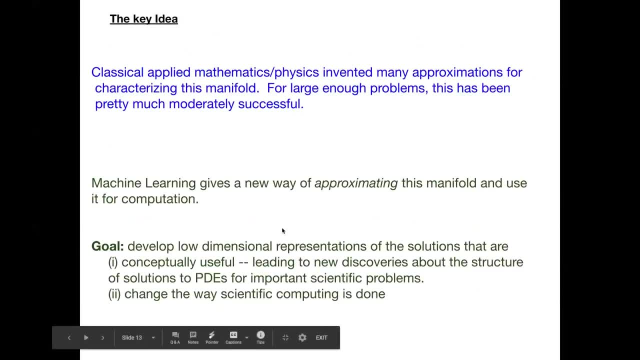 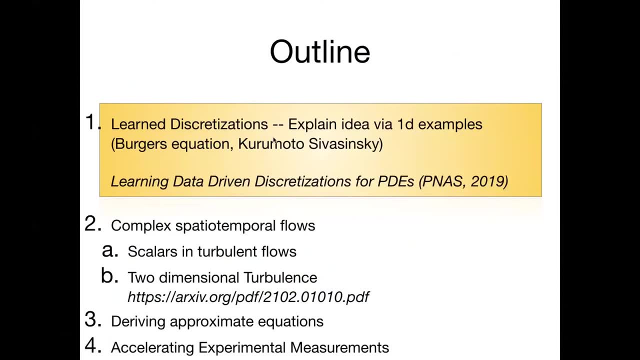 So, so okay, I've already said this part. sorry, this is the part where I'm skipping slides to catch up, So this talk has sort of. I'm going to have this talk, have 2 parts and actually I have references to papers of these parts. 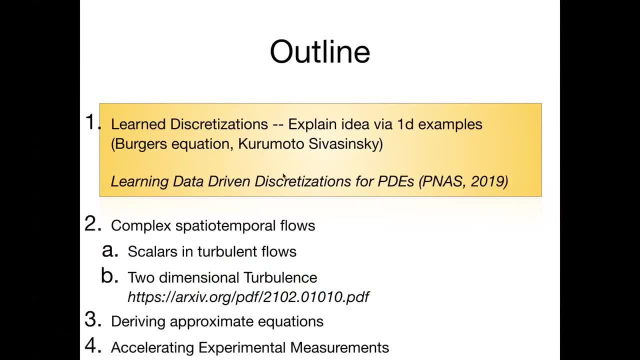 because I seem to be going quickly and just to make sure that people understand. So the 1st thing I'm going to tell you about is an idea of which we call learn discretization, that I'm going to explain via simple 1 D examples. 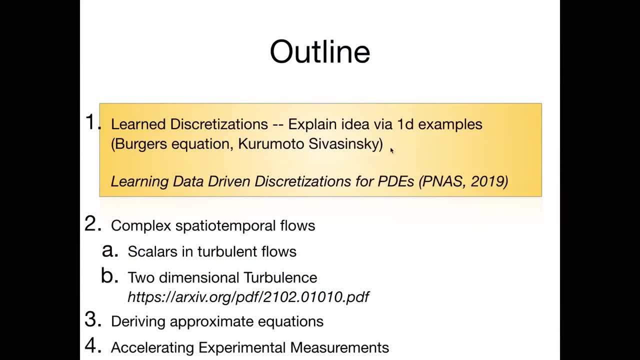 which I think what sort of makes the pedagogy, the idea clear, and this is a paper that was published in P N A S In 2019, and then what I'm going to do is I'm going to skip to a paper that we just posted to the archive last week, which is applying these ideas to 2 dimensional turbulence, and and that's what I'm going to do in this talk. 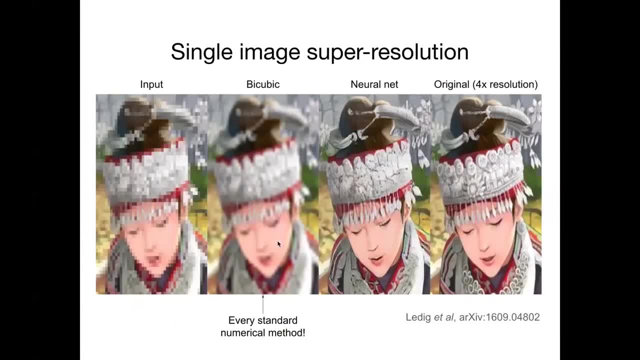 So, by the way, I know the spirit is that no 1's supposed to interrupt me, but I'm self conscious, So if you want to, then go for it, Okay. So we are inspired by what I'm about to say, by the example of single image, super resolution. 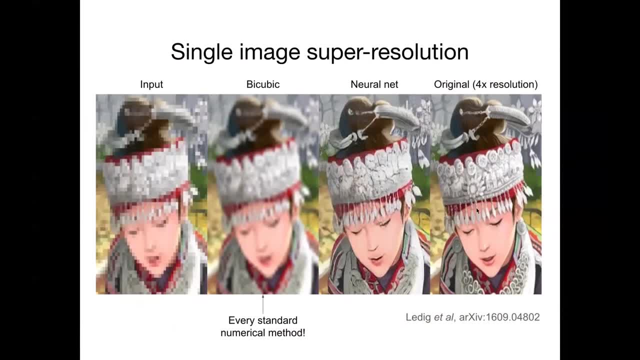 So this is a machine learning computer vision method Where 1 takes an original image at its original resolution and down samples that to be able to store it better, And then 1 is presented with the problem of how does 1 up sample the down sampled image to reconstruct the original image? 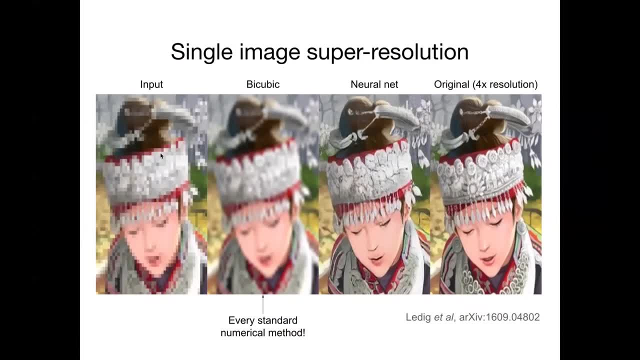 And of course the simplest way to do this is to simply use some sort of interpolation scheme on the pixels of the down sampled image. And if you do that with by cubic splines, then the image is blurred. But you know computer vision. people have discovered that by using neural networks locally. 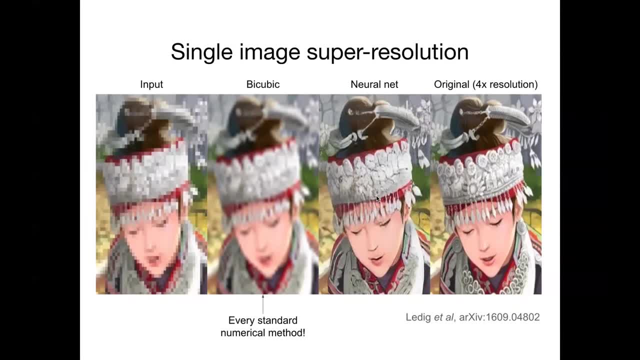 That is, are acting a little local Parts of the image 1 can can sharpen things up considerably, and these neural networks are trained on, for example, large number of consumer images. So, from the point of view of, Of numerical analysis, numerical analysis, of course, up samples with interpolation, That's what we do. 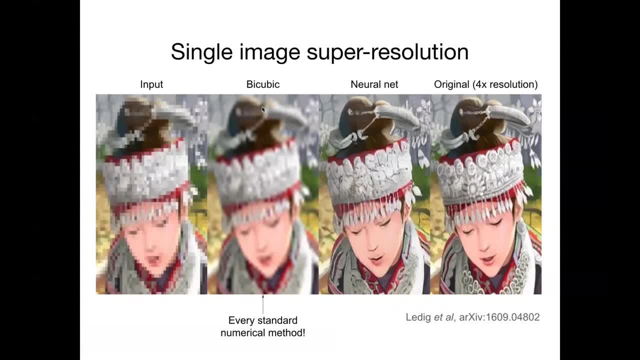 We consider some type of interpolate that we're sampling with, and we tend to use functions that are that are as general as possible so that we can represent whatever it is that might happen, And the thought was that maybe basically that what the neural network. 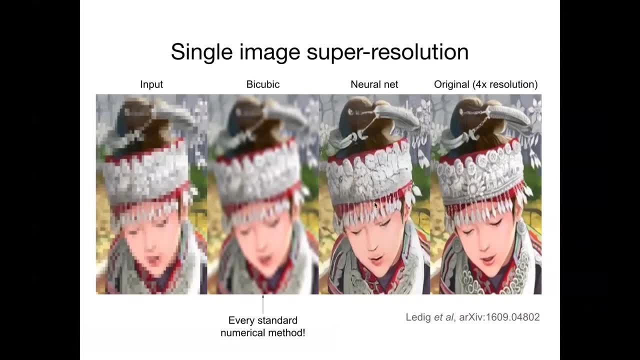 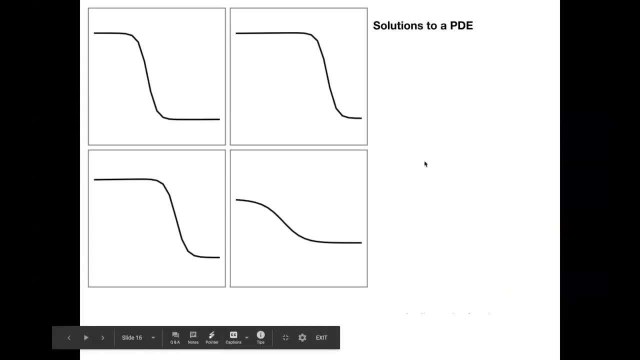 Might be doing is learning something about the underlying functions in the set of images and using those top scale, And that idea should be applicable to as well. So, just as a toy example to get you all in the mood, Imagine that that these curves are solutions to some PD, and I don't tell you what PD they are, but I want to numerically solve them. And so the way we typically go about this, of course, as we choose grid points- and I've purposefully chosen grid points to essentially under resolve the shock in this picture- 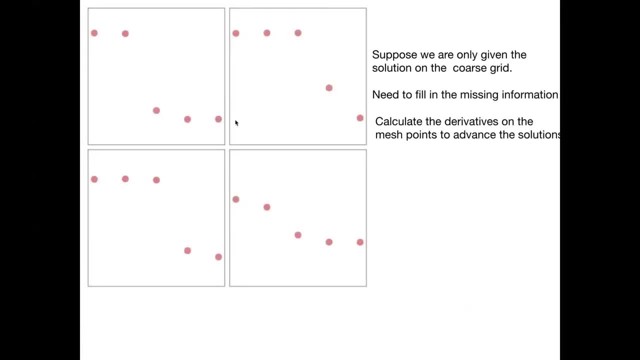 We then erase the original solution And I then give you the The Solution, and I then give you only the solution on the grid points and I ask you to please time, evolve the solution in time. So in order to do that, given the PD. the PD depends on the value of the function and its spatial derivatives. 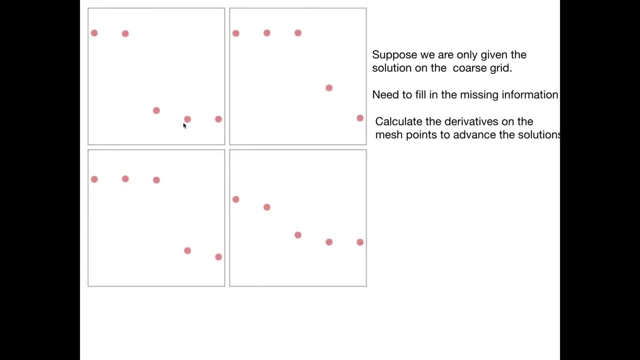 So I need to be able to estimate the spatial derivatives of each of the red points. But of course, if I do this using a polynomial interpolate, then there are well known problems that cause you to make errors when the solution is under resolved. 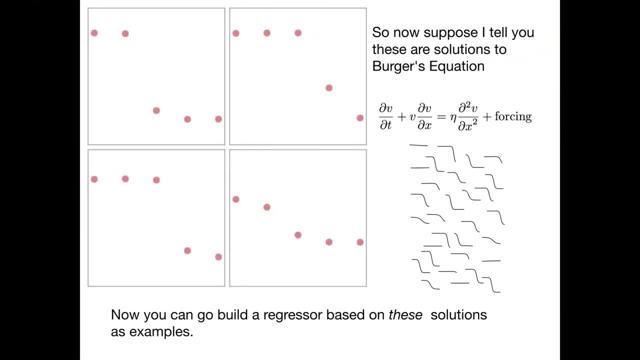 And so, on the other hand, if I told you that I actually That these dots corresponded- solutions of burgers equation, which is 1 of my favorite equations, And if you're an expert and I told you that here are lots of examples of solutions to burgers equations which I could generate with my computer beforehand, 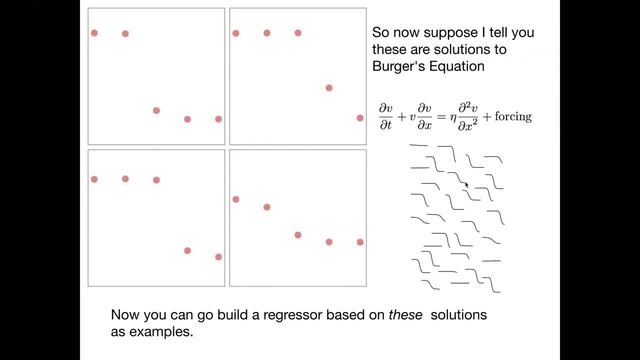 Then you know- and if you're an expert in burgers equation, then you all know that- that the polynomial interpretation that I showed can't be solutions to burgers equation. In fact, the burgers equations can only be chosen from this set. So the notion is: is that what I'm going to now do is when I build my interpolate, 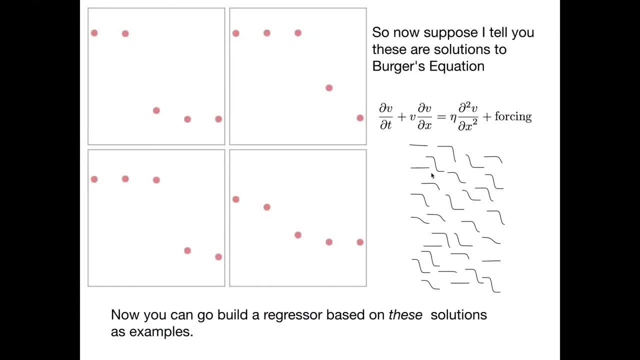 instead of using general functions, I'm going to just build a regressor based on what I know can happen, and then use those to compute derivatives, And, of course, this works much better. right, When you do this, the yellow curve works much better and lets you- and that's the basic idea- 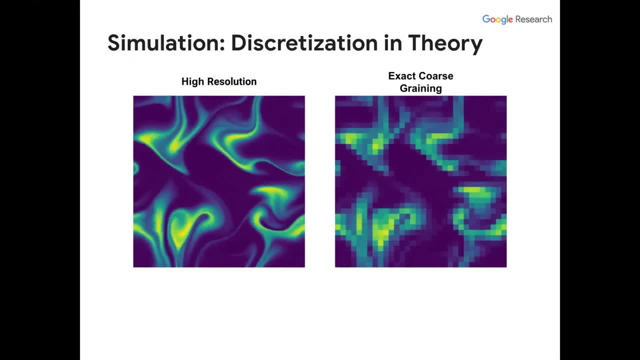 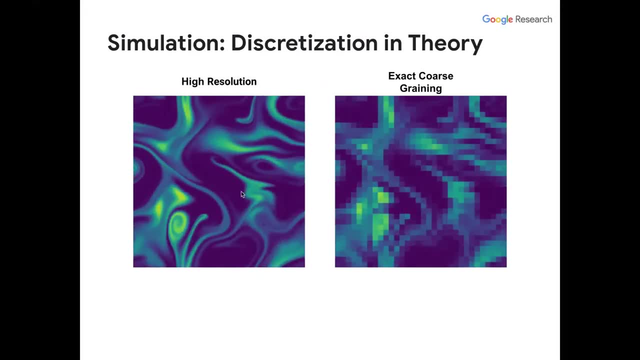 that we're going to bootstrap off of. So what we're going to be in the business of doing today is the following: I want you to imagine I have a high resolution simulation that you've acquired through some means, and then I'm going to imagine that you coarse, grain it. So this picture on the 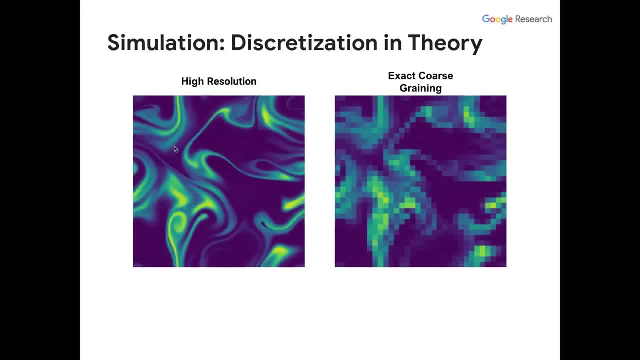 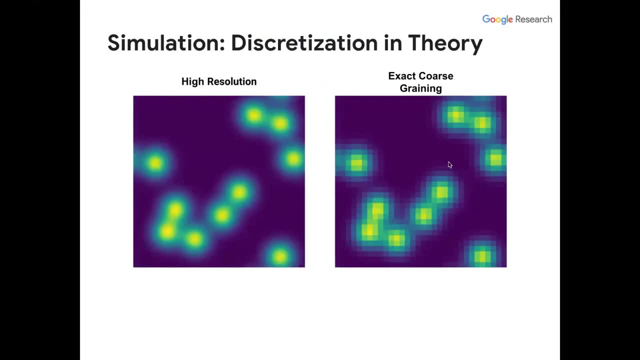 right is an exact coarse graining of the solution. So what we've done is taken the high resolution simulation, we've drawn it into smaller boxes, we've averaged the solution within the boxes and you're looking at the time course of it there. But what we want to ask is: suppose we solve the 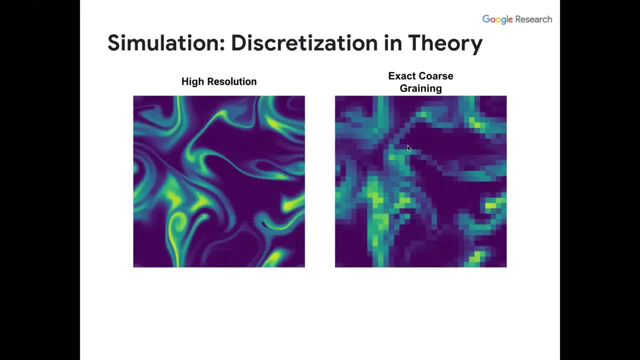 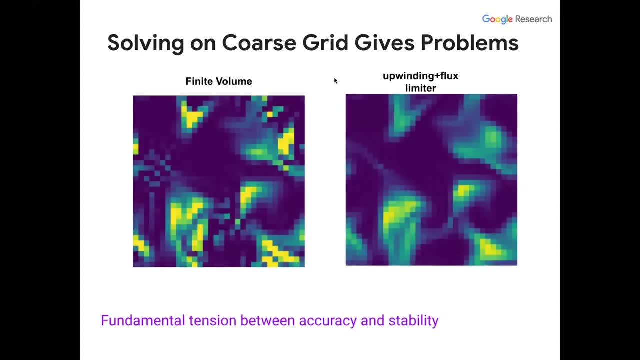 numerical method on the coarse grid instead of the fine grid. Can we get a stable time evolution operator to work on the coarse grid? Now, you all know better than I that, of course, if you try to do this, there are two classifications. There are two classifications. There are two classifications. 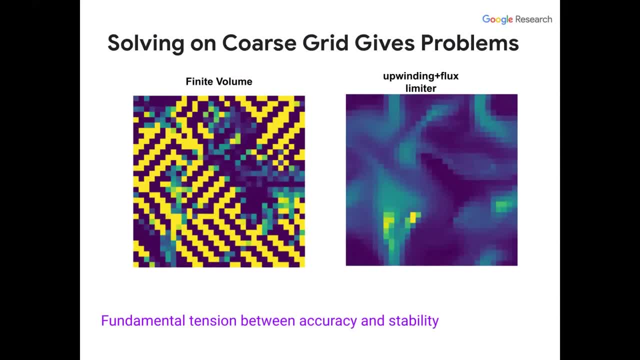 and there are two classifications. There are two classifications and there are two classifications- problems that occur with classical methods. So one is that if you use, for example, a simple finite volume method, that it's sort of easy to find coarse grid situations where 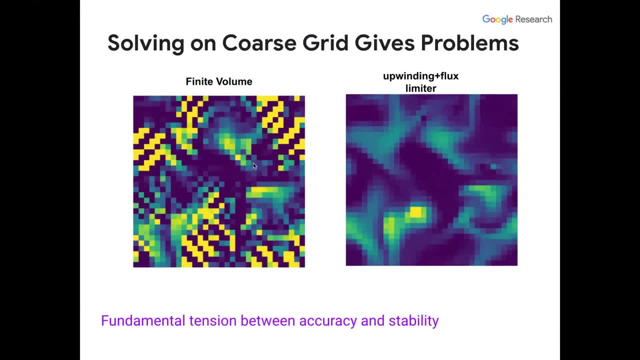 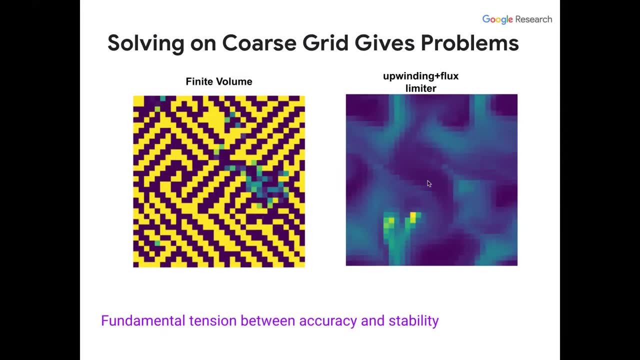 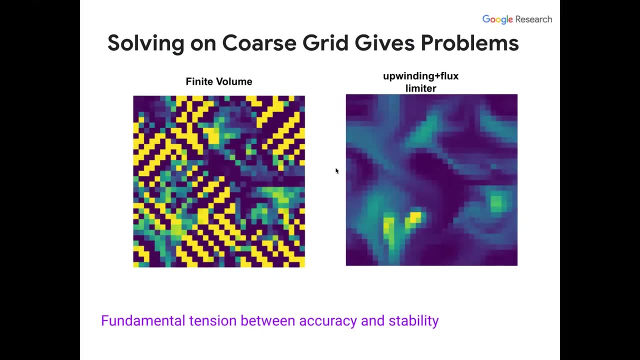 the solution destabilizes basically when you evolve it on the coarse grid, Or you can use a more fancy method and then the solution doesn't destabilize, but it blurs out And there is a canonical tension between accuracy and stability that we as a community have been forced to. 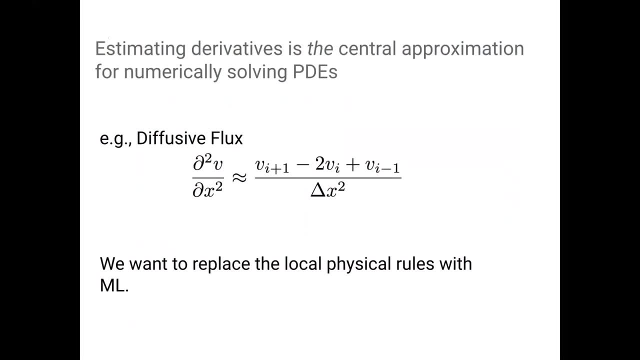 deal with. So this is the core of what we want to try to go after and what I'm going to tell you today. So what we're going to do is we're going to do things like take – so we want to learn equation-specific methods for numerically solving PDEs. So that is – I'm going to discuss a class. 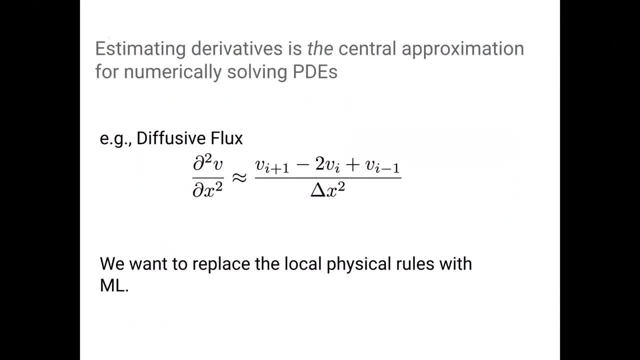 of methods which try to produce exact solutions that are coarse right on a coarser mesh than can ordinarily be done, but that the methods can only be applied to specific equations. So this is taking a hit from you know. an example analysis. On the other hand- and I guess I don't have to convince this group- we don't really care about that many equations. So actually, as long as you could do that for the right equations, it would be a big win. And what we're going to be doing are things like this: We're going to replace the derivative operator. So this is the discrete derivative operator that we 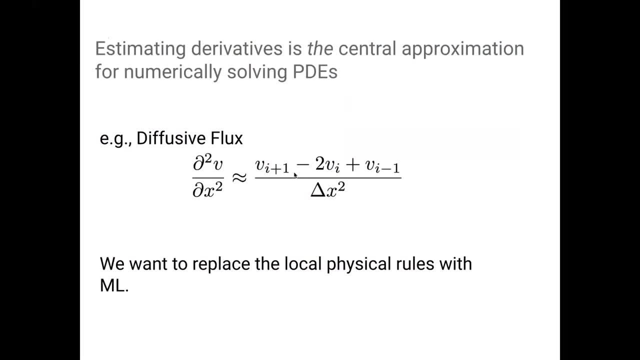 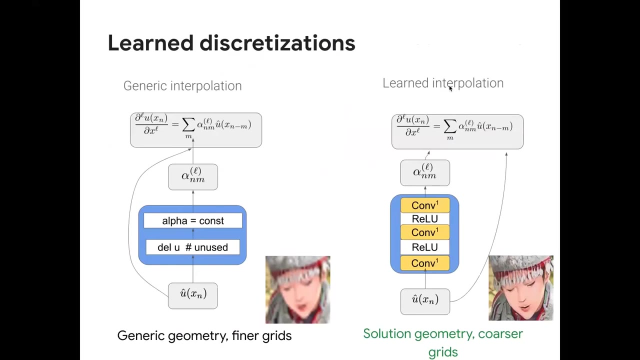 trivially derive from calculus. We're going to replace it with a machine-learned alternative. So we'll, for example, learn an interpolation that is typical for the solutions of an equation and use those to advance the solution in time. Okay, so here is the idea. Here is just an initial idea. So, as I said, we call this learned interpolations. So generic interpolations are sort of depicted on the left. I mean, you basically take the solutions at some mesh points and you basically, you know, 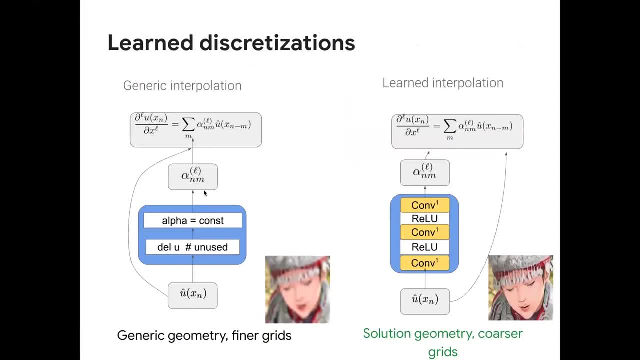 interpret with Lagrange polynomials or whatever basis set you'd like, and then take the derivatives of the formula to derive a discrete formula for the L-th derivative In learned interpolations. what we're going to do is we're going to take the solution at a discrete set of mesh points, We're going to send it through a neural network. 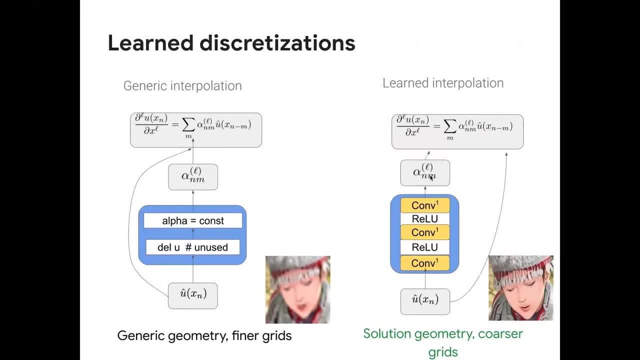 which will, you know, predict the interpolation weights alpha that it will learn based on data in a way. I will show you in a minute and then that will give the derivative formula. And so these are analogous, but in the case that I'm going to be telling you about, we're going to be learning the interpolation rates. 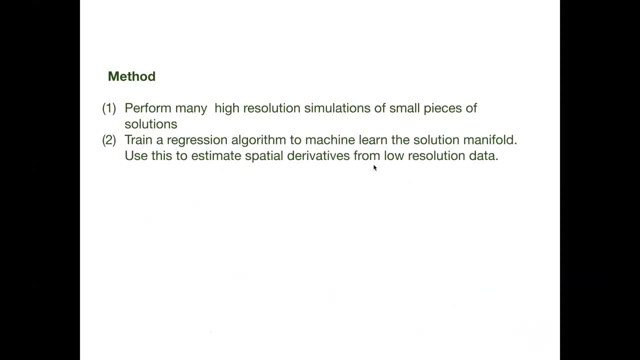 So okay, so the general method is the following: How do you learn the interpolation rates? Well, you need data. Where do you get data? Well, you simulate data And, in particular, we can simulate large numbers of small pieces of solutions. Notice the word small pieces. 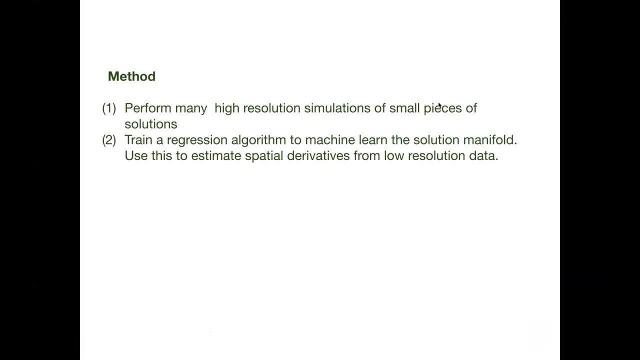 This is one of the ideas here that we're going to be trying to do. We're going to be trying to upscale locally and thus the hope is that, by you know, we don't have to do big simulations of fine resolution. We can do, you know, fine resolution of small pieces and stick them together to make the whole thing work. 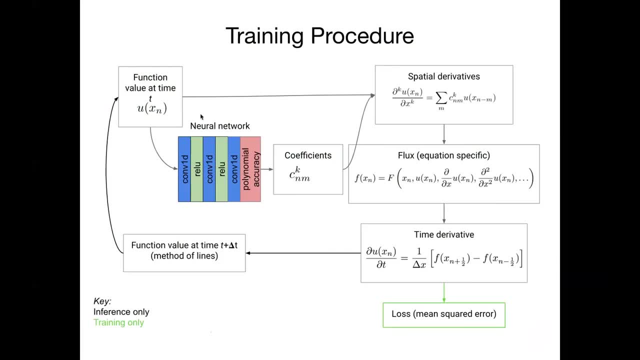 Okay, so here is the training procedure, So and so, what we're going to do is this is, as I said before, we're going to take the solution at time. T on the mesh points XN. feed them through a neural network. 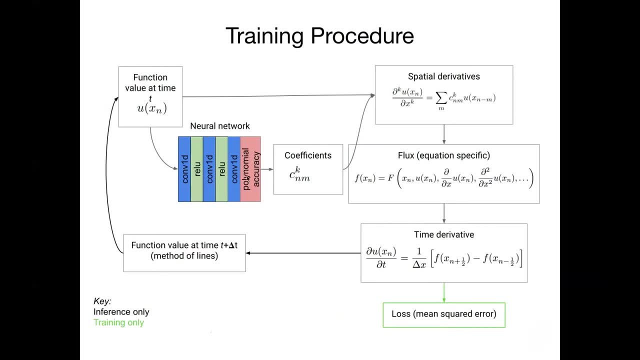 There's a polynomial accuracy layer at the end which basically takes the formula We're here predicting. I unfortunately changed notation between the pot slides. These are the weights in the derivative rules and we basically project these on the polynomial accuracy constraints to demand that the case derivative has some order, basically in the limit as the mesh spacing gets small. 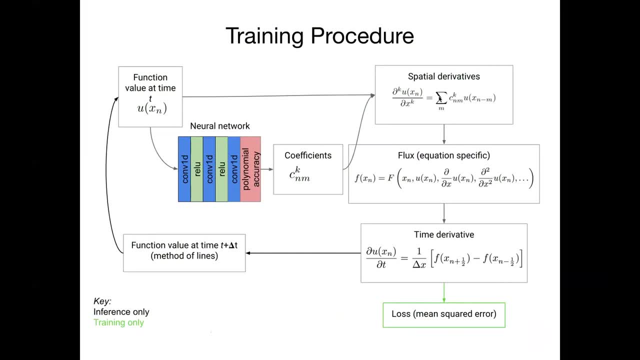 But of course the whole point is that we're going to be operating them outside of that regime. We then take these formulas for the derivatives. We basically compute fluxes from them, from the boxes. We we can compute the time derivative. 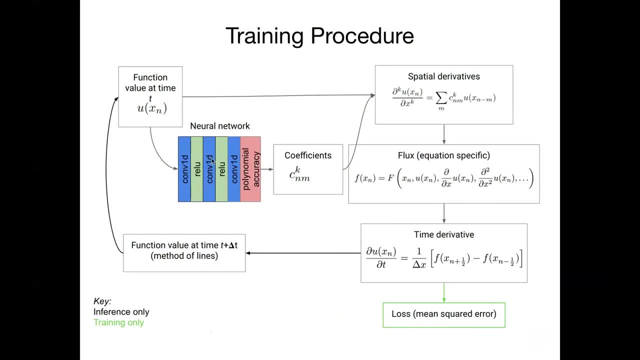 And then you know, if you know, if you've already learned The, the network to give you the coefficients, you can time evolve by just going around the loop. If you don't know the thing, then what you can do is you can train it by defining some loss which you can choose as you want to basically train the coefficients. 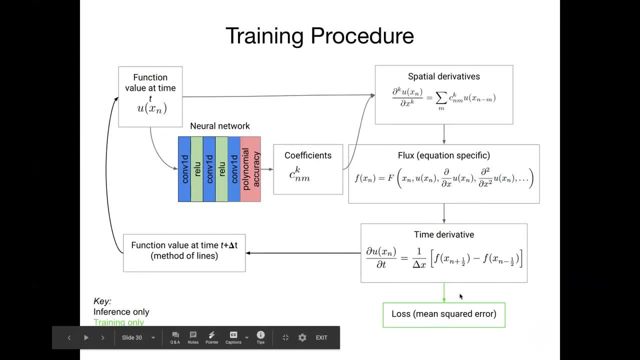 Now the way that we have trained this in the examples I'm going to give in today's talk is to, is to take fine resolution, high resolution solutions and to And to use them and to basically demand that on a course grid, we reproduce the. 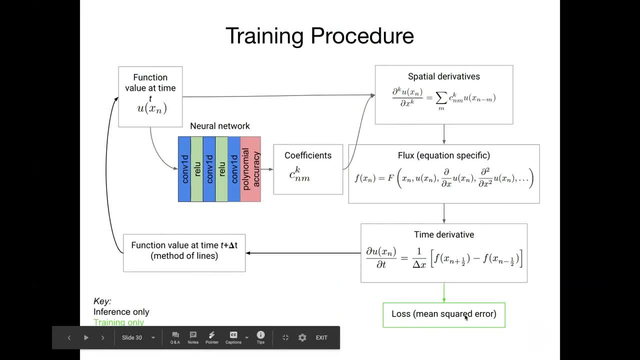 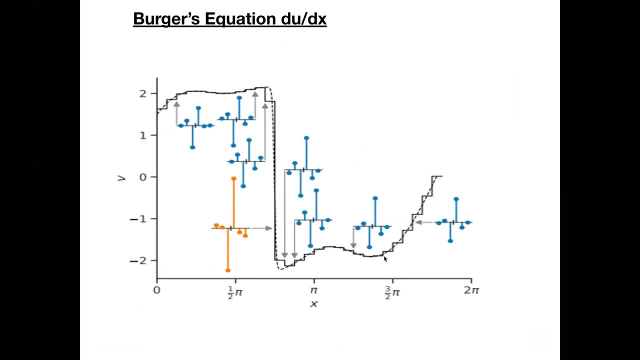 We reproduce point wise: the, the, the, the, the fine mesh solution, and that's the way that we train this. So so what does this give? So this is a solution to burgers equations. So these are the stencils that are given for the 1st derivative operator that is given out of this, And what you should notice is is that at different places in the solution there are different stencils. So the stencils depend on the solution. 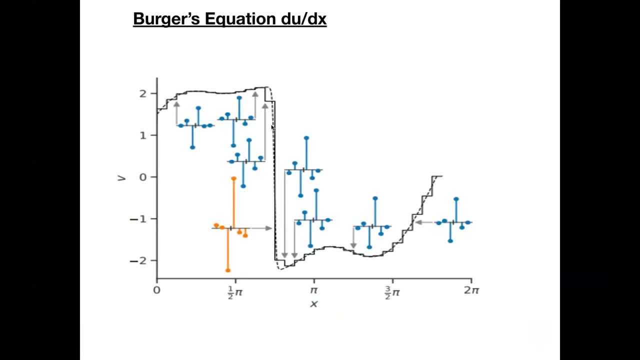 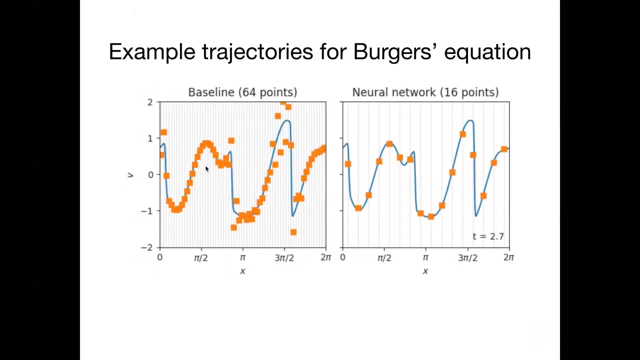 For example, the stencil for computing the derivative operator in the vicinity of the shock is different than that In a part of the The solution, where it's relatively smooth, and the algorithm learns this in order to basically maintain the sharpness of the shock. And so, basically, the summary is that this works, and I'm going to just show you some plots that this works, how this works in these 1 D examples. 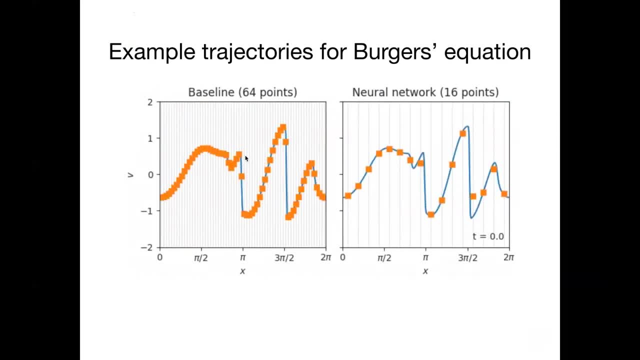 And then I will move on to turbulence. So this is a baseline method on the left which uses 64 points and you'll notice that it destabilizes. So this is the neural network, which basically means the discretization. So if you think of that matrix, 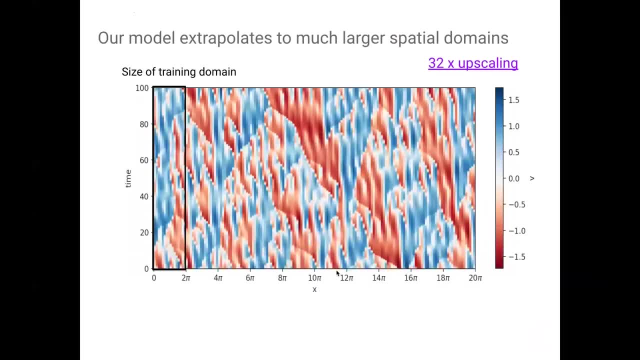 With a lot of neural network And with 16 points, it remains stable for a long times. So our model: we're able to use this to train it on small pieces because, since we're learning, what we're learning really are local features of the flow. we can train this locally And then, and then roll it out globally. 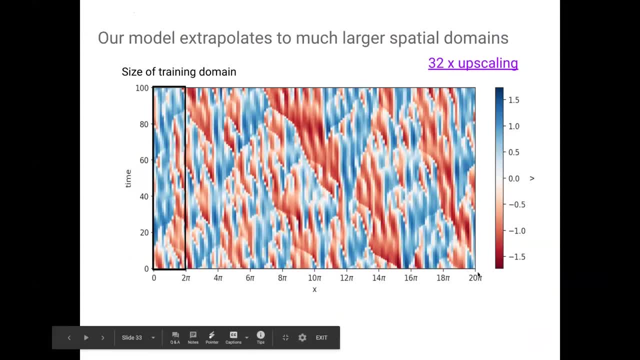 So the training domain for this solution, the burgers equation is: Is this black box? so it's from 0 to 2 PI. but here we've, We've solved for a solution Which is a box of size 20 pie and rolling it out in time. 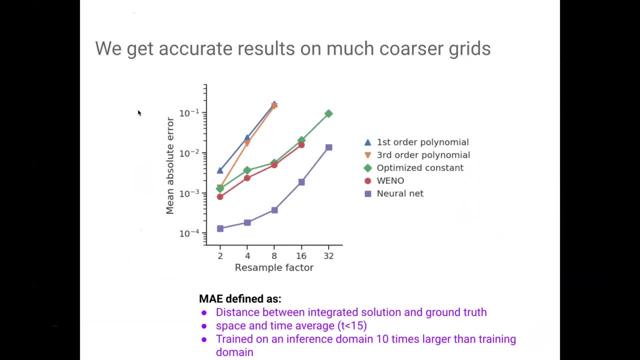 And this is with 32 times upscaling the solution. And then you can Like I mentioned from the baseline method. So let me just show you some numbers for accuracies in these 1D problems. So this plots the mean absolute error as a function of the resample factor. 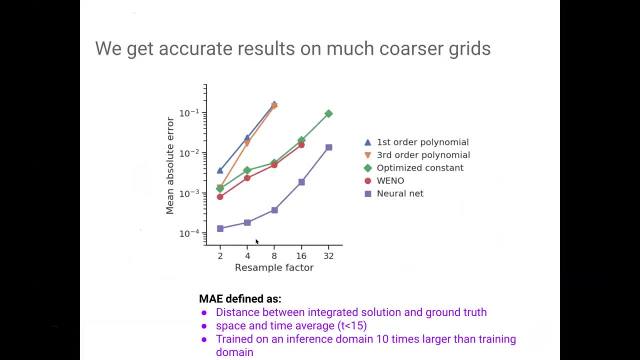 The resample factor is how much we've coarsened the grid over the high resolution solver. So these mean absolute errors are computed as the L2 distance between the integrated solution and the ground truth which was solved at high resolution. And we're doing both a space-time average where the solution is being solved. 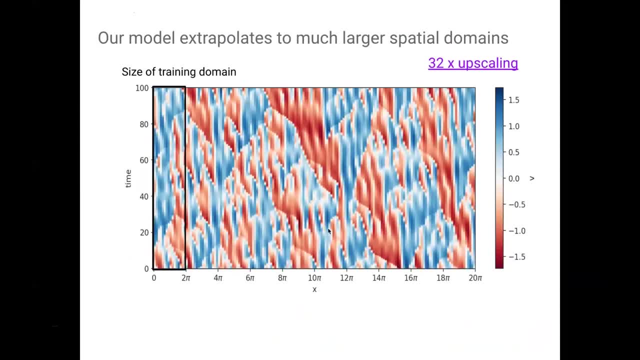 It's in a situation like this, where the domain is much larger than the training region. So we're integrating over all of space and we're integrating out in time to 15. So that's like looking in this part of a region. That's what this is- an error of. 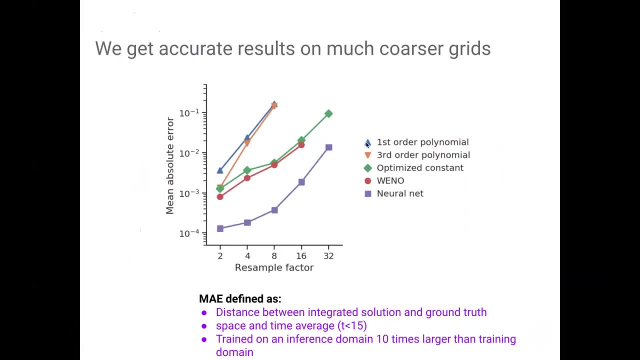 And this compares the error for a series of different methods. There's first-order and third-order, normal numerical methods. There's the WeKnow method, which is the state-of-the-art method with handcrafted coefficients for solving shock equations, And this purple is the neural network which outperforms it significantly. 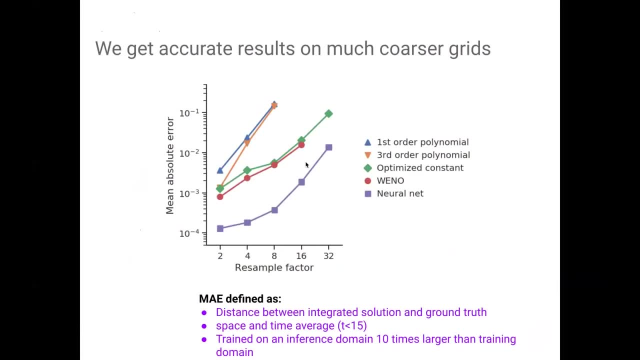 If we, in our optimized code, demand that the algorithm has constant coefficients so that they don't change in space, then we can actually find a method. The algorithm will converge onto a method that basically has the same accuracy, the WeKnow method. 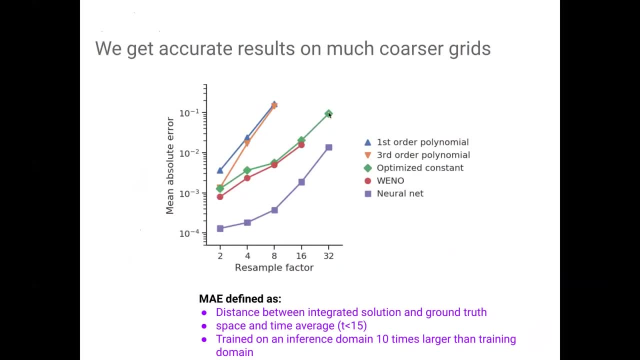 Actually, and just for the experts in the audience, we're going to use the same method, but that's only when we impose- I should have written this on this- that the green dots also have gotten-off type flux constraints imposed, which, of course, are very natural. 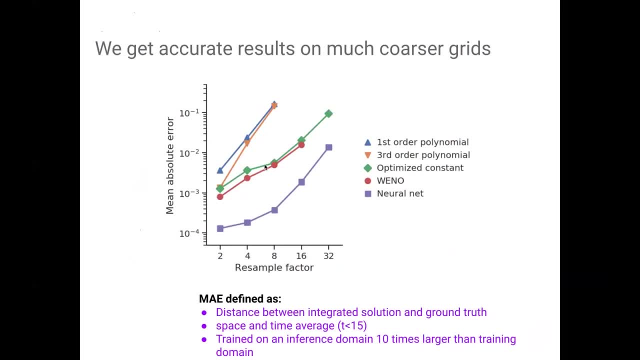 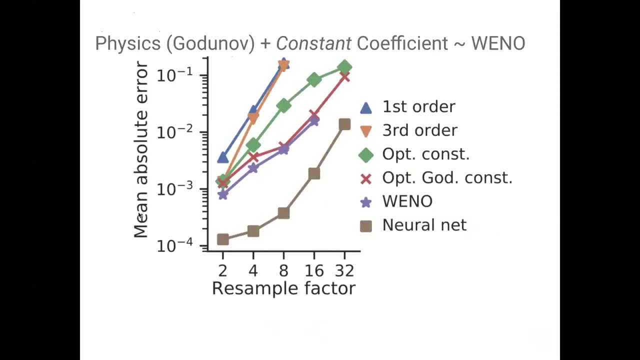 And so that which is sort of comforting to know that one can recover, you know, but then you can beat the ground, truth. So I'm going to skip these slides because I'm running out of time. We did this on lots of equations. 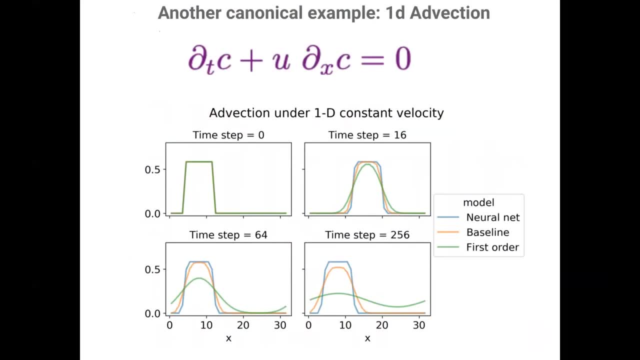 It generally works. There's a. if any of you are interested in this and you want an example, there's a simplest example you can possibly imagine is 1D advection, where we also did this, And actually Xiaowei Zhuang, who's an atmospheric chemistry graduate student. 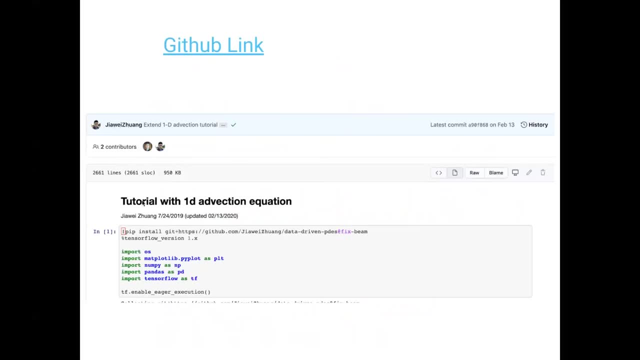 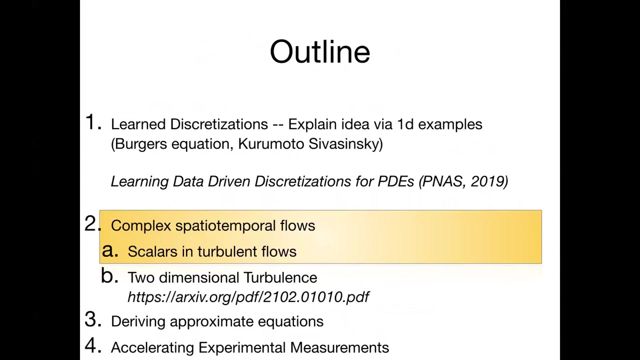 at Harvard did this and posted this to his GitHub site, a tutorial on using this with his with the advection equation, which is a nice way to sort of see how this works. And that is that. So I'm now going to move on to talk about more complicated turbulent flows. 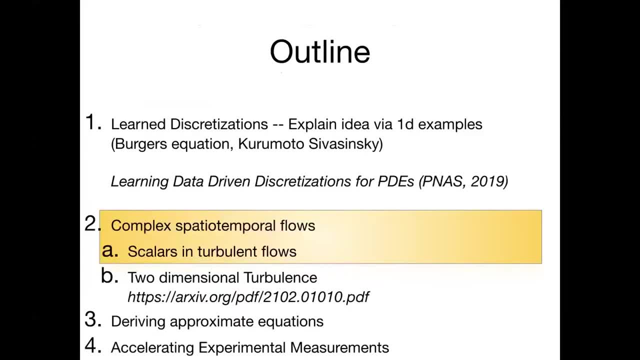 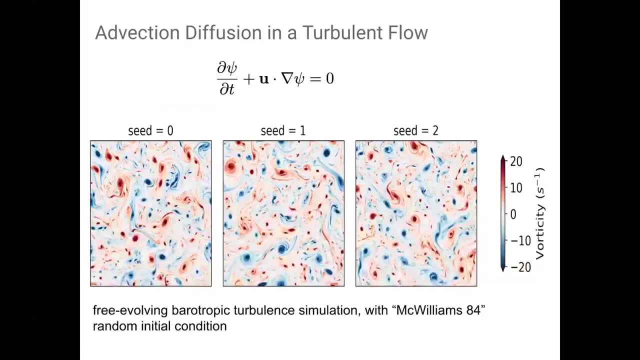 Actually in the talk I had passive scalars and turbulent flows and 2D turbulence, but I'm going to just skip that, Skip right ahead to 2D turbulence, if that's okay, unless anyone has anything to say. So I'm going to. does anybody have anything to say? 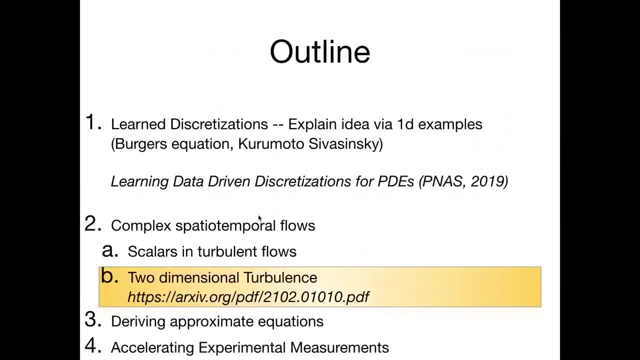 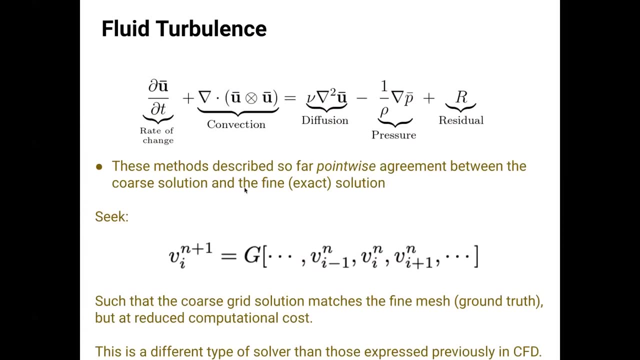 I don't see anything in the chat. Okay, cool. So so okay. This, as I said, is based on a paper that was that was just posted last week, So okay. So we're interested in seeing if we can apply these methods to the Navier-Stokes equations. 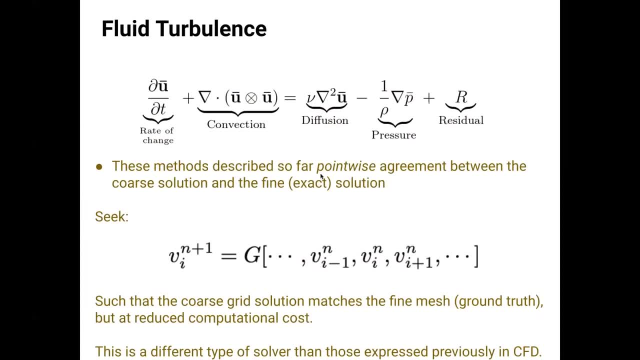 And so what we seek, so and what I've described so far, so what's sort of unusual, I think, about the methods that we've that I've described, is that the is that you know in opposition to, for example, you know, LES models or models that use eddy viscosities, which are trying. 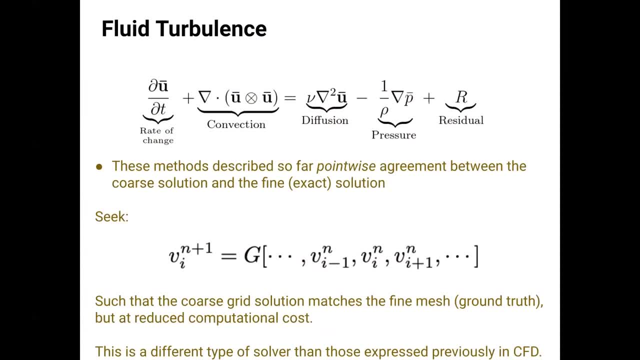 to capture local statistical properties of the flows. here we're trying to demand point-wise agreement between the coarse solution and the fine solution, And what we're seeking are numerical update rules. We want numerical update rules that basically allow you to to stably integrate the equation on long rollouts, in which the the coarse 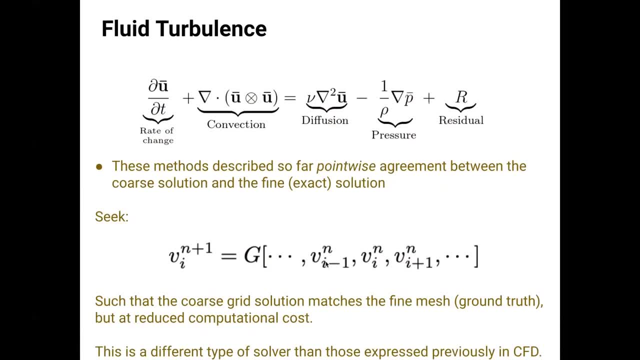 the coarse grid solution hits the, the accuracy of the fine mesh, but of course at significantly, one would hope- reduce computational costs because the grid is coarser. So this seems to be a sort of different type of solver, And- and this is, and what we're trying to figure out here is, is how well this, this, can work. 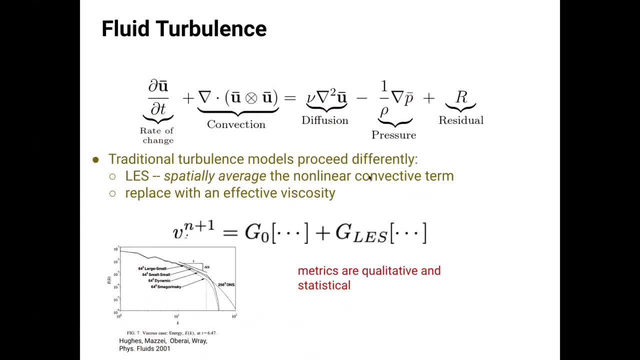 And I guess I I have this comment here that traditional turbulence models proceed differently. I mean LES, For example, spatially averages, the nonlinear convective flows term. So you know, you can you compute an averaging operator of the whole equation. 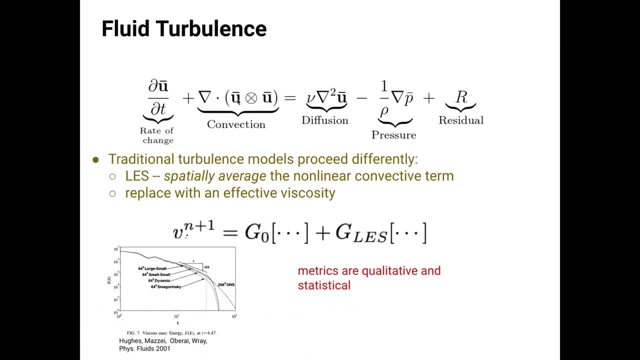 And then once you have an averaging operator of this, you have to model it and and you know it ends up being an effective viscosity or something. And in for LES models comparing with with direct numerical simulations, the metrics tend to be statistical, like showing that spectra agree. 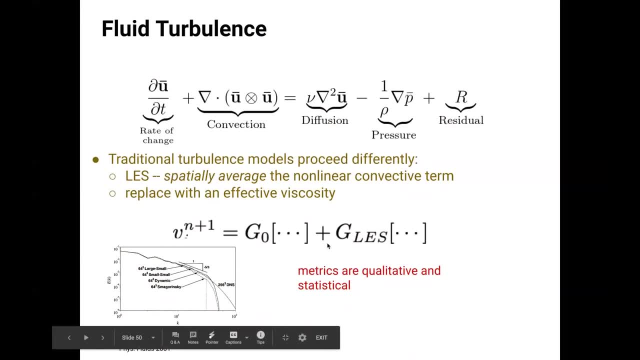 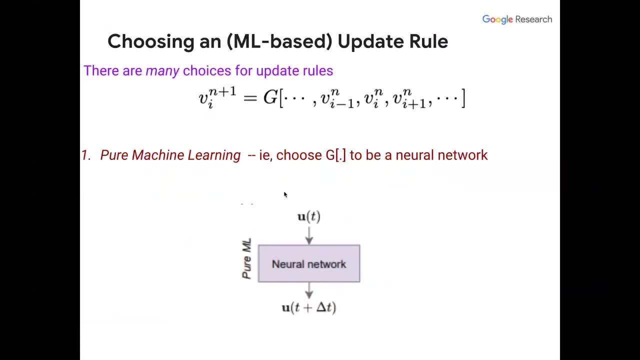 This is a classic LES paper and qualitative, Whereas here we're, we're really going- and this may be insane, but this is what we're doing- is we're going after point-wise agreement, So okay. So I want to just make a comment about update rules. 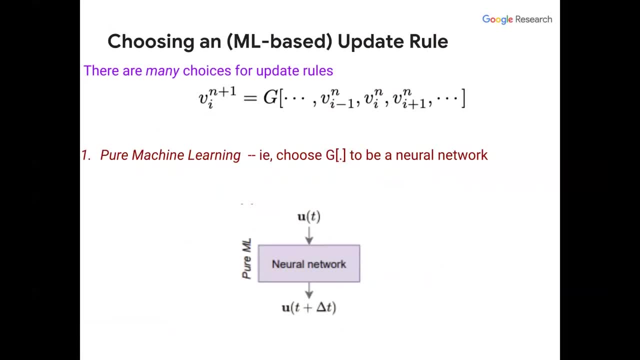 So classically, of course, you know, when we teach numerical analysis we derive update rules. We teach classes on how do you derive from calculus update rules. If one uses machine learning, there are lots of choices for update rules And I just want to acknowledge them all upfront because I don't think it's. it's. 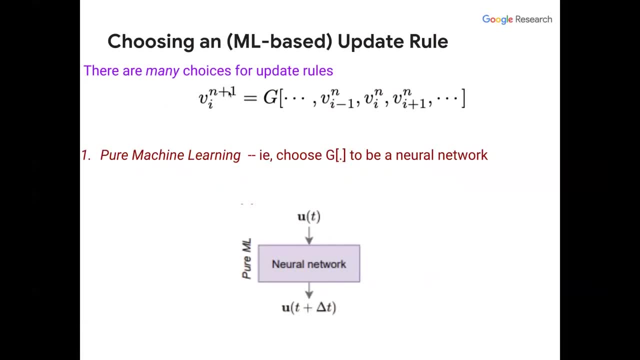 there's no theorem that states that one is better than the other. So an example of an interesting update rule is a pure machine learning update rule. Namely what I just showed you was about learning a discretization which was really using the structure of the equation in great detail. 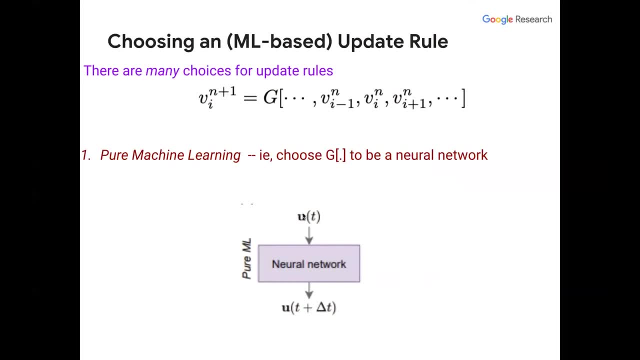 But you don't need to do that. I mean what you can do and what people do is you could just basically say: let's forget the equation. I'm just going to replace it with a neural network, and that will be my update rule. 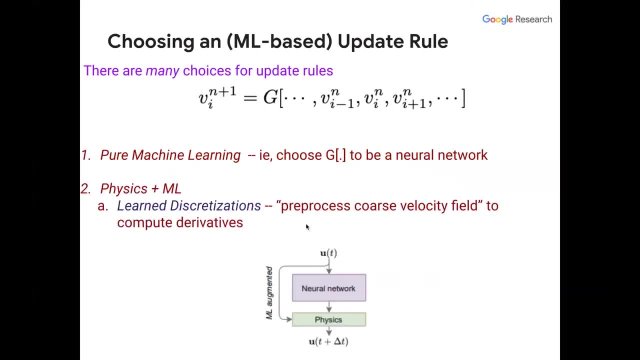 So that's a perfectly reasonable update rule. So another thing you can do is you could combine the update rule with physics in some way, And this, basically block diagram, represents what I showed you a moment ago, which is learn discretizations. What we do is we take the solution and we pre-process. 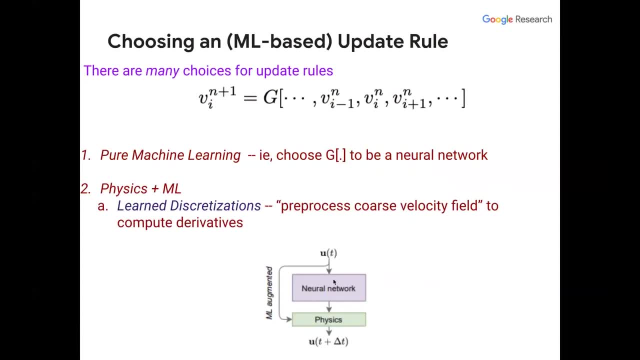 It into a neural network, to get the, to get the, the, The interpolation coefficients, to then put into a normal physics solver and and so. so this is, this is a sort of a pre processing, and that's another type of an update rule. 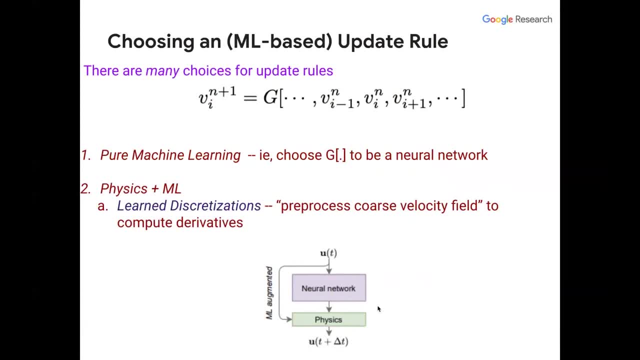 No. 1 would hope, and actually I'm going to show you that, basically by including physics in the solver, at least what we see is that the solver becomes much more generalizable than it does Otherwise. so 1 would hope that there was. 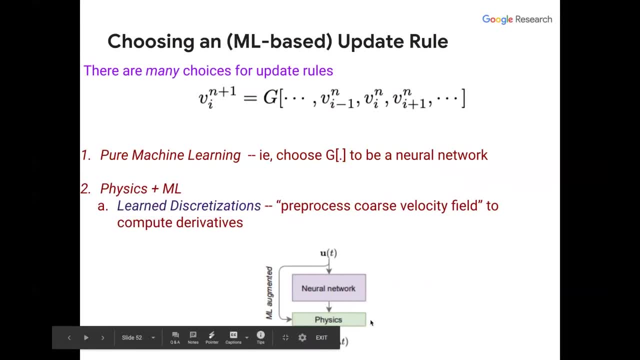 An advantage to doing something like this, but I think it's an open question as to how best to do this. So this is a 2nd way of choosing an update rule. Oh, and, actually I should say so. here is the particular way that we, the update rule, and what I'm about to show you works. 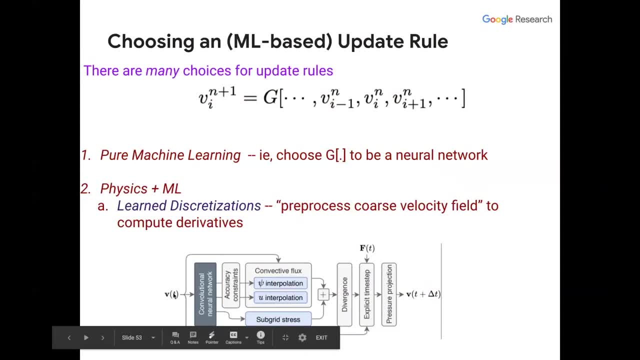 So what we do is we take the input velocity field- This is going to be intuitive spatial dimensions in this talk- and we We push it through a neural network to get interpolation coefficients, as I said before, to compute the convective fluxes. 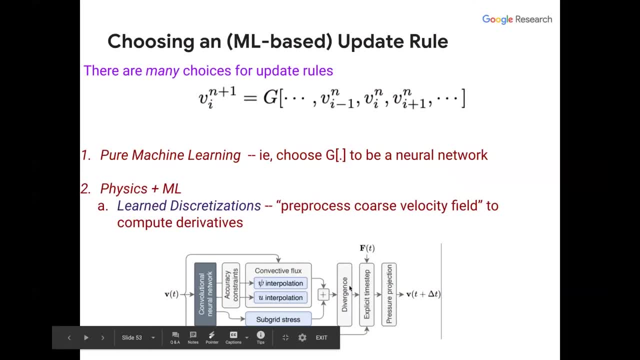 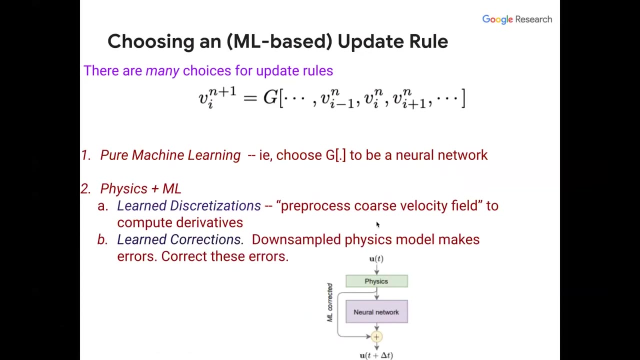 We then basically, you know, conserve mass, we time step and we do a projection, pressure, projection onto divergence, free velocity fields, And that is the block that's going to be used in what I'm going to describe to in a moment. So another approach that 1 could use- and I think this is also an interesting approach- is that 1 could start with the numerical discretization, and that's what I mean by physics in this spot, but on a course mesh. 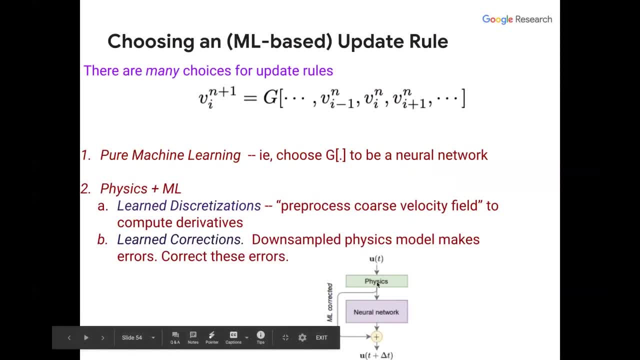 And 1 could then say that, oh well, I'm going to use. And 1 could then say that, oh, I made a mistake, because you know the mesh is course and you could sort of train a neural network as a corrector to it, And that's a. we call that: learn corrections. 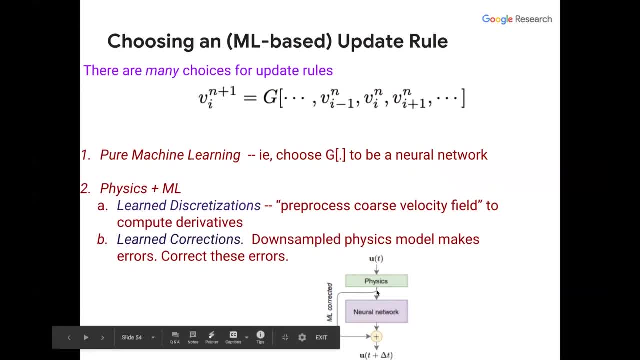 And that's a sort of another approach to including update rule, And there are probably more versions of update rules that 1 could consider And I mean I think generally what we, the community needs to do is try them all and see what works better for the for the purposes. 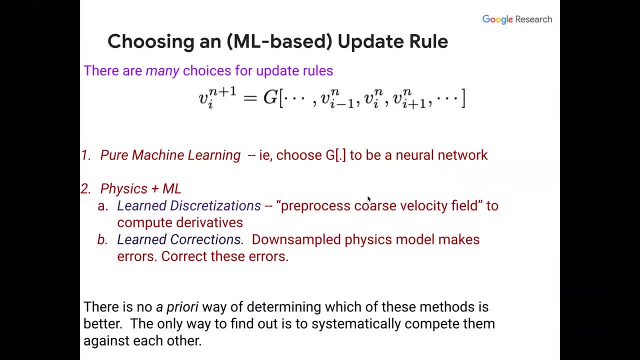 So there's no way of determining which 1 of these is better. The only way, at least not now, in our like steam engine before car, no version of the world with no theory, The only thing we can do is systematically compete them against each other, And that's what I'm about to show you. 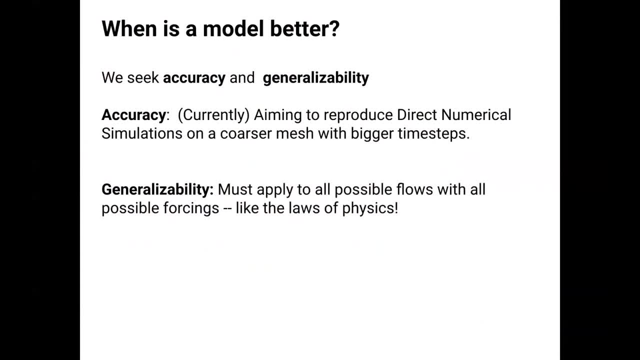 So okay. so the other thing I want to talk about before I show you results is: what does it mean for a model to be better? So this is an important comment, because there's a lot of results out there and there's a lot of things 1 can do, And I think we have to be careful. 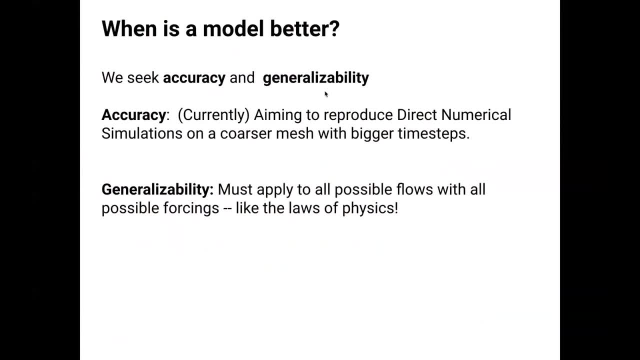 So we need both accuracy and generalize ability. I've already told you about accuracy. Our current approach to- Although 1 could easily adopt other metrics- is to reproduce DNS on a course of mesh with bigger timestamps. So, generalized ability. we're interested in solving the laws of physics, and the laws of physics have this wonderful property that I changed the situation. 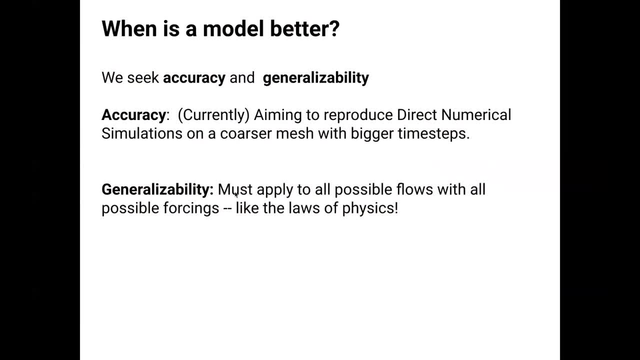 Then it still works and we really require that, should require that- as a consequence of our update rule. So we, for that reason, have designed a set of generalization tests and I will show you them in a 2nd, but they are sort of different hierarchies. 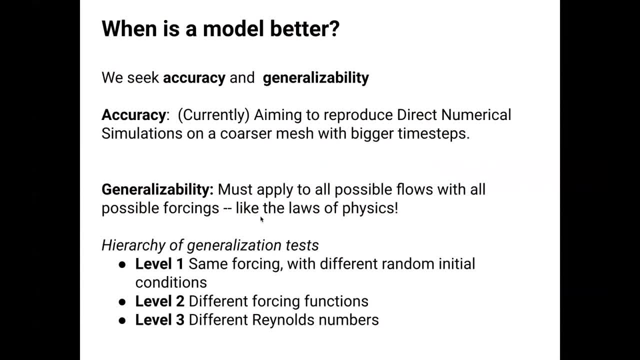 Of difficulty and I think this is important. So the simplest generalization test is like the sort I showed you in the 1 day, which is the. what you do is you solve the thing, Like you solve the equations with some initial condition and you train it on that with some force, And then what you do is: 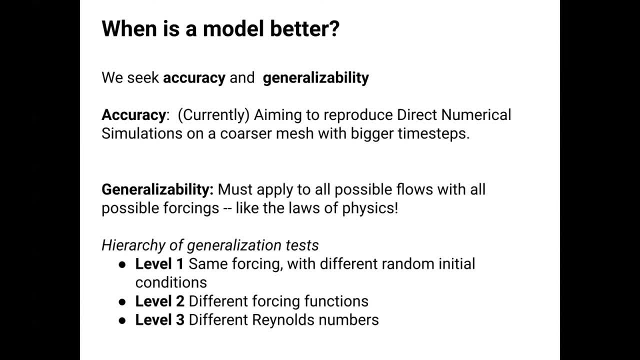 The generalization. you choose different, random initial conditions. So these are initial conditions and those flows that weren't in the initial set, and so they are legitimately called test sets. That is, a Is independent of the way that it was trained, but it's a very weak test set in the sense that you know, we all know that the solutions are chaotic anyway and they evolve in little blocks, So there's not a lot of generalization there. 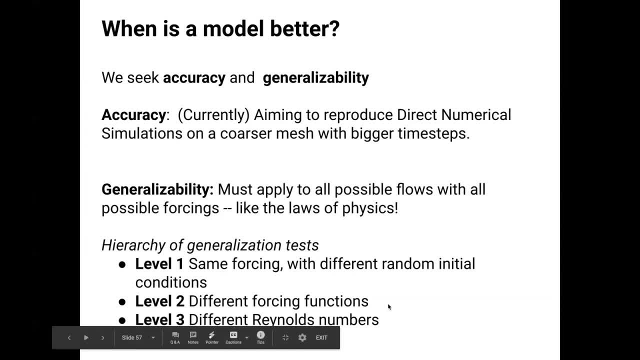 So the next level of generalization test is different- forcing- and the next letter of general, of level generalization test, which is even harder, is different rounds numbers which you know, namely changing equations, which, for turbulent flows, is something which is reasonable to think about because of the well known universality of turbulent flows as the rounds number gets large. 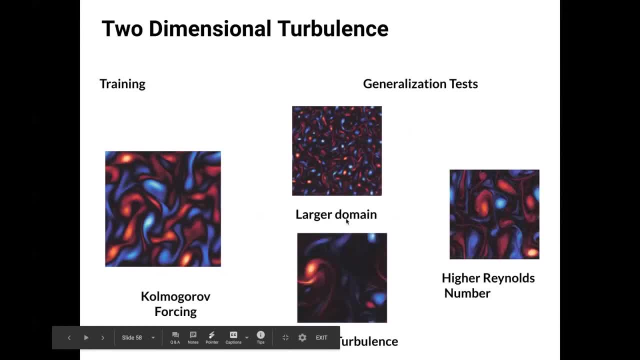 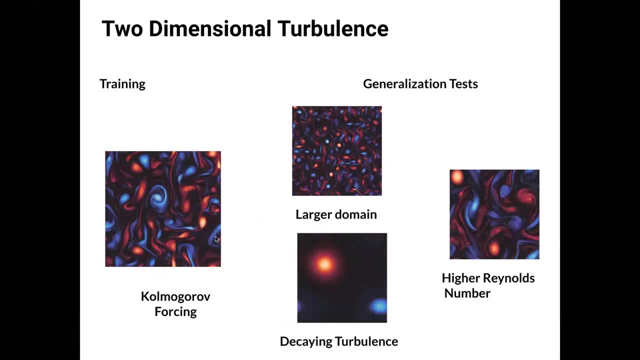 And So. so, with that in mind, what I'm about to show you are results on 2 dimensional turbulence. So we have what we do for training. is we choose a particular example of force 2 D turbulence, which is forcing, which was invented by, which is called forcing. 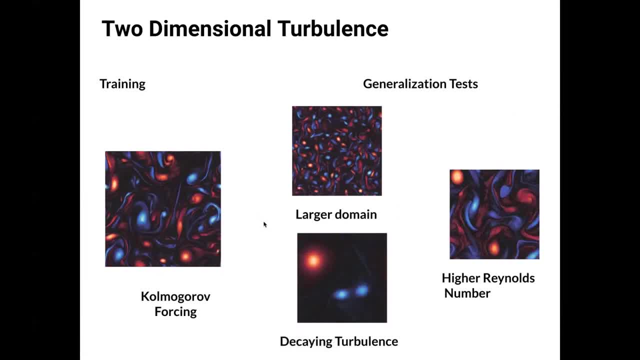 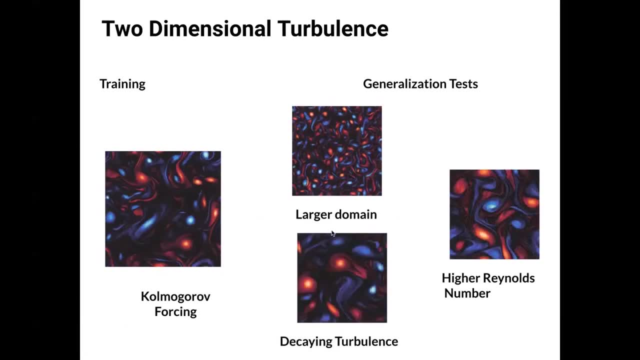 And we then have a set of generalization tests in addition to the different random initial conditions. We do generalization test by increasing the size of the domain. We do generalization test by turning the forcing off and letting it decays And finally we do generalization test it. 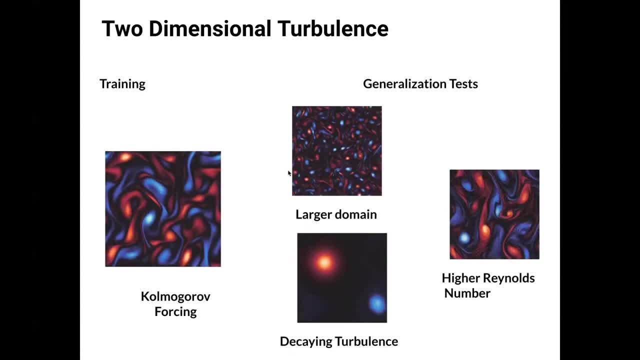 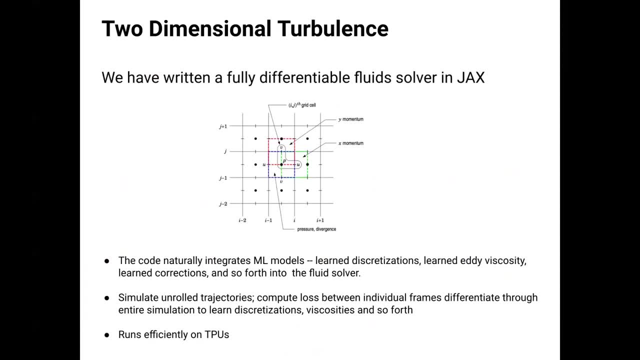 We do generalization test, which we do in the 3 dimensional turbulence, which, by restricting the forces, we require higher Reynolds numbers, And what I want to do right now- and it's almost 330, but I'm gonna take another couple of minutes- is just walk you through what we found. 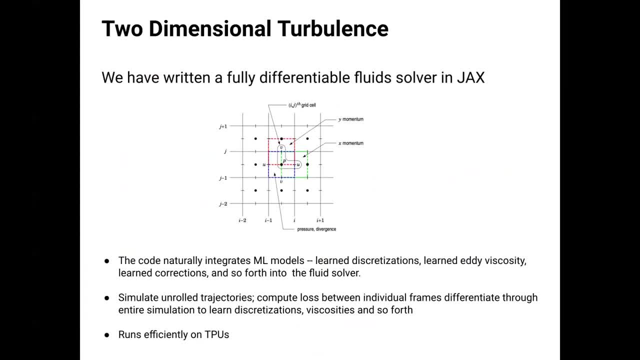 From this. So okay, so the results I'm going to show you are from a fully differentiable fluid Mechanics solver that we wrote in jacks that will be open sourced, hopefully very soon. It basically is it, It, it, it, it's a finite volume solver that. 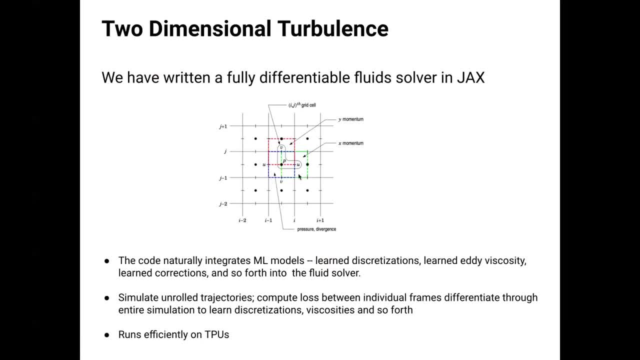 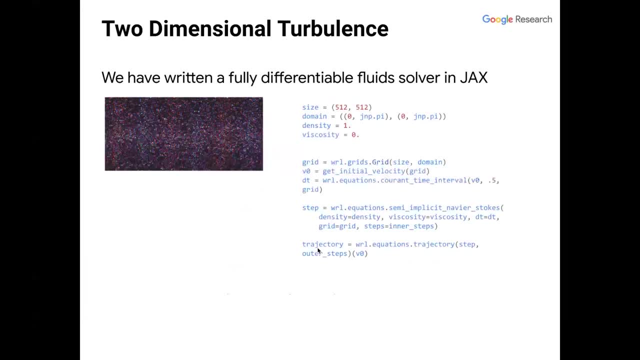 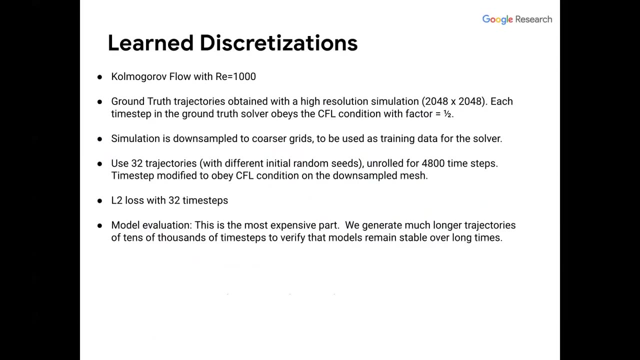 scheme showed here, And the beauty of it is it's fully differentiable and so we can easily incorporate machine learning at wherever we want in this and compete things against each other. So here's a little snippet of code of how it works. I'm not going to belabor it, Okay. 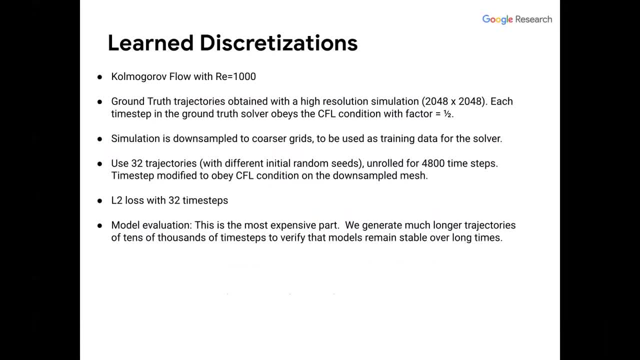 so these are results. So what we did was- and I'm going to first start with learned discretizations- is: we considered Kolmogorov flow with Reynolds, number 1,000.. And we trained ground truth solutions, trajectories with high resolution simulations, which were 2048. 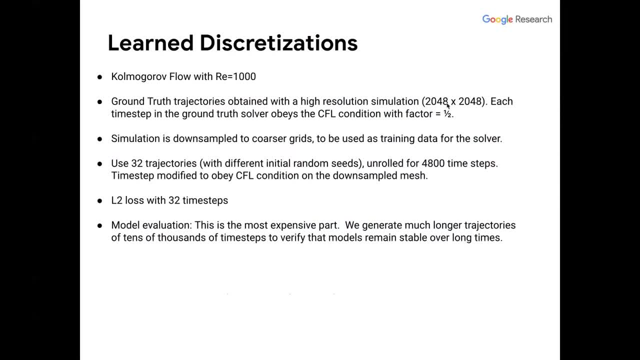 squared. So we demanded that each time step in the ground, truth solver obeyed the CFL condition with a factor of a half, with a safety factor of a half, So DT scales with DX. We then downsampled this to coarser grids to be used as training data. When we downsampled it. 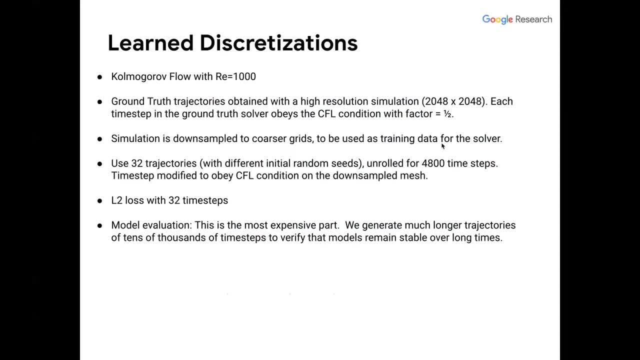 we also downsampled the time to maintain the CFL condition on the coarser grid With a factor of a half. In order to train the model that I'm about to show you, we use 32 trajectories, each of which has different initial random seeds, and we unroll it for 4800. 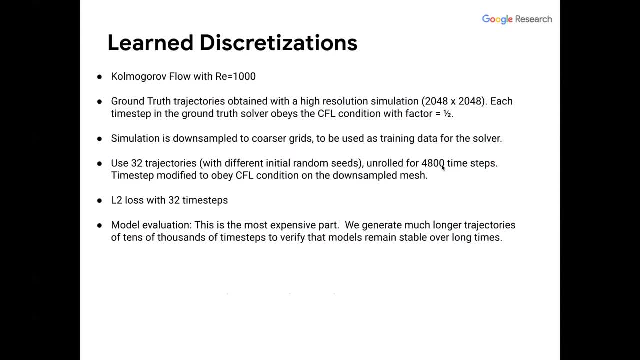 time steps And we basically train it with an L2 loss, basically in accordance with what I was trying to say. So, in order to evaluate the models, this turns out to be very expensive. The reason that model evaluation is expensive is that we really- you know, these update rules. 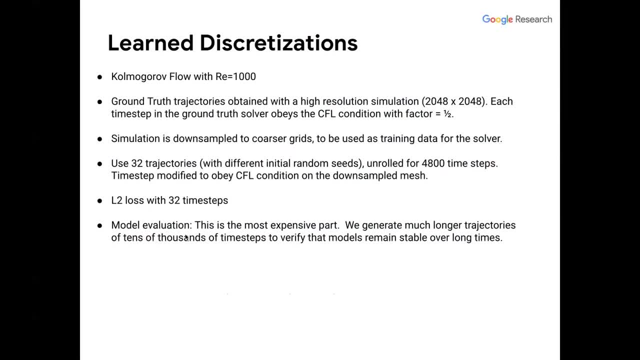 the most important property of them is that they are are stable on long rollouts, And the only way that one can check stability and accuracy on long rollouts is to generate much longer trajectories and verify that they remain stable over those times, And so that's what we did. The evaluation part is over tens of 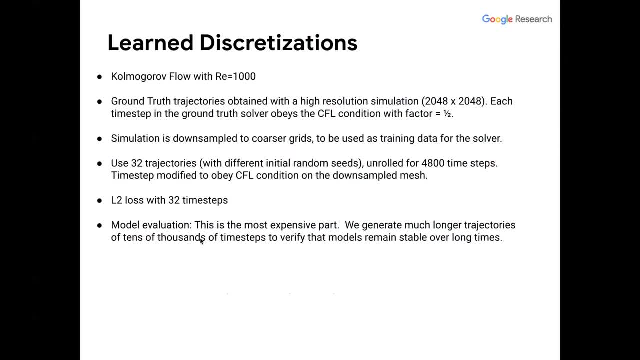 thousands of time steps Of course beyond a certain amount of time, the solution is chaotic, And so you can't expect pointwise accuracy anymore, because when you're well beyond the Lyapunov time, but at that point we can check statistical accuracy and statistical stability. 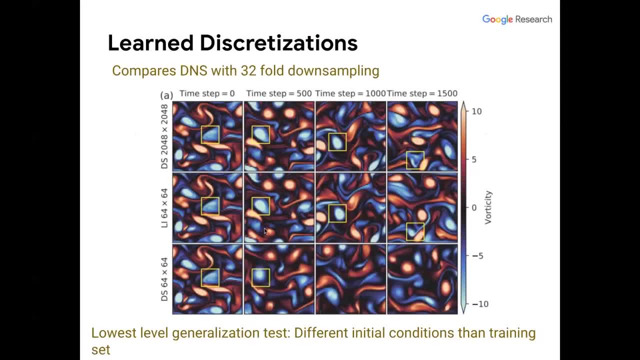 We do So, okay. So I'm going to start by um showing you the simplest example of a test set. So this is a test set which, um, which was just a different, random initial condition And the the ground truth solution is is at the top. 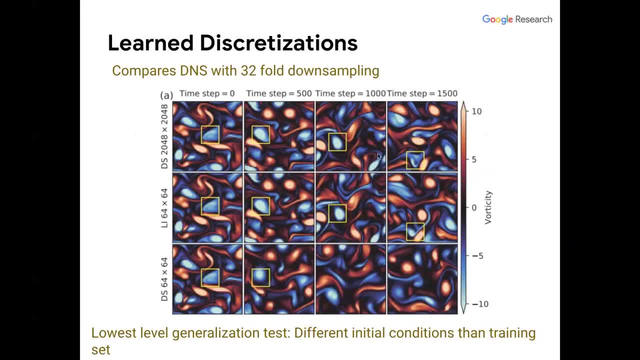 here It's 2048 squared and this is rolled out for 1500 time steps. So the, the, the DNS solution that's downscaled by 32, a factor of 32, this is on. this is DNS. the bottom row, Um, you'll notice. 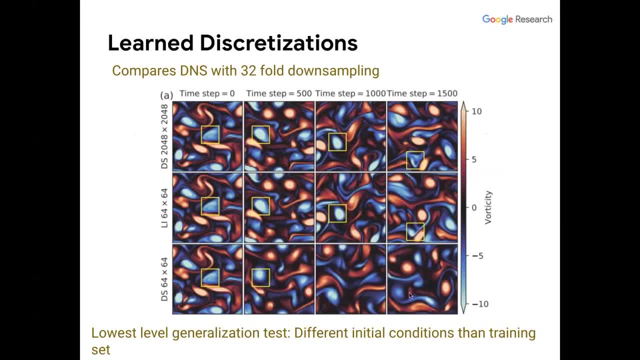 it sort of craps out very quickly, um, because of numerical diffusion, the learned interpolation model on the same Mesh. basically, though, um well captures the solution. So this is the lowest level generalization test that one has, but in this case the learned interpolation model passes. moreover, we can use 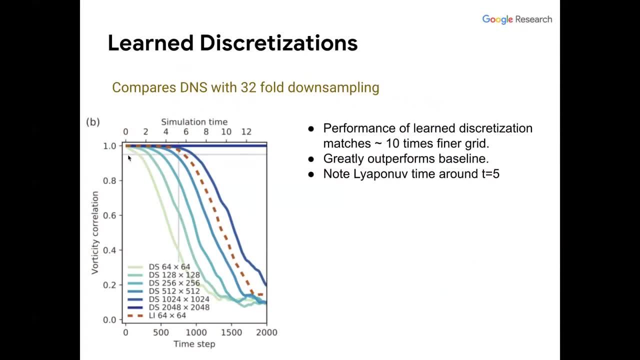 this, to study this quantitatively. And so to do this quantitatively, let me show you a plot. So this is the vorticity correlation as a function of time step and these curves. So the 2048 ground truth is um is this curve here? This is 1024.. The red dashed line is our 64 by 64 learned. 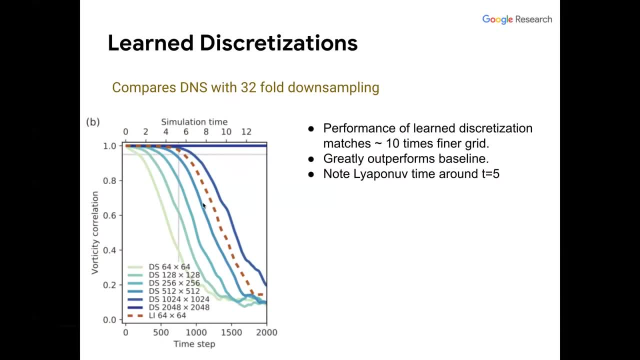 interpolation model, This is 512 squared, And so what you see is- and this, this vertical dashed line here is the Lyapunov time, So actually beyond this time, there's exponential divergence of trajectories. What you see is that we basically achieve the same performance as a grid, which is ten times. 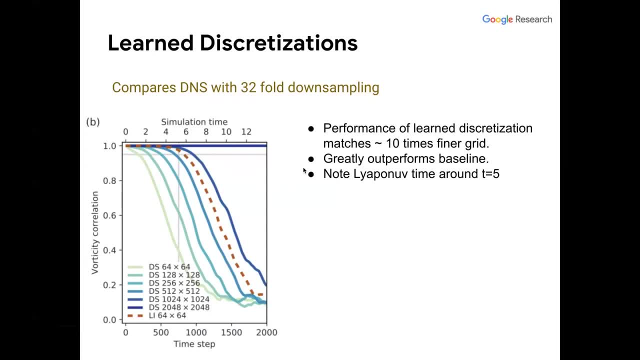 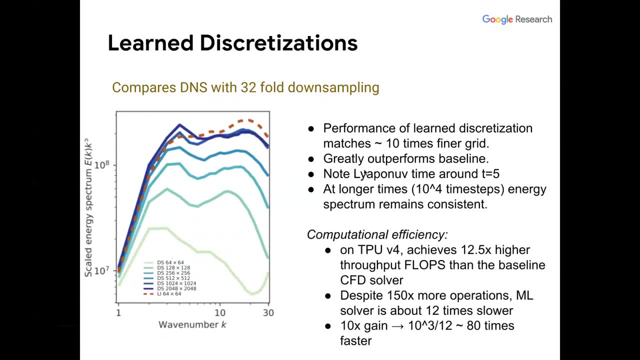 Finer using this model and this is maintained. If you look at spectral accuracy over much longer time steps, the spectrum basically remains constant. So and now- and this is, I think, is extremely important in terms of computational efficiency. So we ran these experiments on TPUV4s and basically the deal is that the ML models 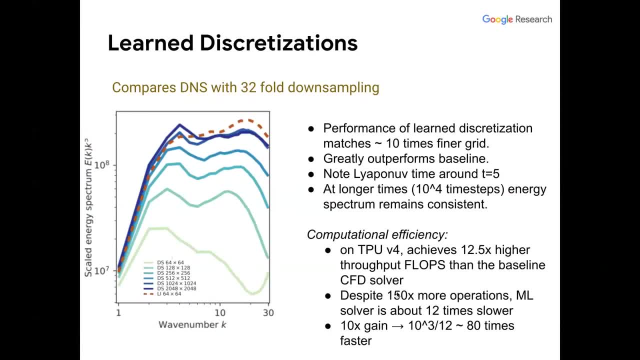 of course require more numerical operations because we have to compute these neural networks at every grid point. So there are about 150 times more operations in the ML solver than the baseline CFD solver, But because of the TPU and the high throughput in terms of flops, it turns out only to be. 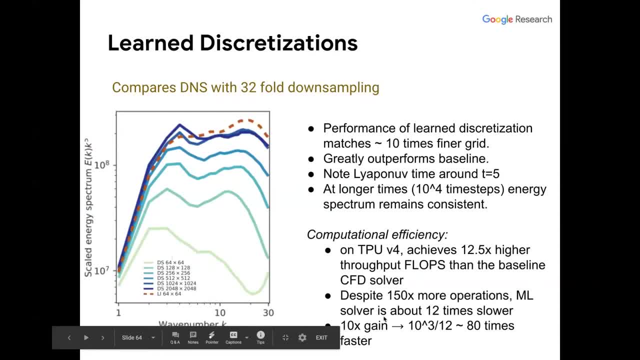 about 12 times slower. Now I told you that we have a 10x gain in terms of upscaling from the grid, So that results in a time savings of 10x cubed because there are two for space and one for time. 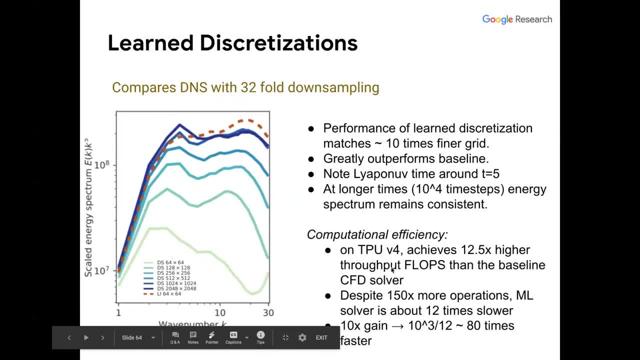 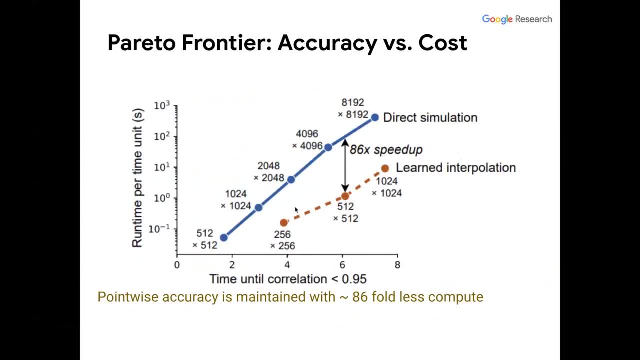 And then if you divide by 12, that's about 80 times faster for the ML model. And just to sort of drive home, we said, well, we're going to do this. We sort of did extensive tests on this, basically for upscalings of different you know for. 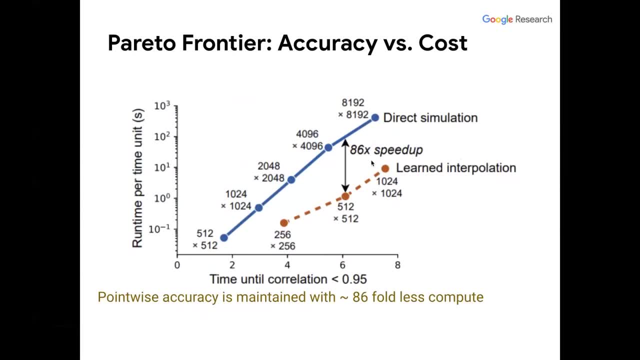 downsamplings of different size meshes And what we see over. so this is plotting the runtime per step as a function of the time at which the correlation between the solver ends up being less than some threshold, which we just chose to be 95%. 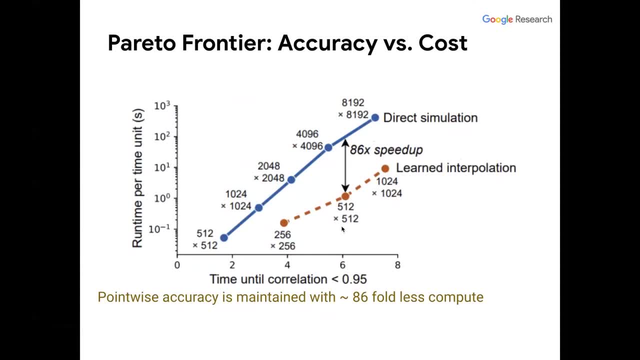 And what you see is that we're able to achieve the same accuracy with about a factor of 86, about a factor of 86 faster. So that's the, so that sort of switches, the, You know, the, the, the, the, the line in this trade-off from, you know, standard algorithm. 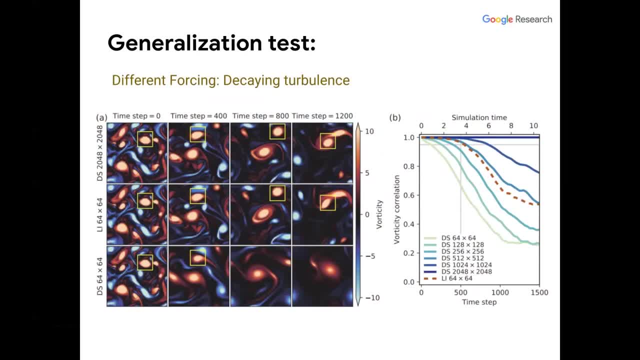 So now let me just quickly flip through some generalization tests and then I will end, because I know I'm reaching time. So this is the same thing, except that now we're using decaying turbulence. So I want to emphasize: what I'm about to show you is with the same model that was trained. 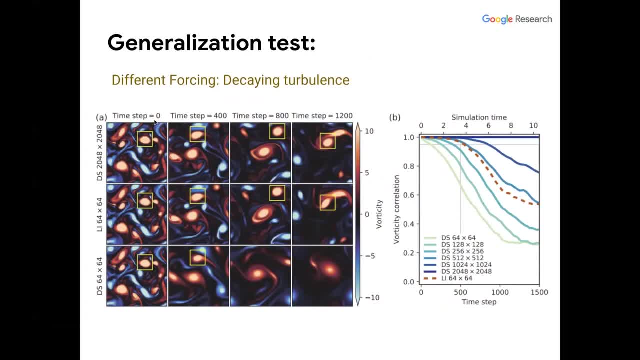 before. we have not retrained the model Um, so this is decaying turbulence. Here's the 2048 squared baseline. This is DNS. I mean, this is the DNS at 64 squared which drops off quickly. This is the learned interpolation. 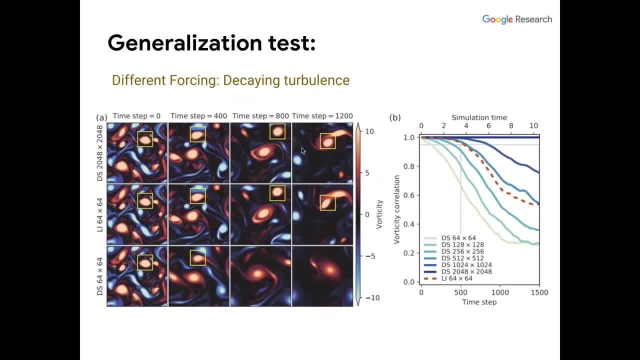 You see, we've put boxes around The vertical structure so that you can see that it's tracked. If you look at vorticity correlation as a function of time, we're not doing better now than the, than the um, than the five, 12, slightly worse, but this is about a factor of seven or eight. 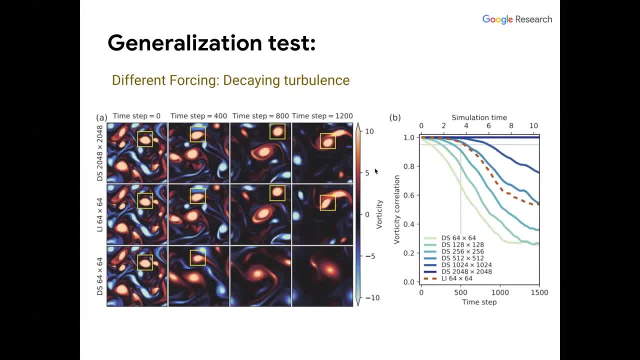 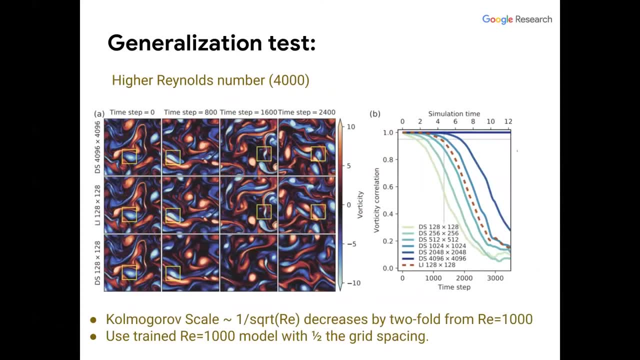 times upscaling um over before, while maintaining the same accuracy. So this is the hardest generalization test is to go up to higher Reynolds numbers, And I need to explain this briefly. So if you believe in the turbulent cascade, then what you, what you, what you might imagine is: 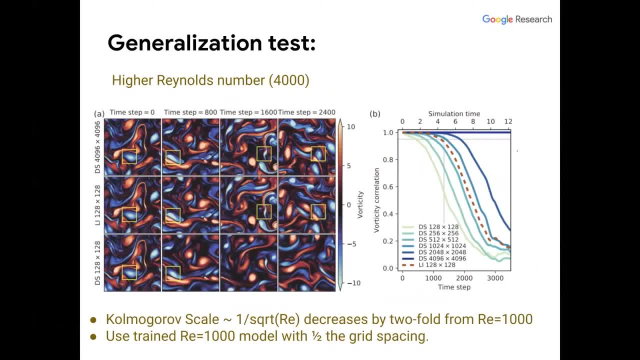 that what these things are doing is learning the, the, The solutions around the smallest scale eddies, and building numerical algorithms around them. Now, in 2d turbulence, the comagraph scale, namely the, the scale at which dissipation kicks in um, scales like one over the squared of Reynolds number. 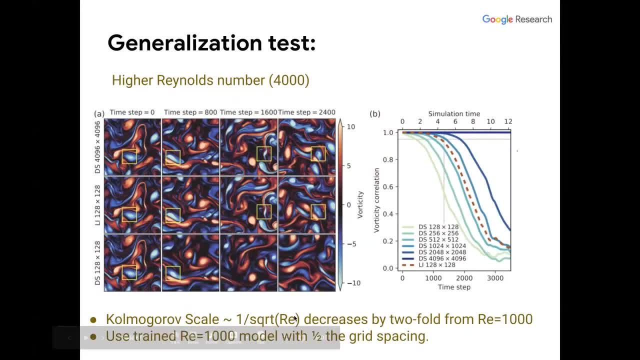 So what that means is is that if you jump from Reynolds number 1000,- which is where I, where we train the previous models- to Reynolds number 4000,, then that corresponds to a factor of two decrease in the scale in the comagraph scale. 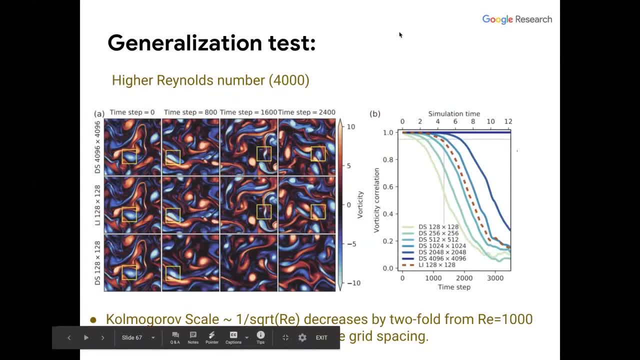 So what we did was to take the model that we trained- Reynolds number 1000, and we cut the grid spacing by a factor of two. We used exactly the same model other than that, And we then applied it directly to Reynolds number 4000.. 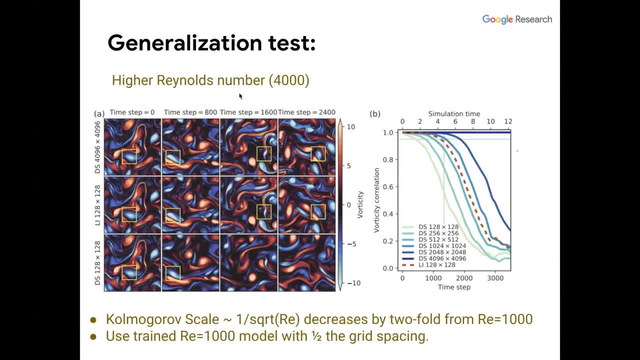 And again you can see the comparison between the DNS and the learned interpolation. You'll notice that the grids are bigger because we needed to to maintain the same accuracy in this from the previous. But again, the learned interpolation massively outperforms the baseline and and leads to something like eight X upscaling. um of the thing. 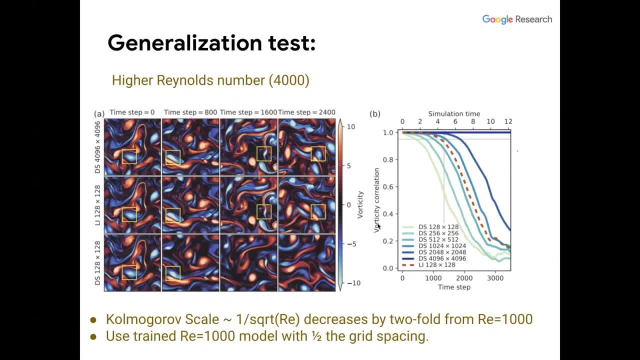 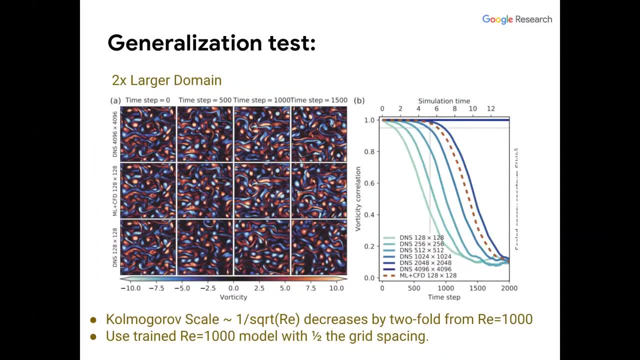 And so, um, Like I said, this wasn't- we didn't make any effort to actually train this for Reynolds number scaling, but this, I think, demonstrates the number scaling as possible. And finally, this is a similar result on a larger domain that I won't belabor. 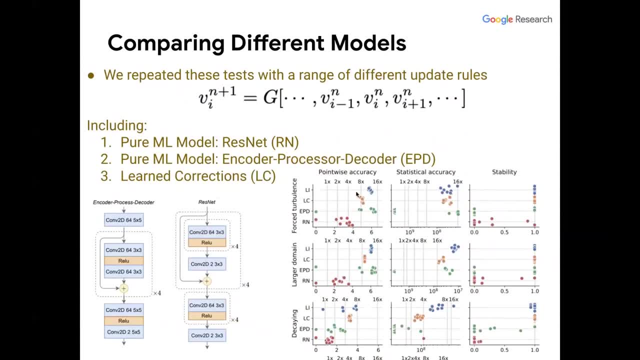 So, um, and this will be my last idea, and then I will stop. I'm sorry, I'm going over. So we were very interested in doing this and comparing as many different models to each other as we could, So we took the model. Remember, I told you there were pure models. 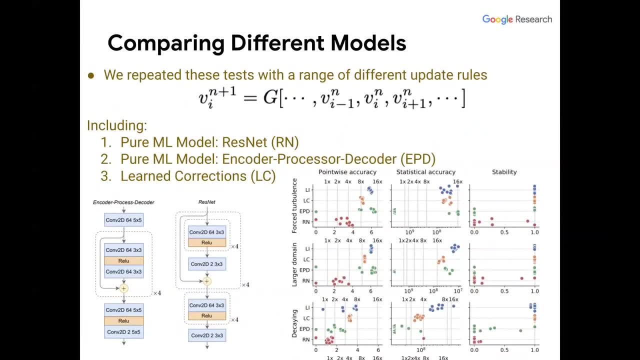 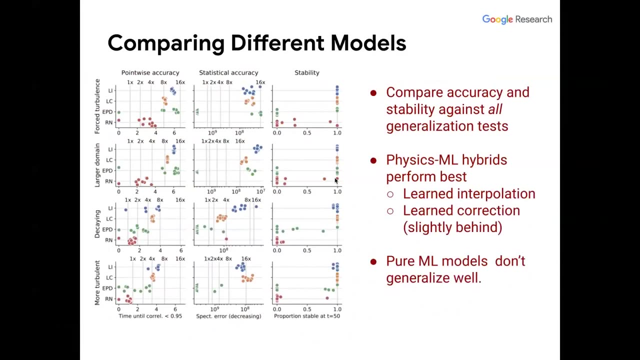 There were learned correction models and we basically competed them All on these different test sets: force turbulence, larger domain decaying turbulence, higher Reynolds numbers with different accuracy metrics, point wise, accurate statistical accuracy, stability- and I have a bigger version of the slide on this talk And I don't. there's a lot of stuff here. 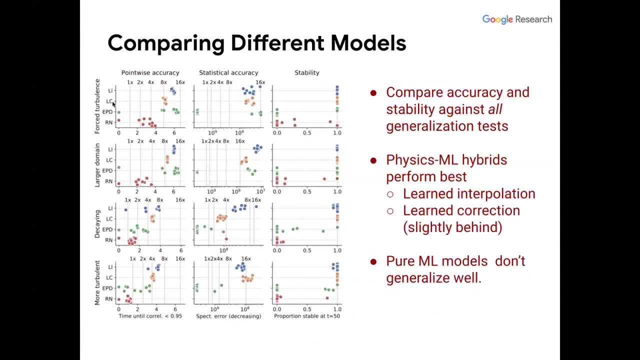 Li is learned interpretation, LC is learned, correction, and this is, this is an encoder decoder architecture. These 2 are pure models: resonance and encoder decoder up. And if you just look quickly at this and these different dots are are different runs, different trained models for each of them and essentially what you see broadly. 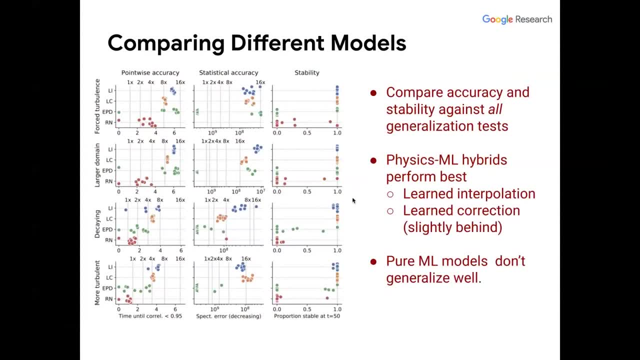 when you look over these spots- and I don't have time to go through this in as much detail as it deserves- is that the physics of all hybrids perform the best. they basically are more accurate. They are more generalizable. You'll notice that like 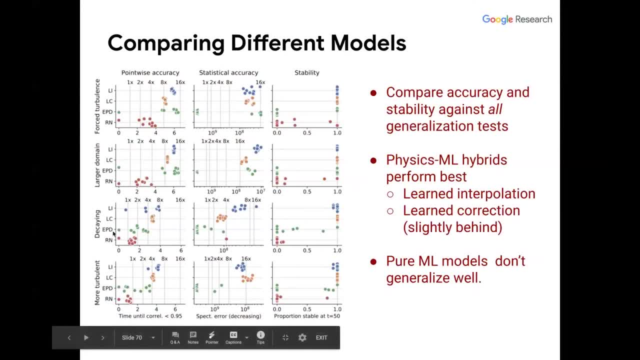 for example, on the decaying turbulence test set, the pure models really don't do very well. They've never seen it before. on the higher Reynolds number they do even worse. They've never seen it before. They simply can't keep up. Whereas because we've built in both learned interpolations and learn corrections, the structure of the Navier-Stokes equations into the solver, it appears to be much more generalizable. 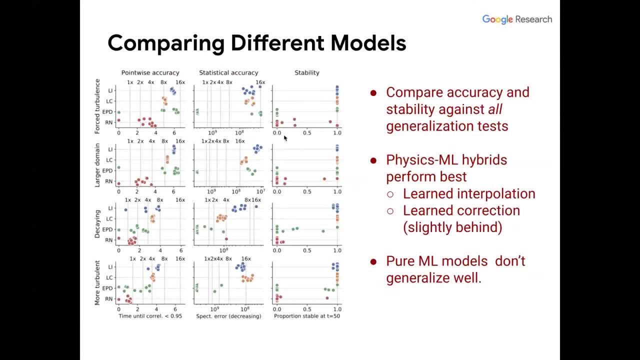 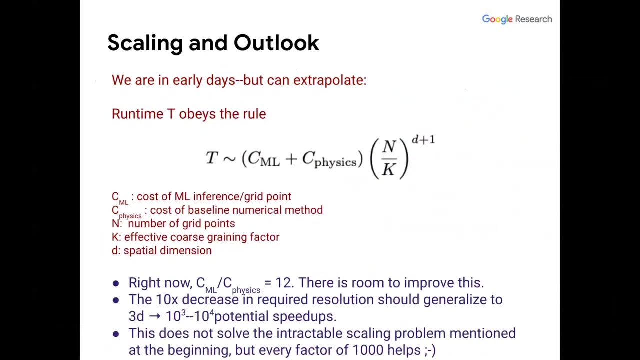 So the learned interpolation basically sort of has the highest performance on these test sets, but the learn correction is only slightly behind and in many ways is a simpler model. So, and finally, we did this directly on large eddy simulation showing similar results. I know I'm out of time. What I want to say is- and this will be my last slide, I'm really sorry. 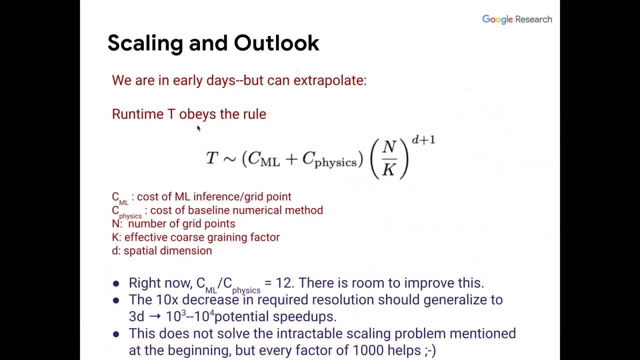 I Organize this. this was not a 30 minute talk, so I just so. we're in the early days of this, but from where we are now it seems reasonable to extrapolate. So the run time basically. So let's capital TV the run time, let and be the number of grid points, but K be the effective course grading factor that you're allowed to get away with, to to solve with a given accuracy. 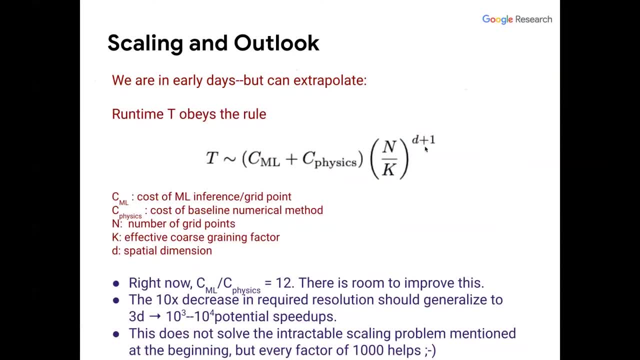 And this, of course, is raised to the D plus 1st method for the power for the type of explicit method that I've been describing. So there's see, physics is the cost of the, physics Solver is the cost of the, and you could ask how much cost savings could you get out of this. So right now, as of today, at least in our hands, the ratio of the cost, the physics cost, is 12.. we believe there's substantial room to improve this. 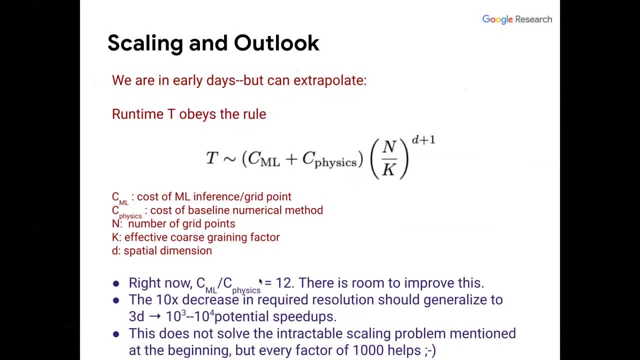 We have not tried, but but that at least gives an initial thing. So the 10 X decrease that we find in required resolution, we believe, although all we know is what I told you, but we believe this is probably fundamental, That is. 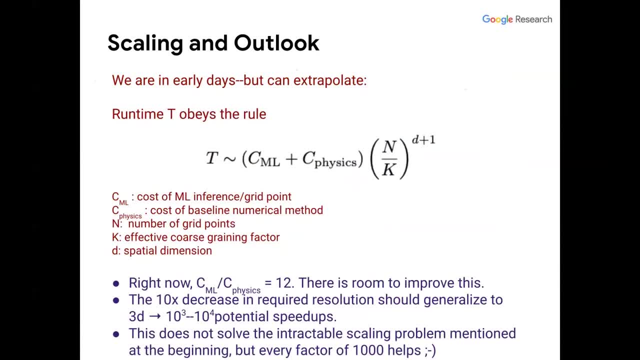 it's unlikely you're going to beat this and maintain point wise accuracy. This must be roughly the upscaling that you can do and still know that there's an Eddie inside of your box to try to interpolate to. So if you were to basically extrapolate this 10 X to 3 D, then this has just using all of these numbers and that would suggest that there's a sort of 1000 to 10,000 times potential speed up. 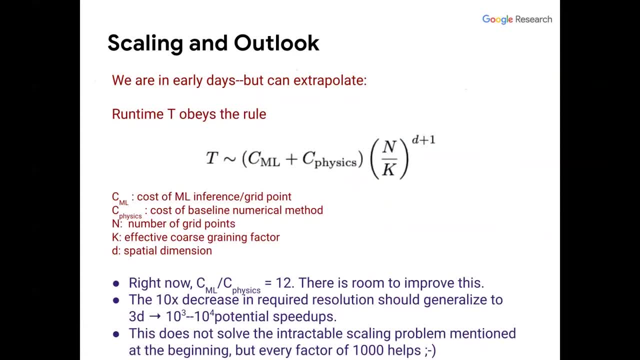 That is, in this type of algorithm. Now, this, of course, does not solve the intractable scaling problem that I mentioned at the beginning of the presentation, So that I mentioned at the beginning of this talk, which is, of course, 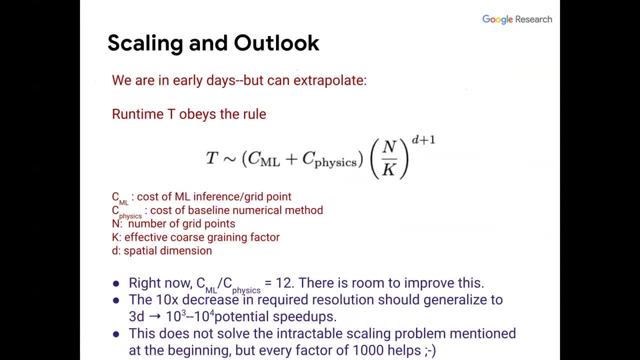 core for the climate community. I mean, this is not going to do a long way between resolving the flow and 100 kilometer matches, But what I would say is that every factor of 1000 helps and, moreover, this is only a particular formulation of how you could have frame these models. 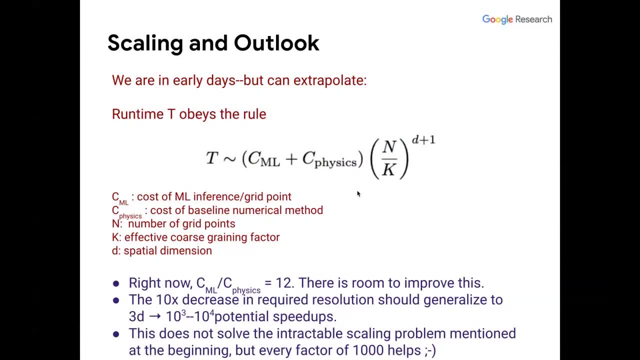 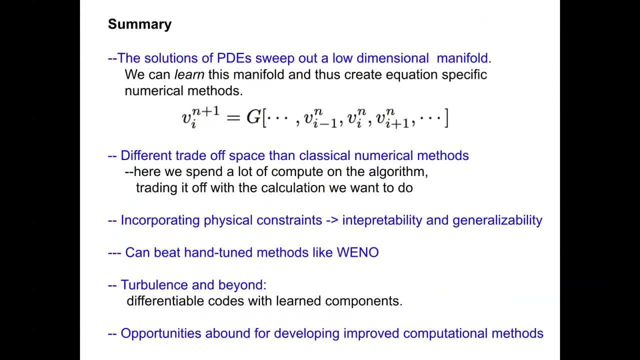 And I think that there's just a ton of other things. you could try and make things better. So let me stop there. I appreciate your attention. I'm sorry I went over. Thank you, So we'll take the next 20 minutes for Q and a. if you have any questions, feel free to type in the chat box or you can use your raise your hand button next to your name and you can ask it out loud. So with that, I do see a couple of questions in the chat box. 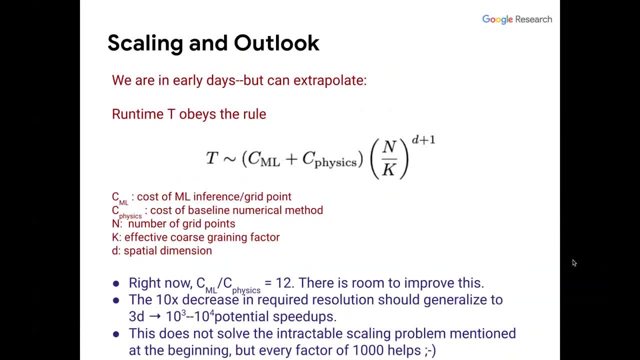 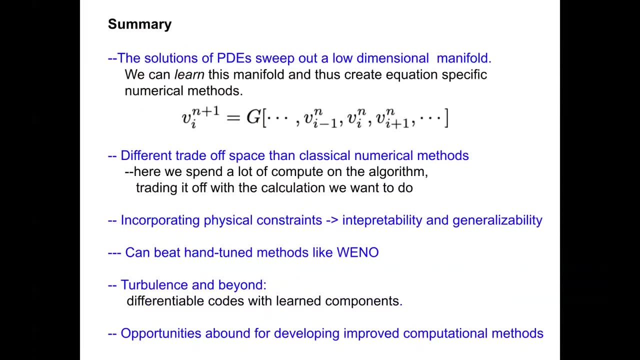 Let's start with the one by Paul Ulrich. He says great talk, Thanks. Generally, grid codes are memory bounded instead of compute bounded. Were these problems small enough to fit entirely on the GPU? If so, how do you expect wall clock time to be affected? 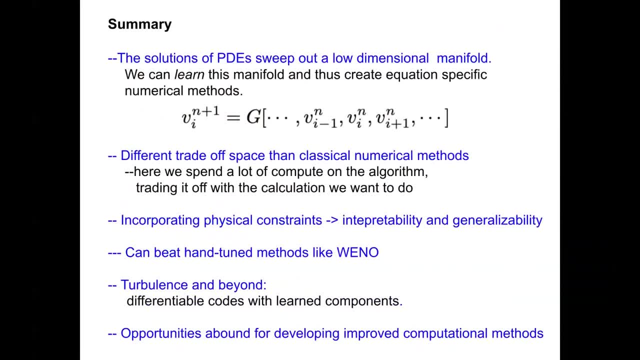 And the problem can't fit. Yeah, this is an excellent question. So so these we everything that was in this we did on single TPUs, but but clearly, in order to go especially to 3D, right, that is no longer one needs distributed computing. 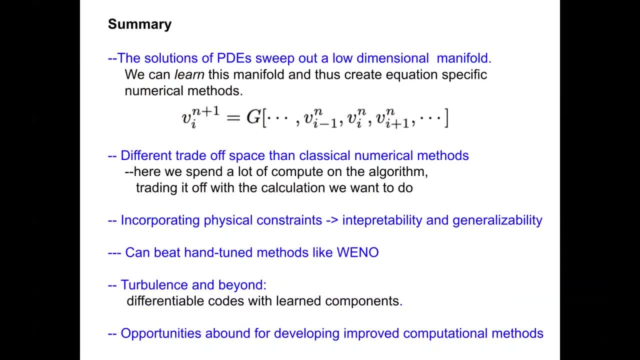 And we're currently working on that, But I agree that that's a challenge. I mean the. the 1 thing to say is that we that you know the machine learning overhead. maybe this is a, maybe this is a useful comment, or 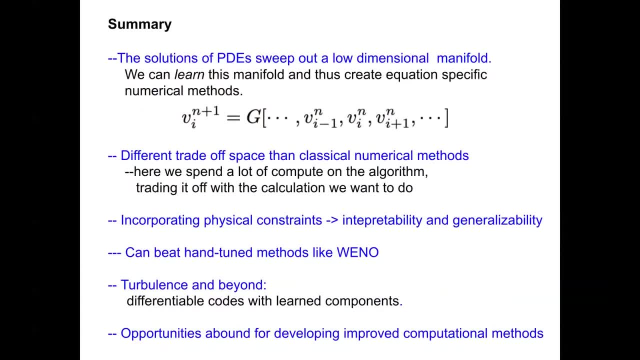 Is that so? there is, of course, a machine learning overhead for doing these computations, but since much of the time, in sort of typical physics solvers, is writing the numbers in and out of memory, then we're, you know, the, the, the utilization of the, of the of the course as well. 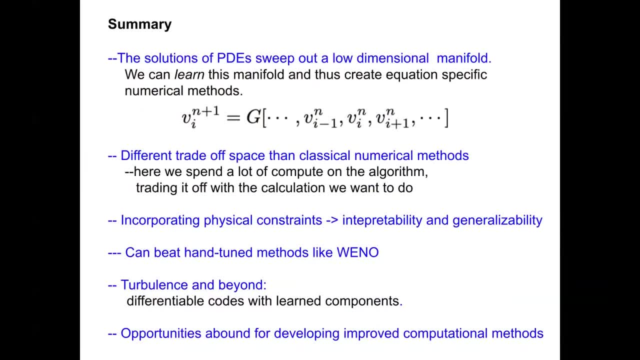 And we're basically using the extra overhead to accelerate, to basically do the, to do a bunch of the ML for free. So, but, but, but for sure this needs to be moved to distributed computations in order for it to for it. 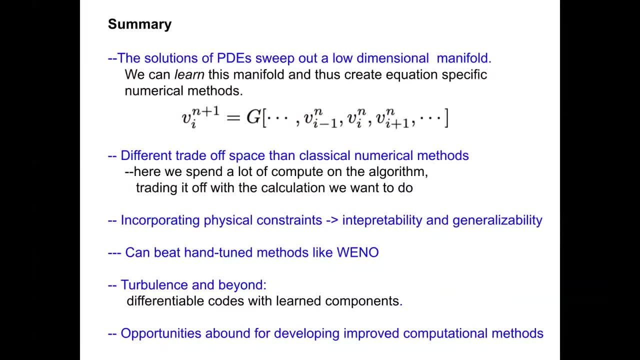 Well, the That's a critical next step. Thank you. Let's take a question from the audience before we jump back into the chat. I see that has a question. want to go ahead and ask it? Sure, Thank you. Thank you for the talk. So I have a related question. 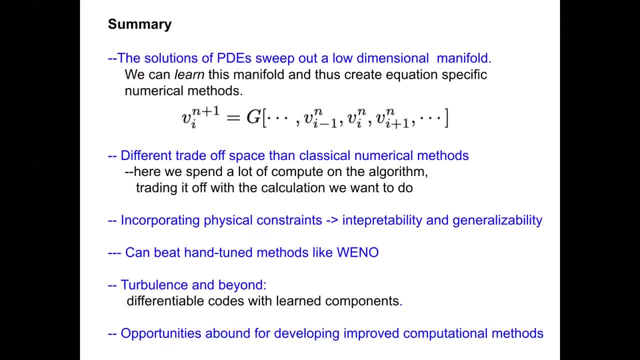 So do you think machine learning can learn how to solve arbitrary linear system? I give you a. this is for different ways. I in another way of saying, learn to Find a inverse. you know I give you a lot of a and it's inverse. Can you give a new a? can you find this inverse? 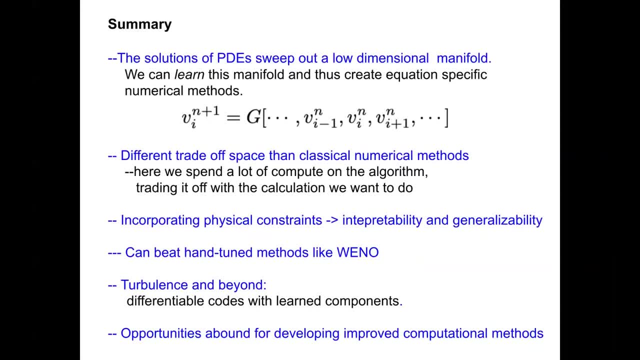 Yeah, that's 1 of those deceptively simple questions. That's I don't know. I mean that's my answer. That sounds really hard to me, though. I mean you know this. I mean that's like you know. that sounds really hard to me for any a right. That's hard. So we're. what we're banking on here in the work that I've described to you is the fact that 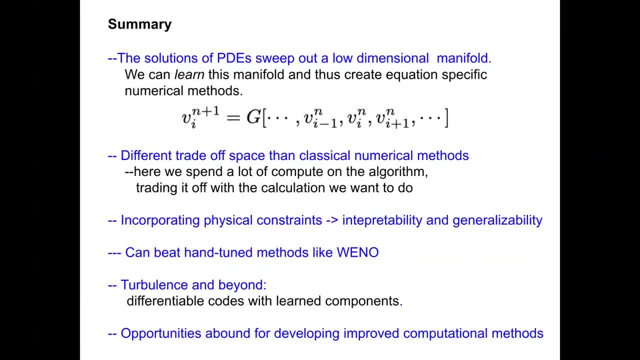 Is the fact that the local behavior of solutions to have, You know, are lower dimensional than those of the interpolation schemes that we typically use. So we are basically learning local properties and that actually you could imagine parameterizing, You know, once you get to solve any large problem with machine learning. it makes me, putting on my applied mathematician hat, Very nervous, Like I sort of feel like. 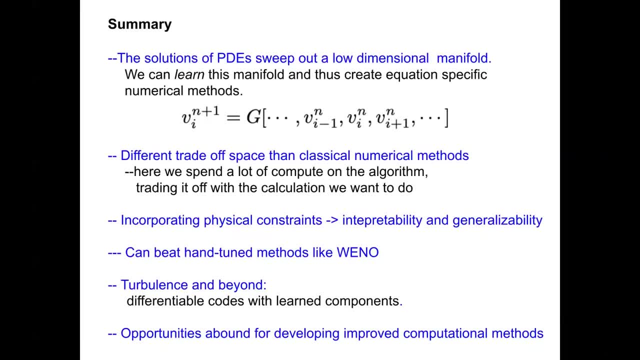 We're not asking. I mean, this is we're asking a lot in some sense, but we're also Asking a lot in a very particular way, where there's hope. I'm not sure that's. I didn't answer your question because I have no idea, but 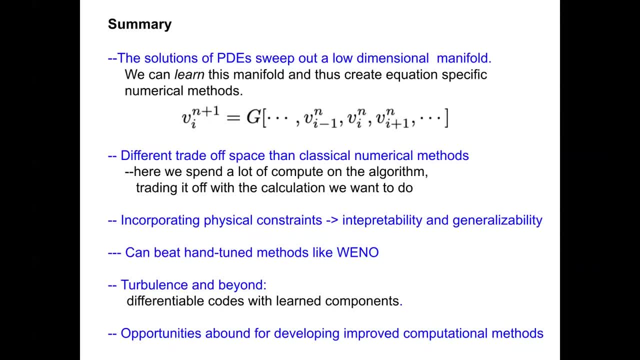 Yeah, but when the coefficient that changing right initial, right inside initials are changing, it's like so in different X you could be no, but it's. but it's doing it in the context of a particular equation. So remember we're training these things by looking at long rollouts of the solutions of, for example, 2 D, turbulence. 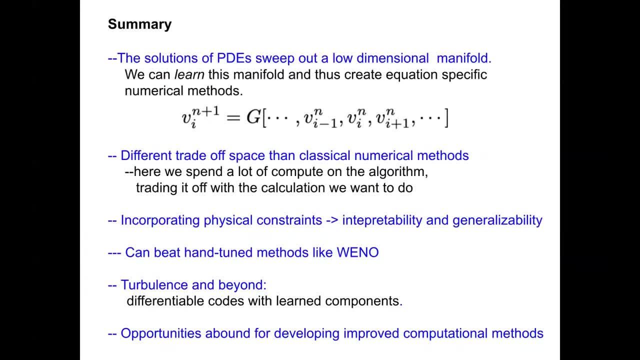 At a particular Reynolds number, And so what we're banking on is that the local behavior of those- although it is changing, you're right, but that there are patterns and that those patterns can be. So it's it and what we're. I mean this sort of gets back to what I was saying at the beginning, that the solution, the dimension of the solution, manifold, is not as large as we're. 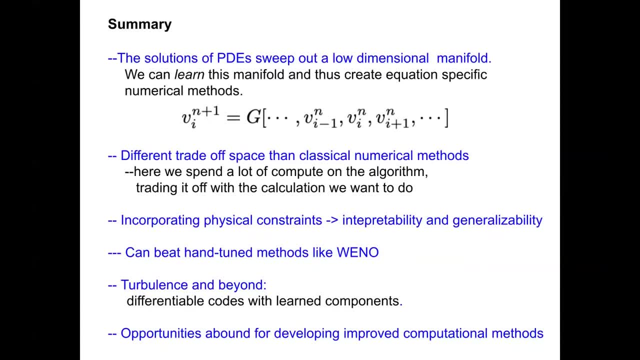 Telling our codes it is, and if we can learn those patterns, then we can Tame them somewhat, and that's what we're trying to do. So I think it's actually a simpler problem than the one that you post What we're doing. we can talk about this more offline, but I that's what I think. 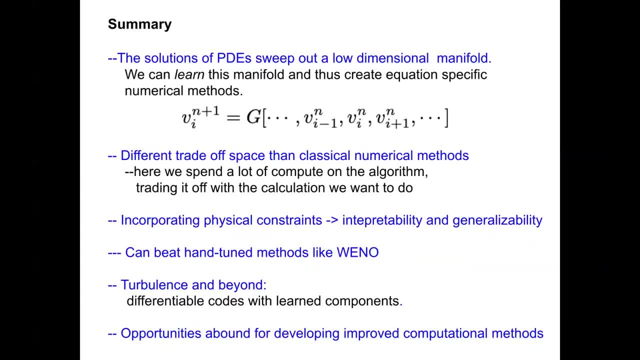 Thank you. All right, a question from Drew. we get to. it's kind of long, So he says this is mind blowing work. Could you, Could you comment what might happen on level 4 general general's liability test? There are, these are tests when some new dynamics 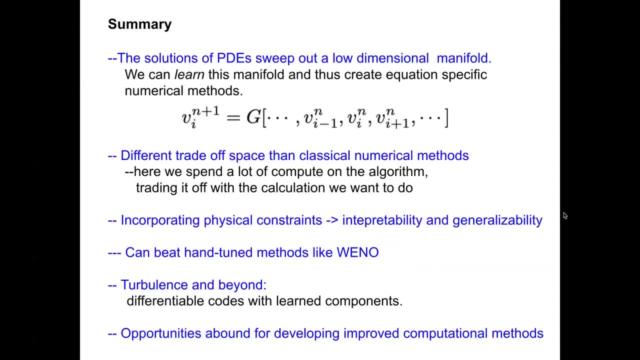 Might come in with change And re or forcing. I am thinking of geophysical fluid dynamic models where some instabilities are not present under some forcing conditions. This is different from 2d, 3d turbulence, which is more of a cascade process. Do you have plans to go in that direction? We're very interested in going that direction And if any of you are interested, we'd love to talk to you about it. That's 1 statement. 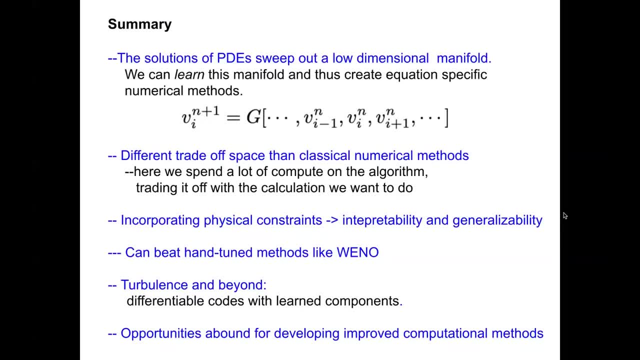 I, I, I agree that this is irrelevant. This is a very relevant question. I don't really have anything substantive to say about it beyond what has been said so far. Sorry, I know That's a non answer. I mean, you know, look, if there are patterns, we should be able to parameterize them. I mean, I guess that's what I would, would say, Right. 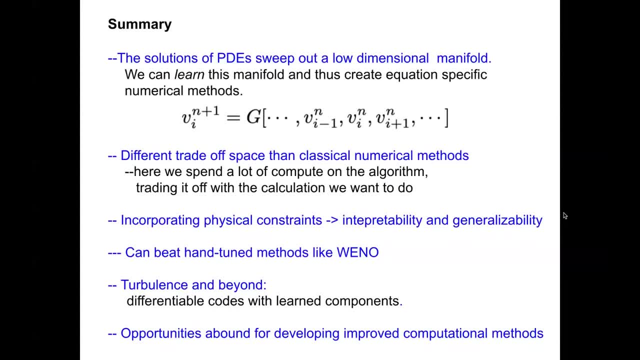 If they're, if there are patterns, we should be able to parameterize. and local, if they're local patterns, we should be able to print. and you know global patterns that are made out of local patterns. That sounds good, You know. 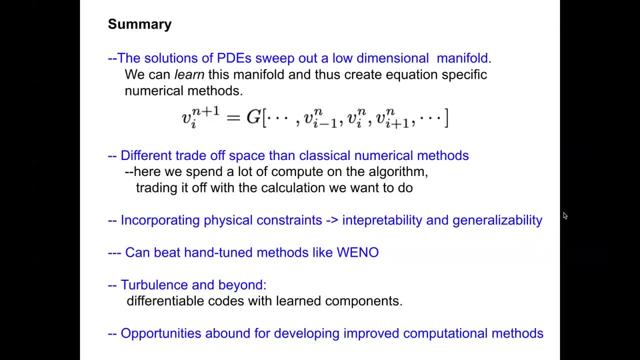 Um, so I see a question by Mike Pritchard. Do you want to go ahead? and? and you yourself? Hey, sure Can you hear me. Yep, Thanks, Uh, yeah, I was wondering. you know I can't. I can't resist thinking about trying to take this to the climate modeling limit. 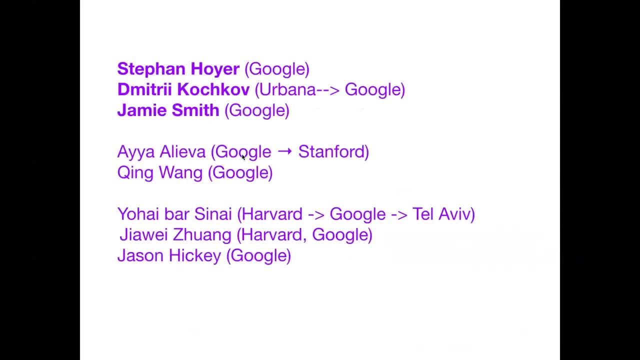 Um, there are several things seem overwhelming. You know it's no longer 1 equation but a terrible mess of interacting your questions and primary stations. but especially concerned about the rollout issue- I think you commented that you needed like. I think you commented that you needed like. 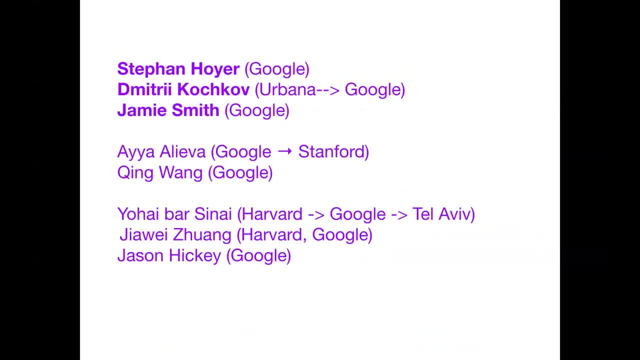 to set for statistical stability in the spectra, like some ten thousands of time steps or something for this experiment. but can you elaborate on how that number arises or whether, yeah, is there a principal way to think about the, the amount of forward integration that needs to be coupled with? 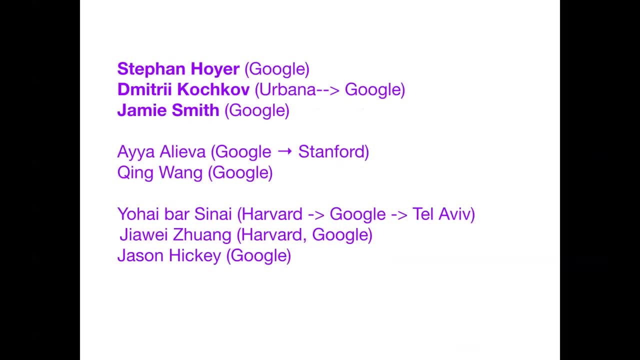 the optimizer of the full model in order to. we didn't optimize it over that much. so, to be clear with, the optimization was over much shorter time steps right. that was. that was the number that was used for evaluation to check for stability in the in the forward algorithm, because you know the 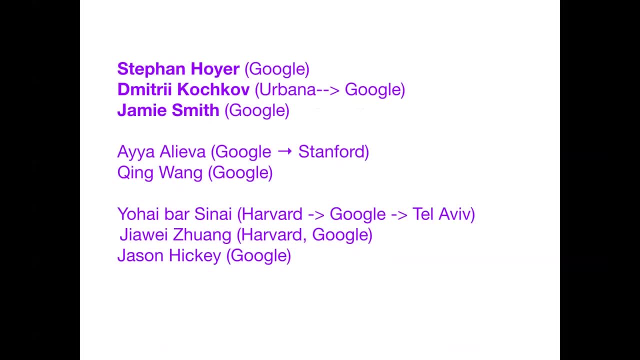 thing to always worry about when you're doing the sort of thing that's here, is that the model somehow blows up because something happens as you're rolling it out that it hasn't seen, and the neural network goes nuts, basically, and then you know you end up with something which is 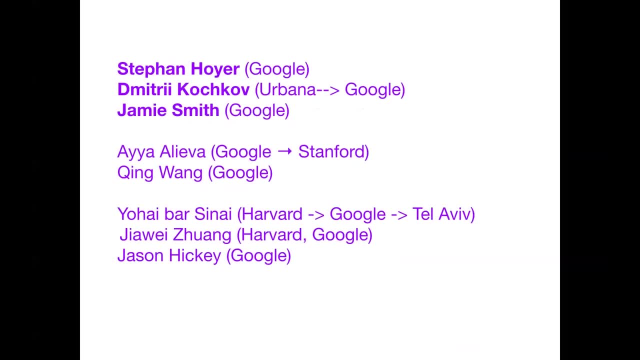 completely ridiculous. i mean, of course this happens in standard numerical analysis too, but in standard numerical analysis we have well-known methods to assess for stability locally. that will give you a good sense of whether or not the rollouts will happen for a long time, and no such theory exists here. so i guess that's my main. so i think i don't. i'm sorry. 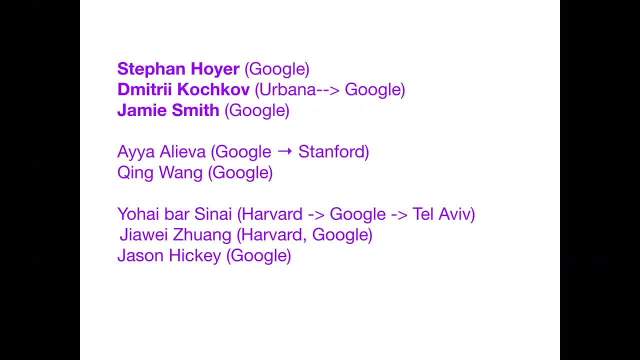 this is. you guys are asking really good questions which i don't have good answers to. you know, there, we're missing a lot of theory here right now and so, um, you know, i would have thought that rolling out, if you've got the thing, that rolls out over tens of thousands of time steps and it's stable. 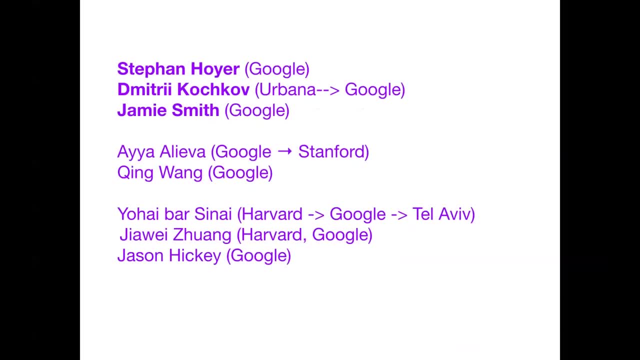 with respect to the spectra, that you're likely going to be okay, basically, but there's no theorem that states that in this case- and i the suspicion is is that purely empirically, as we get experience with this type of methods, you know, if it did blow up then what you would go do is go back and retrain it a bit. 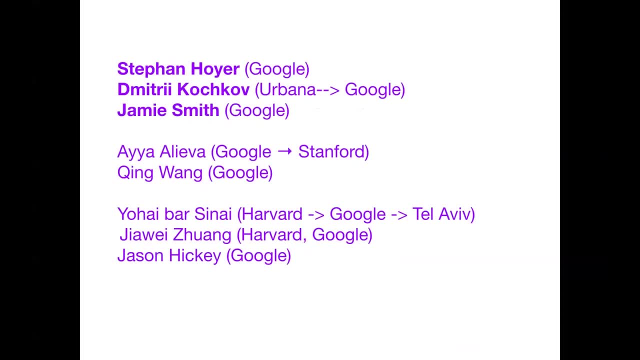 and sort of make it better. and so i, you know, one suspicion is is that you know this is sort of good enough in the sense that if something goes wrong then at least you probably can fix it. but we are, and i mean, i think it's just the inherent problem in doing things this way, you know, with something. 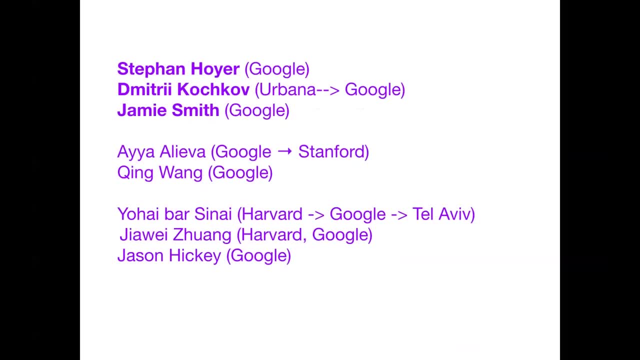 that's machine learned, as opposed to something that's like related by calculus to the original equations, that, um, that we don't have stability constraints yet, but but it's the wild west. i was telling somebody the other day: this is like you know, it's sort of like, uh you. 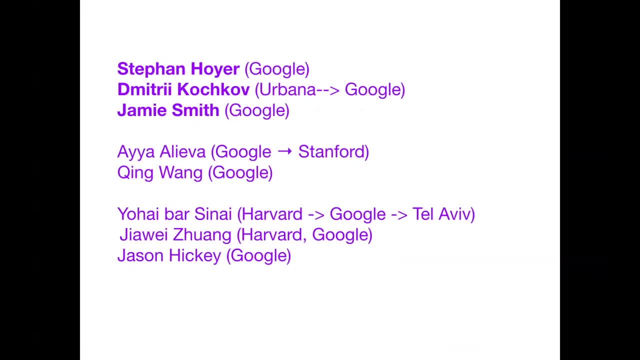 know they're used. in the 19th century there were steam engines, right, and everyone was building their own steam engine and, um, you know, you just wanted whatever steam engine that drove your car or your train or whatever. and but then carno came along and he gave you know the principles of steam. 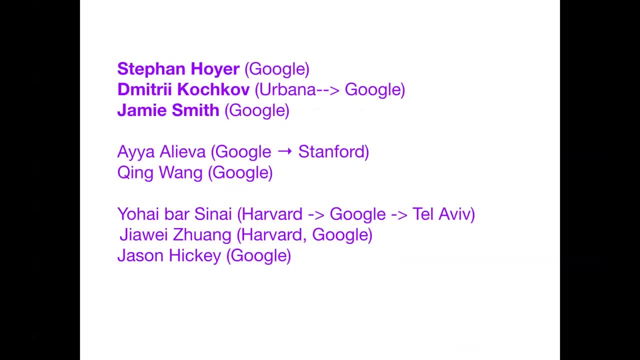 engines, you know, when he was quite young actually, and we sort of need that here. so but this is just an effort to sort of figure out how to do that, and i think it's a good question, i think it's a good show, it's possible. sorry, i know i didn't answer your question, mike, so i just, i think, i just 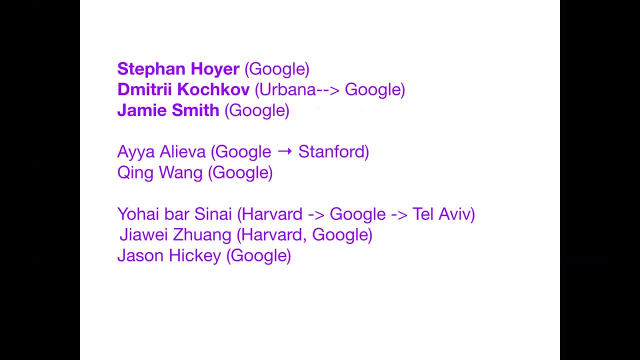 misunderstood one thing: the training was local in time. yeah, the training is local in time. okay, thank you all. right, there are a few questions in the chat um. so zhao wu has two questions, so we'll start with the first one. it seems like the como grow flow does not have a converged solution with 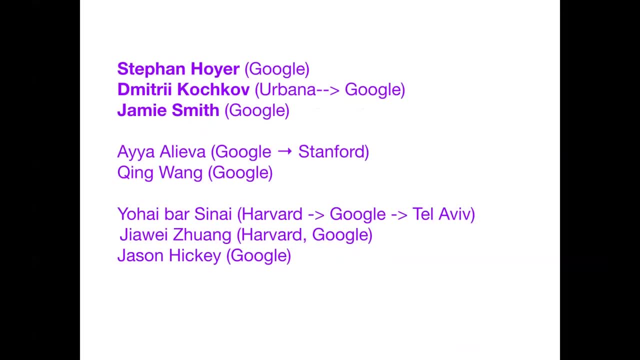 the increase of the resolution. my question is: did you try to use this machine learning method to solve a flow with known converged solution and see if your machine learning method can solve? a machine learning method can get the same statistic. i'm not sure what he means by that. why, why does? 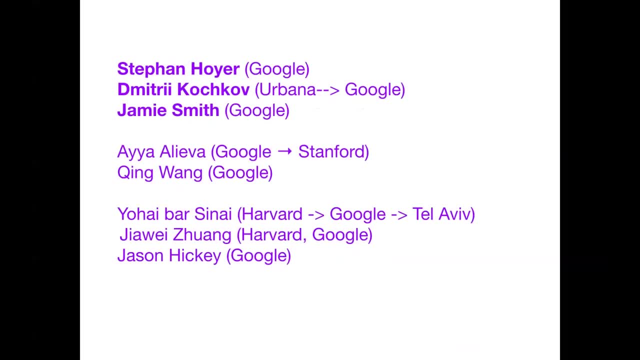 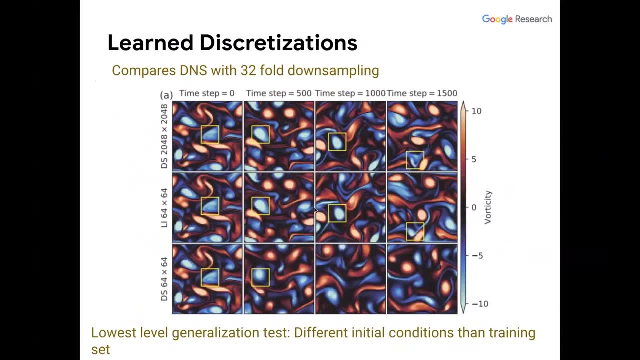 it not have a converged solution. so i would have argued that on these you know flows- i mean here let's just take the initial one- that the 2048 is converged, that this actually, if you cut the resolution, this is actually way overkill for the structures that are forming at this. reynolds. 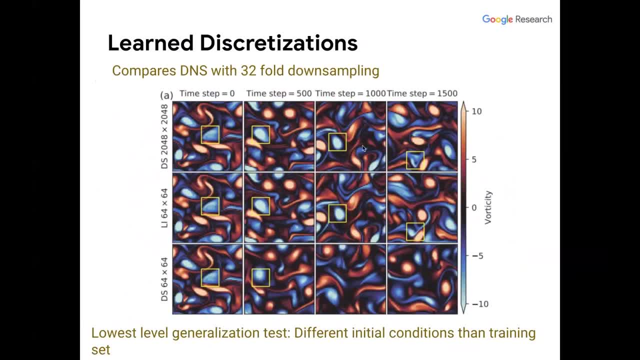 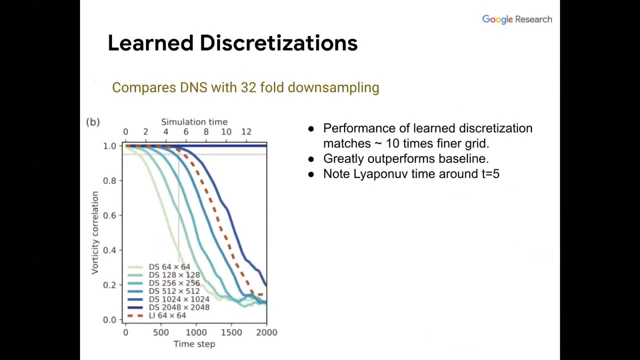 number. if you caught the resolution, it is converged. so i guess i don't understand, um, so i'm just going to go to the next slide. okay, so if you look at the resolution, when you go to uh, 2000 by 2000, the, the statistics, the, the profiles there, and even so, what's the profile? 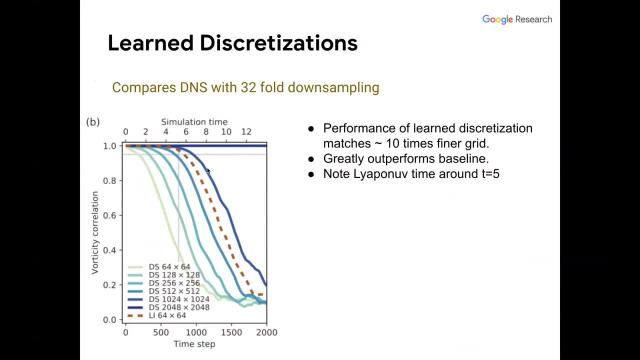 looks like when you keep increasing the resolution. okay, good, so let me let me just explain this. this is good. thank you for bringing this up. so this is the vorticity correlation. so this is basically right. the correlation, the average correlation of the vorticity field over time. this 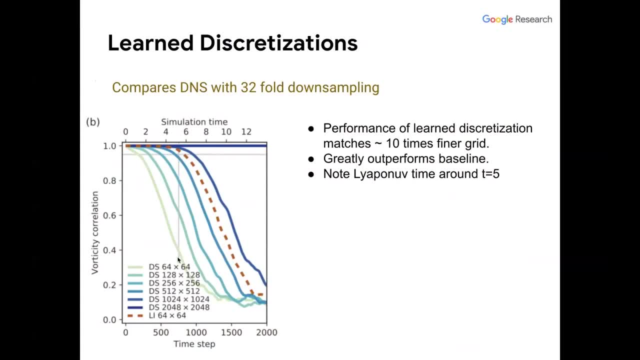 line right here you see this gray line. this is the lyapunov time of the flow which we've computed separately. so when you cut the resolution, you wouldn't expect, you would only expect the trajectories to agree up to the lyapunov time. and indeed, if you look at the 1024 rollout which is 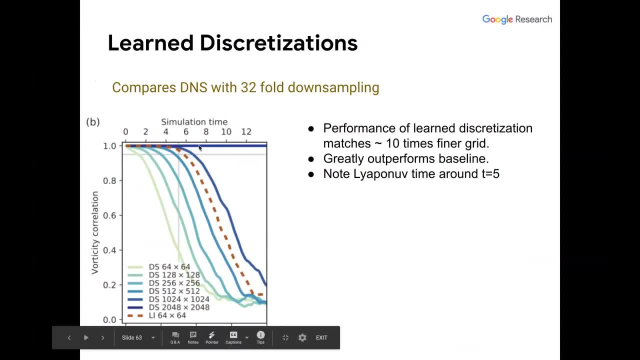 this. it agrees with the um, with the ground. this, this thing is fixed to be one because we're measuring the correlation of it to itself, so it beyond 1024, beyond the lyapunov time. you wouldn't expect it to be one, because we're measuring the correlation of it to itself, so it beyond 1024, beyond the lyapunov time. you wouldn't expect it to. 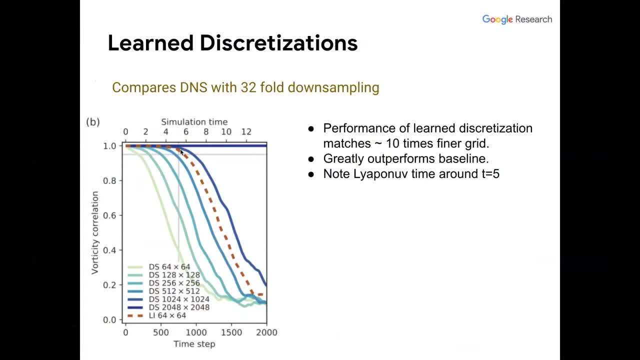 agree, and that's what the one at 1024 does, and that's essentially what the learned interpolation does as well, although slightly worse. so i don't think that this isn't showing lack of convergence. this is just showing that the equations are chaotic. does that make sense? yeah, thank you. 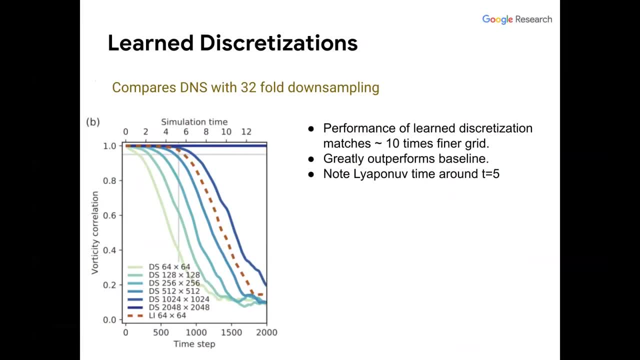 all right, and his second question: zell, do you want to ask your second question? do you want me to read it? okay? um, did you try the 3d flow, for example, the isotropic turbulence, because they have? um, yeah, we're very interested in doing this for 3d flow and this is under. we're working on this, okay. 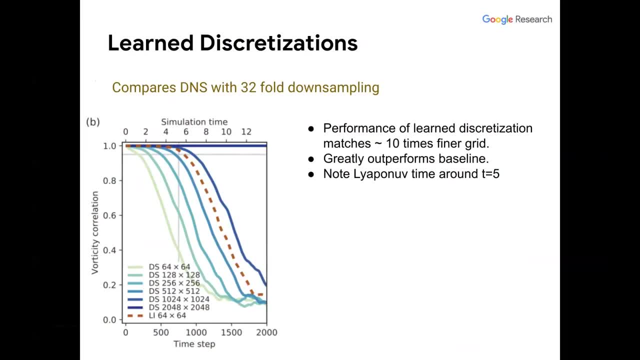 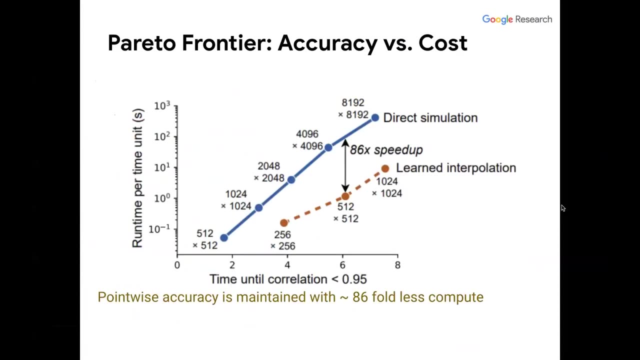 totally agree. without that, then we're not there yet. thank you very much. a question from gavin d: why do you think learned interpolation is slightly better than learned correction, right? okay, that's a good question. so i'm going to give you a hypothesis. i actually noticed a couple of the other people from google are on this, and if any of you guys want to answer, 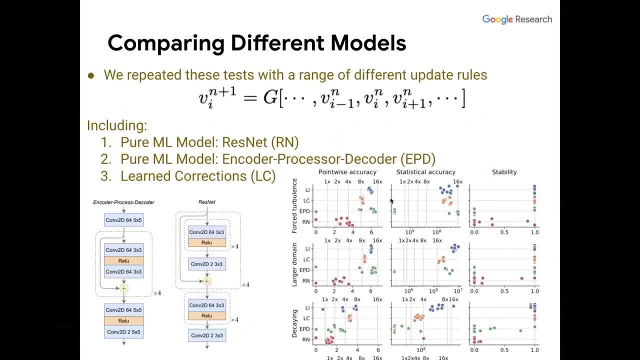 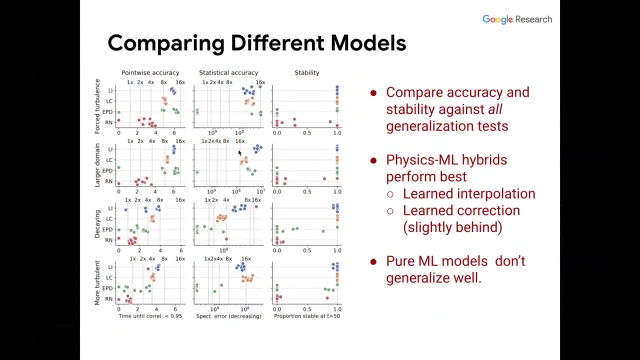 any of this, you please should. but okay, i'll give you um my answer. so i, so i actually the zeroth order answers. i don't know, however, um, but, and that was good, so you're referring to this phenomenon- that learn interpolation is here and learn correction is here. so when we added the correction, remember. 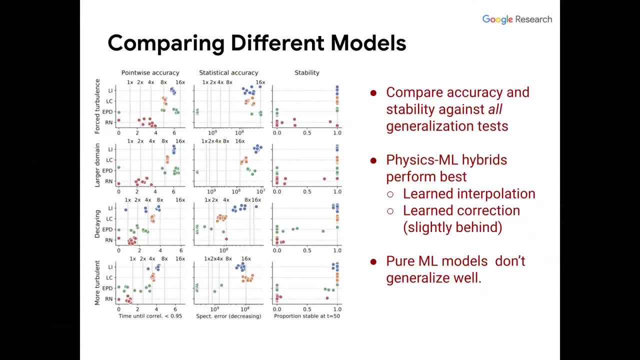 i said we were adding a correction. the way we added the correction is that we literally just added a term we didn't so in in principle right. so there's a. we added a forcing term to the equation. i mean in principle right. any correction term should really be the divergence of 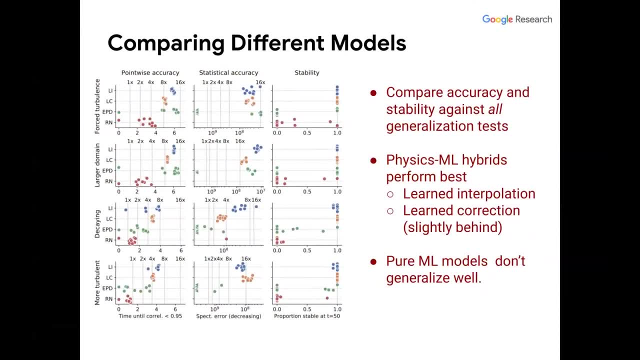 a tensor because you know of conservation momentum, and one hypothesis- which you know this is purely a hypothesis- is that that this gap isn't real actually and that it's simply because we didn't constrain this learn correction to be the divergence of a tensor and thus it doesn't. 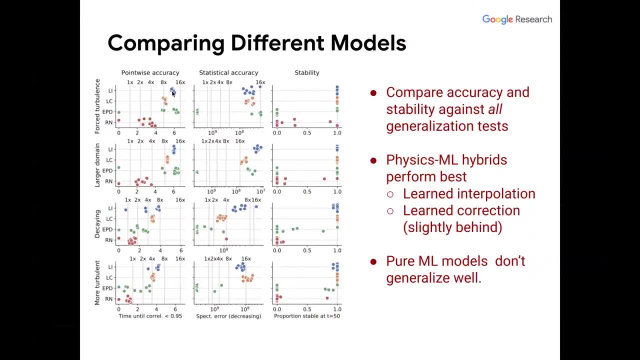 it's not enforced to obey that constraint, which causes it not to be as accurate. so that's a hypothesis. um, whether that's true needs to be tested. just as an amusing aside, we also, of course, tried the following: learn correction: we took it to be the divergence of a tensor viscosity times. 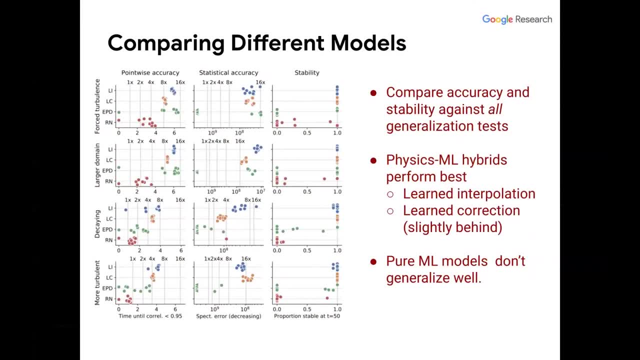 the gradient of velocity, because that's of course what you're supposed to do. we should just train turbulence models right. and that we actually found, at least in our hands, to be worse. um, because it was more. it was more difficult with numerical stability constraints. it had more numerical 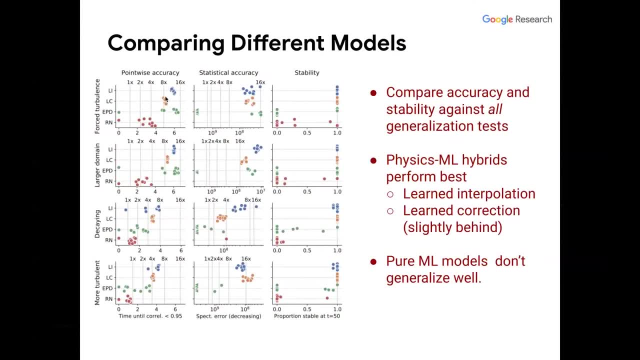 stability problems than this. so, um, but i don't know. that would be my hypothesis, that that this is, that this is a fake, that this really this, these two perform similarly, although we don't know for sure. i mean, i guess, the other thing to say, though, maybe i should just add one more comment. it's: 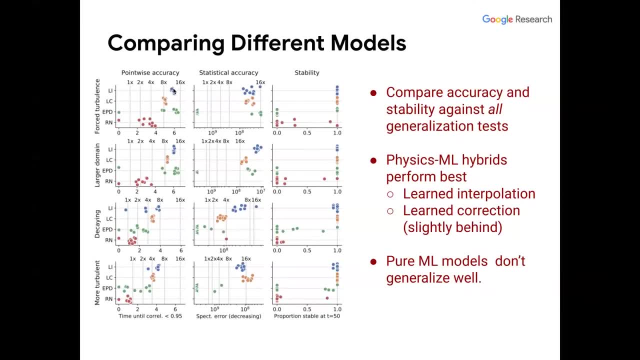 possible that it goes the other way. i suppose, and the way that that argument would look is that you know, when we do an interpolation, we're doing it over some large number of mesh points and, of course, if you look at the effective equation and what we call it numerical analysis, the equation when you 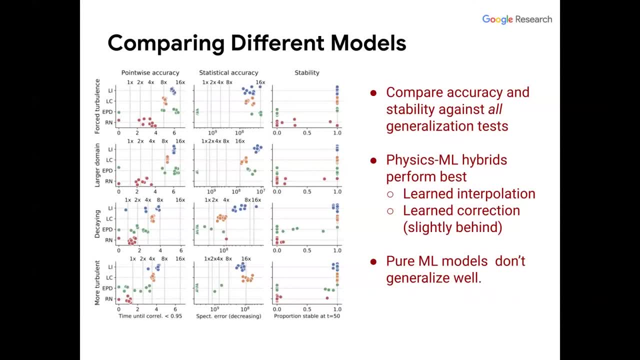 tailor, expand what you have and look at the equation that you're actually solving. the learned Interpolation has more effectively higher-order terms in it than the learned correction does, and it's not inconceivable that that doesn't help. but anyway, we have no idea. 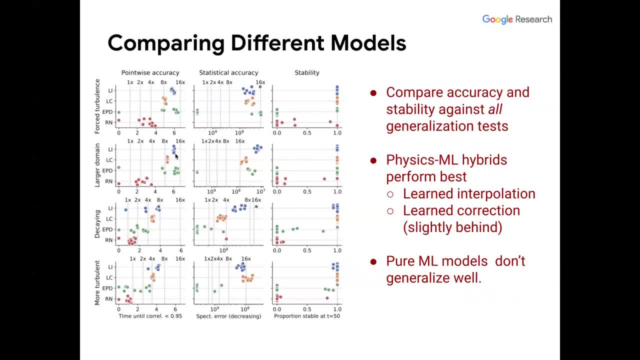 I mean they're pretty close though in performance. They're close enough in performance that you would be pretty happy with either. I think A question from Jack Sheen says: hi, Michael, nice talk If RE numbers go up. another order: do machine learning interpolants have to be trained again? 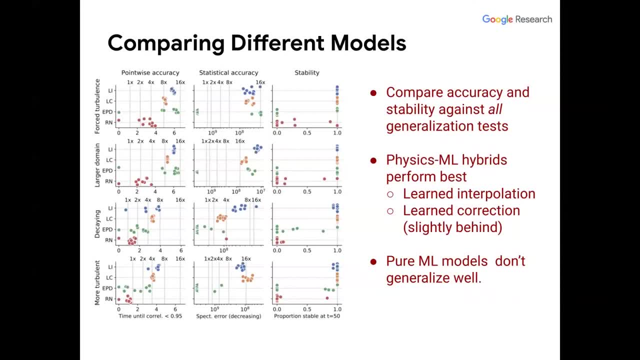 Thanks, That's a good question. We don't know. I mean in principle, I mean we haven't tried it and we don't know, so I'll give you the in principle answer. So in principle, look, if you're in asymptopia, so if you're in the part of the, if Reynolds number is high enough, right that you're actually in the cascade region, then one would hope that one doesn't need to do that. 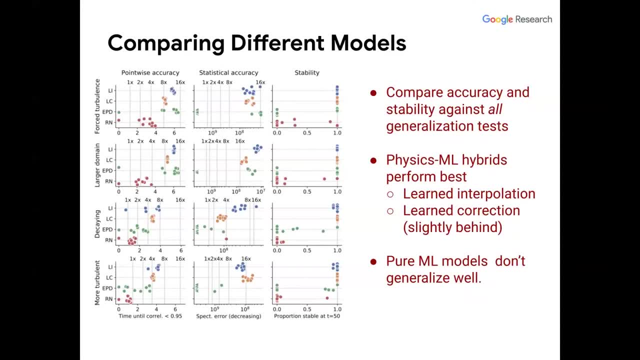 In the same way that we use eddy viscosity models that have parametric functions for the viscosity that you know depend on Reynolds number, in a way that Kolmogorov would have said: You know, and that don't have to be right. It's the same functional form, So that's what one would hope. The 1 thing that makes me slightly nervous here is that we don't have a huge range of scales here. The forcing scale I didn't say, but in the Kolmogorov flow the forcing scale that we use was 1 quarter of the size of the box. 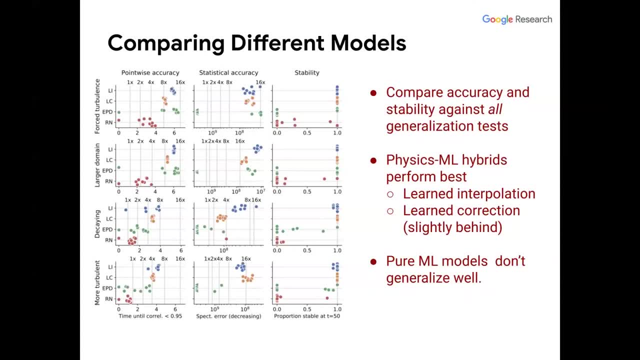 So we basically have from 1 quarter of the size of the box down to 1 over the square of Reynolds. number times the size of the box And that's the. that's the scale, basically, that we're talking about, which is not the best power law scale that any of us have ever seen. 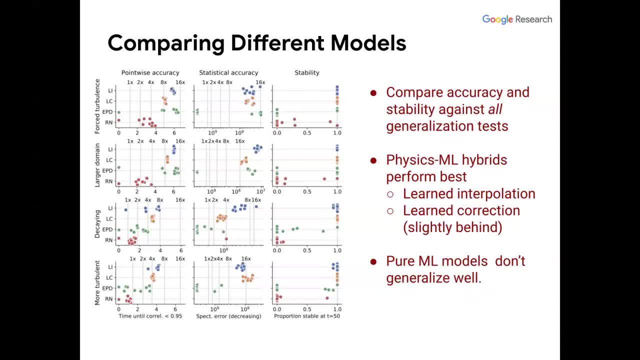 And so you could worry that we're not going to be able to do that, Yeah, In the subtopia yet and ask it's going to have to be. we are trained, but this is something. but in any case, this is an initial step. So 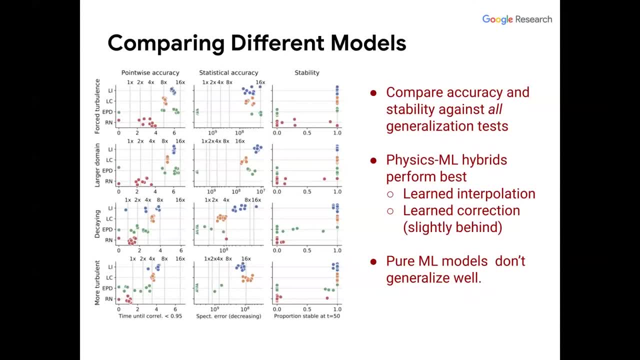 Good question. we have another 5 minutes for questions. Jack says: thank you, Um, so do we have anyone with other questions from Michael? I feel like you've you answered all the questions too quick. Okay, well, that's good. 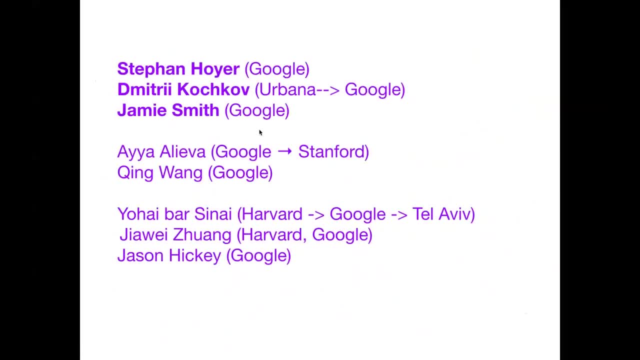 At least I got through it. Well, I just want to thank you all for listening And again I want to sort of acknowledge, you know, especially Stefan and Dima and Jamie, who made this Navier-Stokes thing work, which was a really 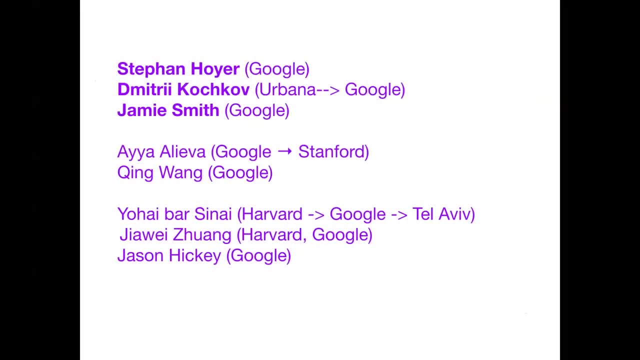 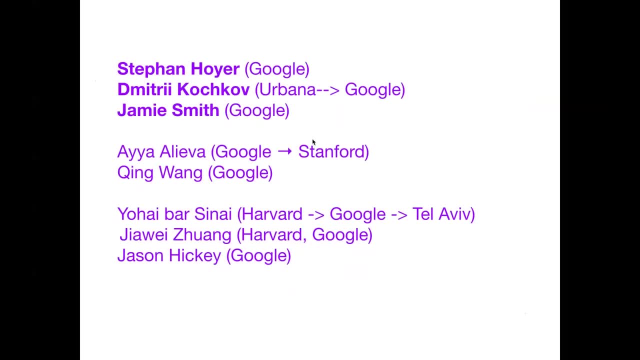 Well, I can't, I can't resist. So can you? can you comment on your outlook on what the most gnarly technical issues are for scaling this up to 3D? Is it the coordination? Is it the coordination across GPUs? 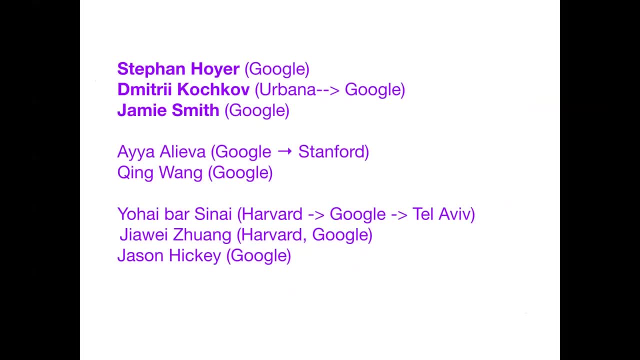 Is it extending the differentiable programming to be parallel, or just curious? Yeah, so it's. it's purely data pipeline issues. It's just that you know the amount of data. you know the scaling is is, so it has to. 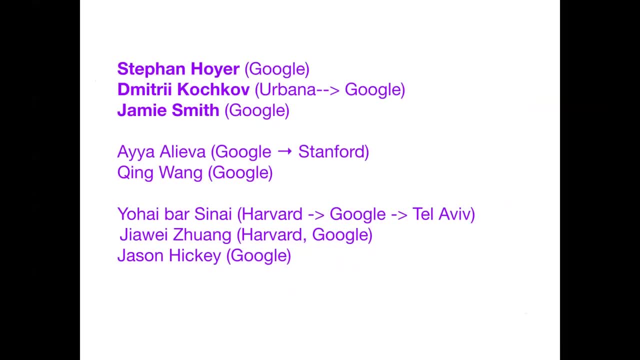 be distributed to do, to do training in 3D. We actually have examples that train on a single TPU in 3D, that at least they start to train. but like the memory issues are, these are, we believe these are solvable engineering. 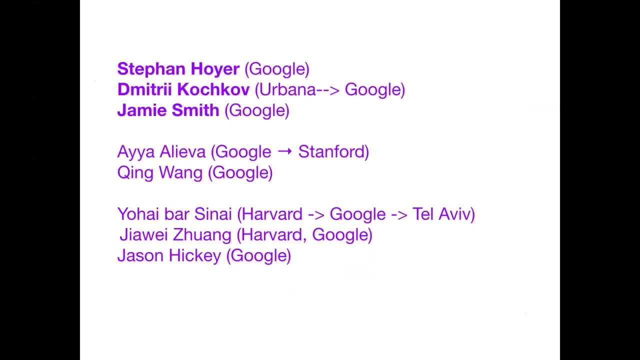 problems, but they're, but it's just, it's not. It, it's not. You know, it's not trivial that the, the code, the, the, the code works in any number of dimensions. It's not just a parameter. 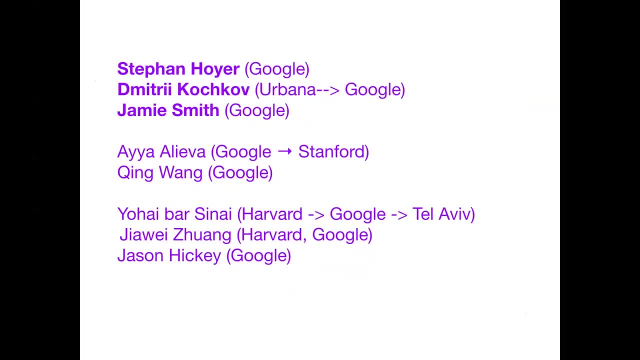 It's not that, it's just the memory. So I guess part of me sometimes daydreams in an industry and in Google that you know they're light years ahead of us in dealing with data sets of gnarly magnitude. but is 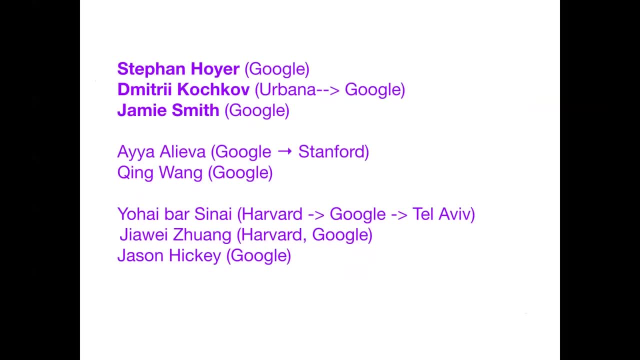 that like a pipe dream, or is there something? Well, there might be, but not. but we're having trouble. Is it like the dimensionality of the industry, Like the dimensionality of the input vectors become unparalleled in industry for these sorts of problems? or 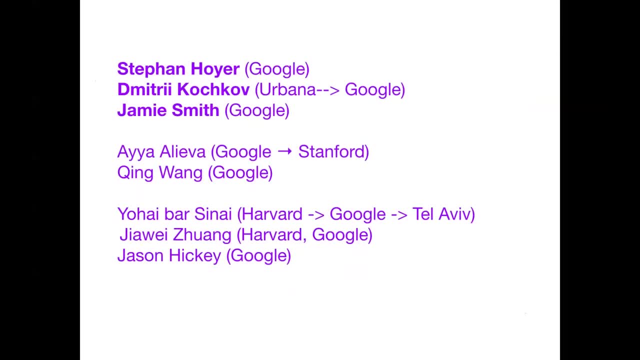 So this is a solvable problem, but it's one that we haven't yet solved. Actually, Stefan is here. Stefan, you should answer this. This is your Michael on us. I mean, I'd say it's, it's not. I think we can't scale up to larger problems. 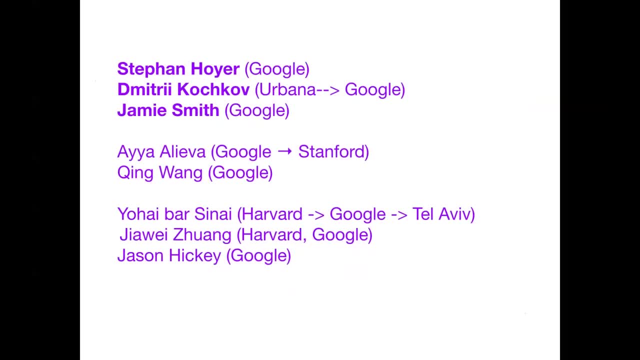 It's just that, like the- this is why we started in 1D- is that the iteration time gets slower and slower If you have 10 times more resources going. 1D problems I can solve, you know, I can solve. 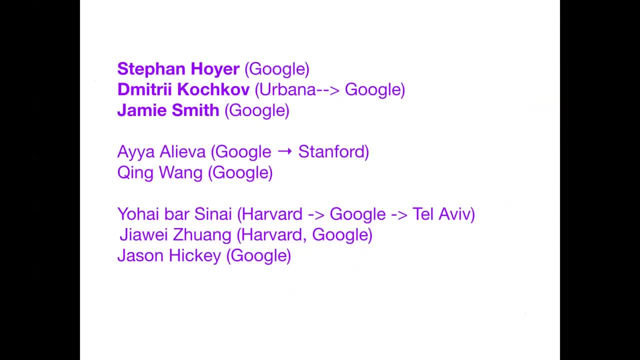 In like minutes. basically, 2D problems take hours. you know, 3D problems probably, you know probably going to take days at that sort of scaling, or you have to scale up to a bunch of machines. So it's just like the duration time, the experimentation time, gets much slower. 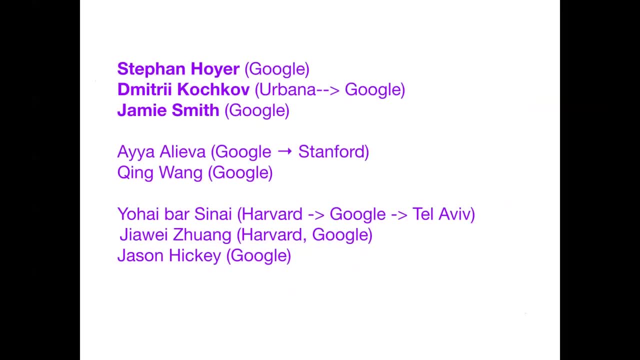 So we wanted to work out the details in in in 1D, 2D first. basically, That makes sense. Thanks, And I think we'll round up the hour with a final question from Drew. He asks: can we play around with the examples, like the one on GitHub you pointed out on? 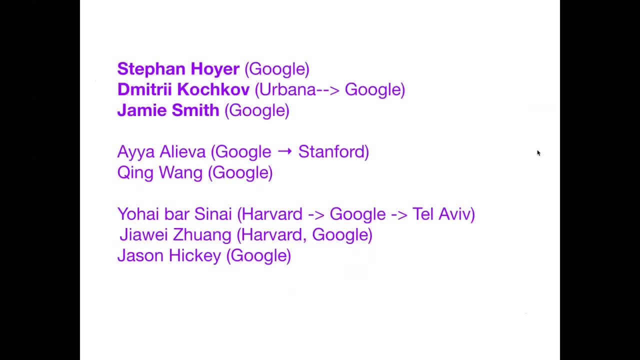 our own computer or do we need some very Google-like or HPC computers? No, you can play with the examples on your own computer. The GitHub link that I pointed out was it's a one-dimensional example and it runs in a co-op, and or you can run it on a Jupyter notebook on your computer. 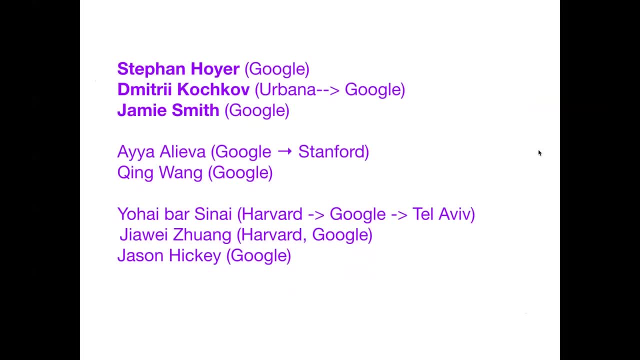 So this doesn't, you can play with this yourself easily. Thank you, So I think we will. Okay, We'll end the webinar here, So thank you so much, Michael, for giving us the talk, and also thank you, Steven, for. 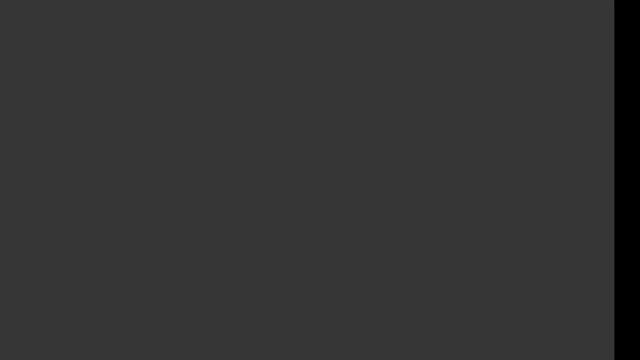 having you know giving your input during the Q&A when we need it. So I will have a recording of your talk available later this week and I will share a link out once it's available. The next data science webinar will be in two weeks. 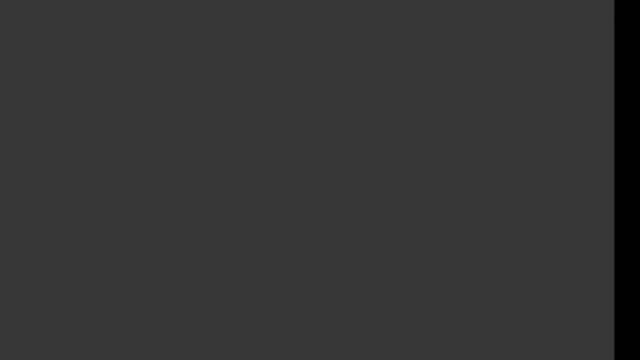 So that's on February 22nd and that will feature Kelly Kochanski. So if any of you guys have any questions, you know, regarding Michael's talk or the data science working group, If you have any questions, feel free to reach out to me. 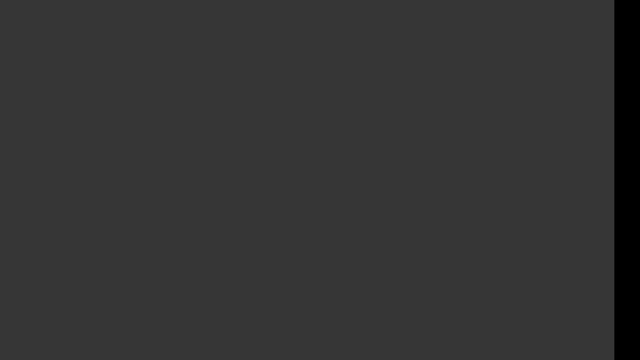 Please feel free to contact me at JZHU at USClyberorg. So once again, thank you so much, Michael, for your talk. Thanks for having us, you guys. 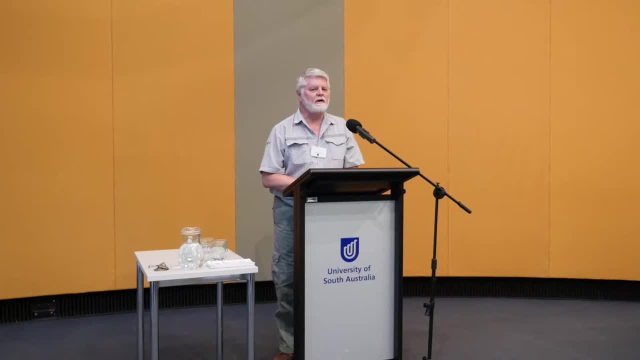 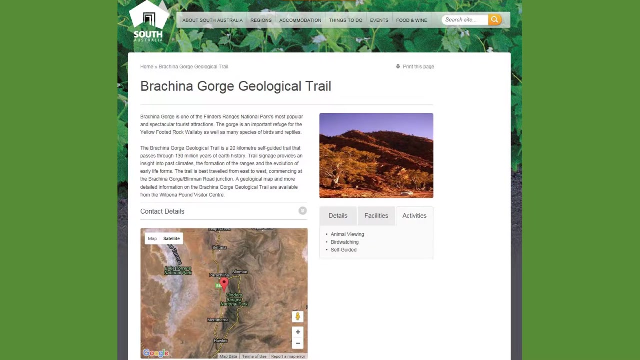 Welcome everybody. My talk is on the opposite end of the scale to the previous speaker. I'm talking about statewide concepts and landscape on a big scale. My first slide talks about the Bratchenor Gorge Geological Trail, which is a 40 kilometre trail cut across the Flinders. 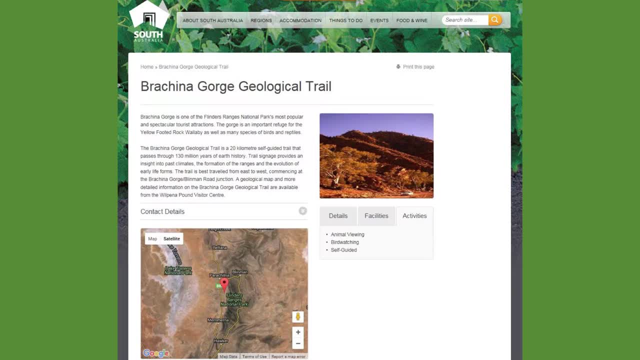 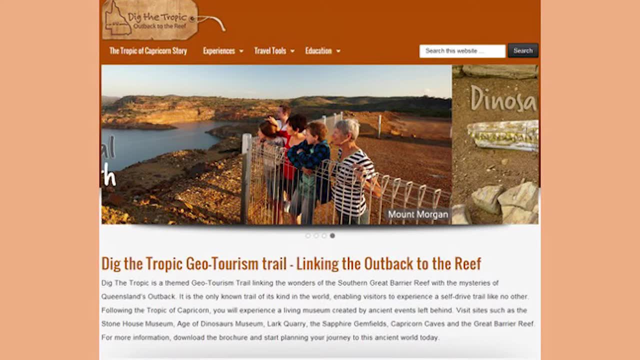 and set up by the Geological Society of South Australia with interpretive signs. But that's not the only trail in Australia. In Queensland, the Dig, the Tropic Geotourism Trail crosses the entire state along the tropic, So it picks up towns, fossil sites, mines. 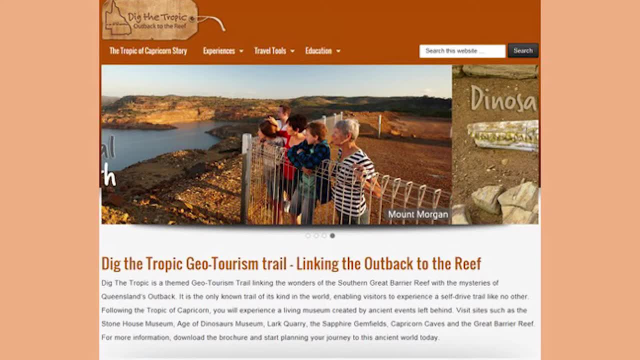 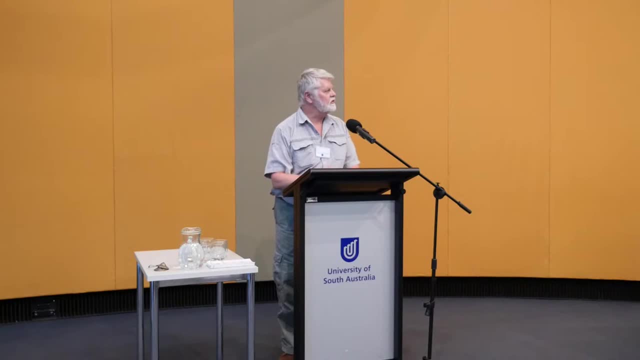 Mount Isa and so on, and it starts at the reef. Big concepts for joining areas with different themes, Not only geological and landscape ones, but the cultural ones associated with them, Slides a bit faint, I'm sorry, but Northwest Tasmania is looking at constructing a range of 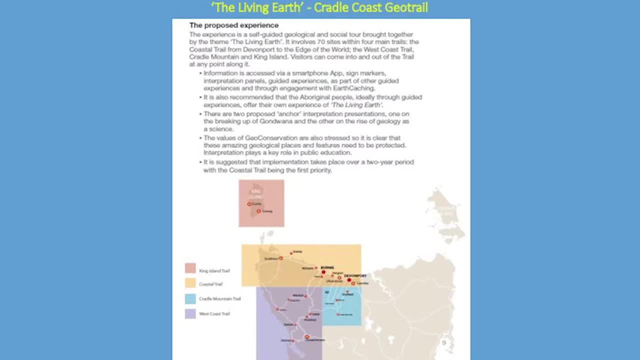 trails that link these things as well. They're geological and natural features, with the cultural overlay Which is one of the themes we've been talking about from all our speakers today. In Canada, there are geotrails all over the place, but they're not coordinated. 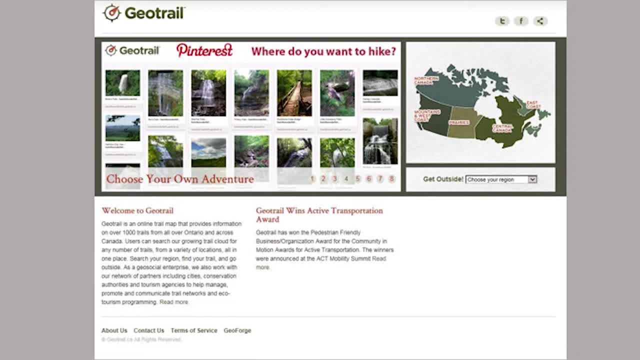 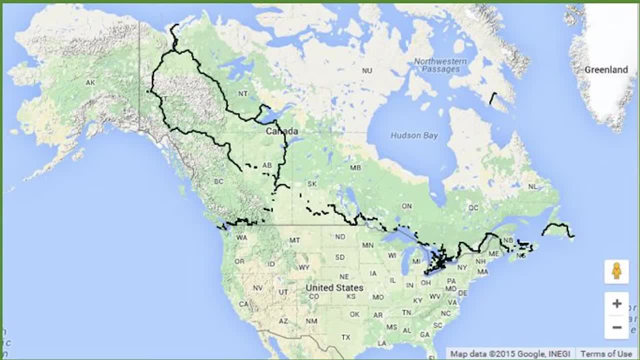 They're done by each province and under local initiatives. And when my next slide comes up, which I calculated should be not here, There we go: The map of the continent of North America, with the Canadian trails cross the continent, And this is one of the visions that those of us in the